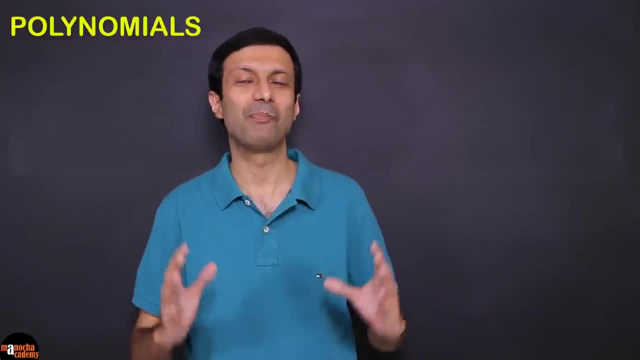 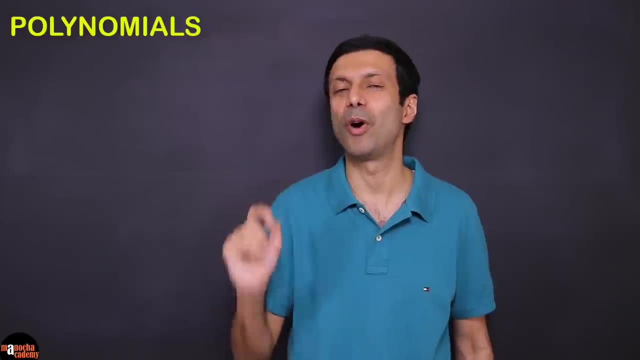 Hi, friends, are you ready to master the topic of polynomials? Then this video is for you, Because in this video we are going to be looking at the key concepts of polynomials and we'll be solving some important questions on this topic. I am going to show you the tips. 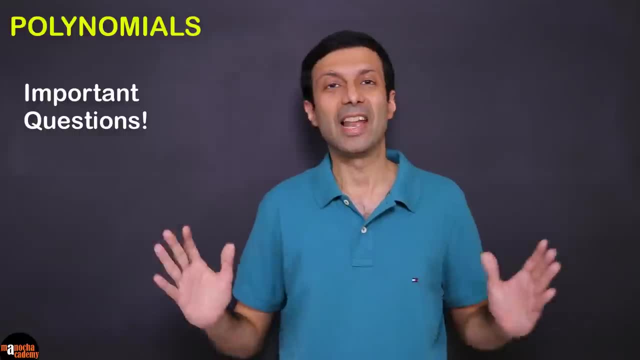 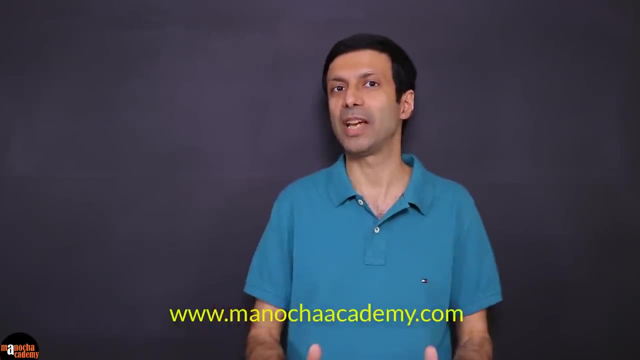 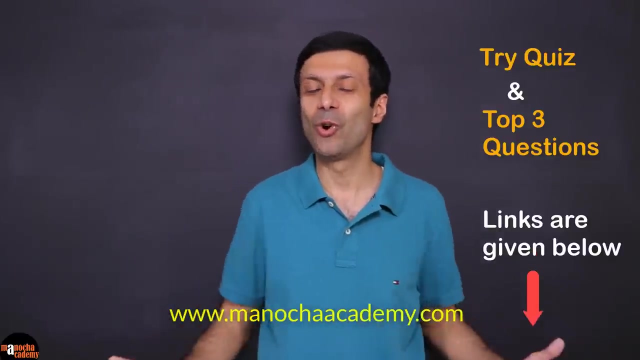 and tricks on how to solve the sums. And if you find this video useful, do hit the like button and share it out with your friends. And do check out my website, manochacademycom, for more questions for you to practice And friends. as you know, practice makes you perfect. 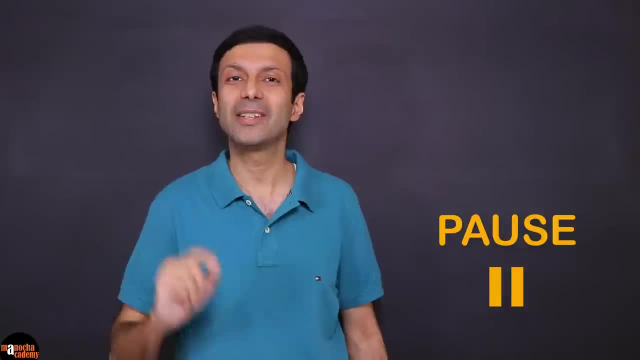 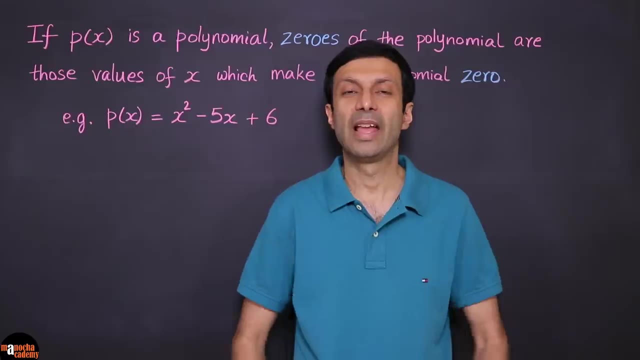 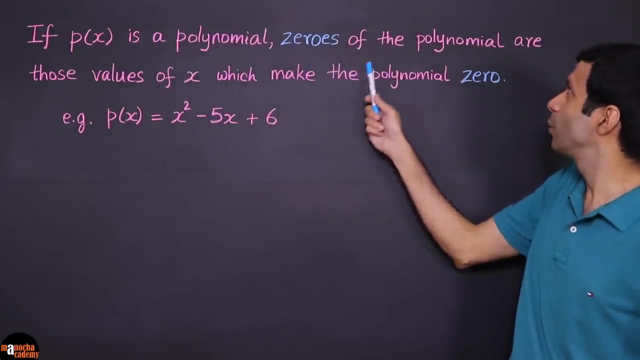 So I want you to pause the video right here and go and get a pen and paper so that we can solve the polynomials topic together. So let's dive right into it. Let's start with the first important concept, which is, if px is a polynomial, zeros of the polynomial are those values of x? okay, 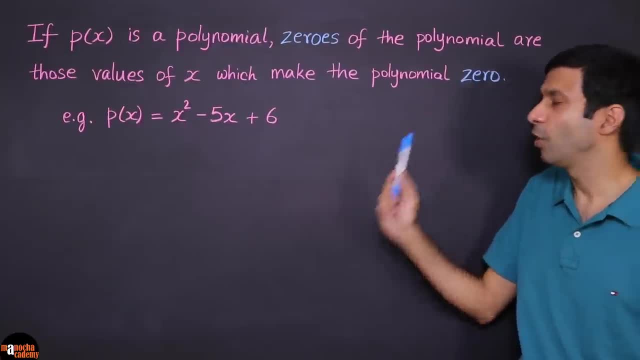 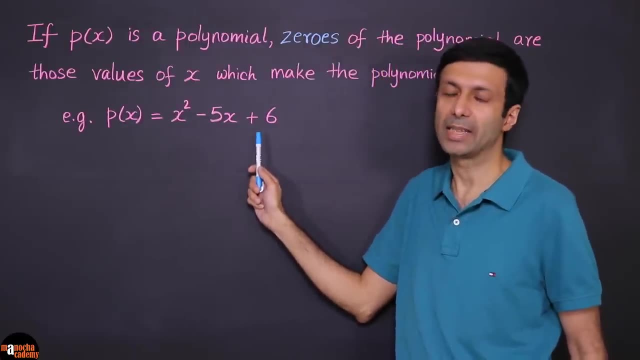 which make up the sum of the polynomials. So let's start with the first important concept, which is, if px is a polynomial, zeros of the polynomial are those values of x, okay- which make up the sum of the polynomials. let's take the polynomial 0.. For example, let's take this polynomial: px equal to x square minus 5x plus 6.. 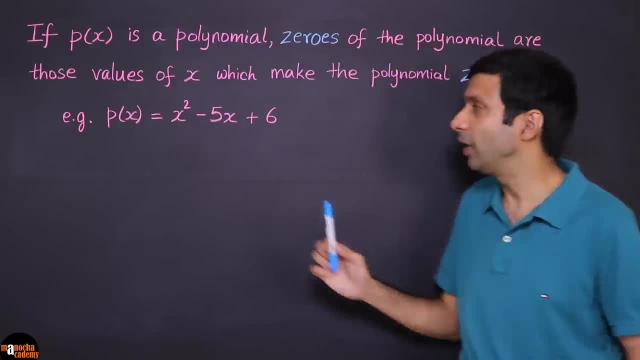 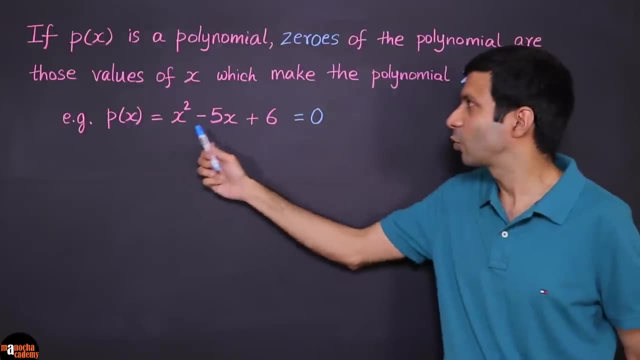 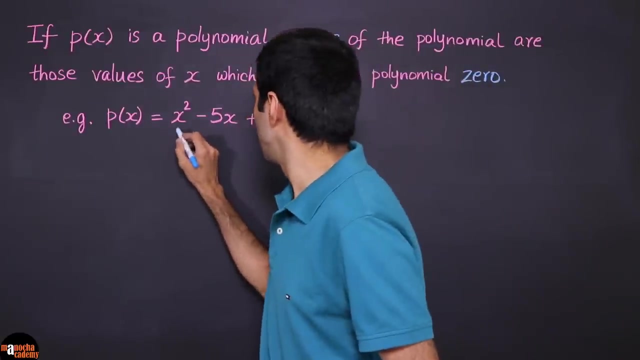 Now to find the zeros of this polynomial, we need to set this polynomial as 0.. So this will be our equation: x square minus 5x plus 6, equal to 0.. Now to solve this equation, we can factorize the left hand side. 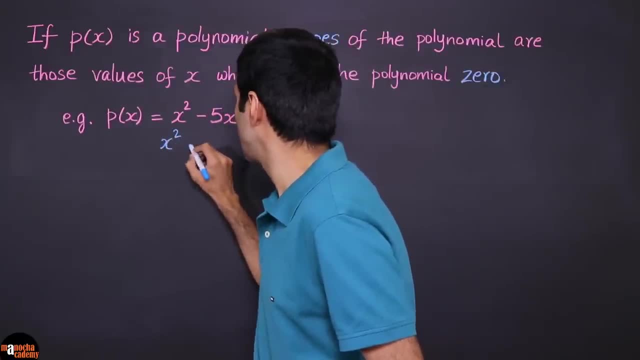 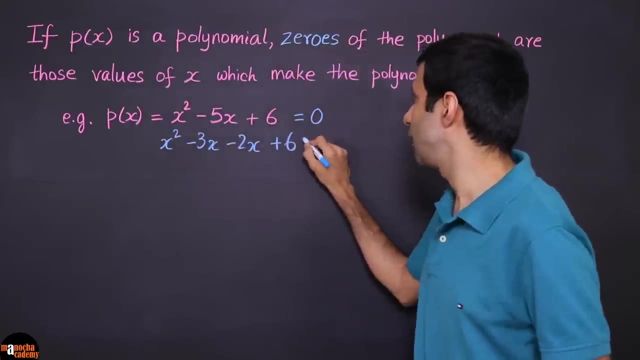 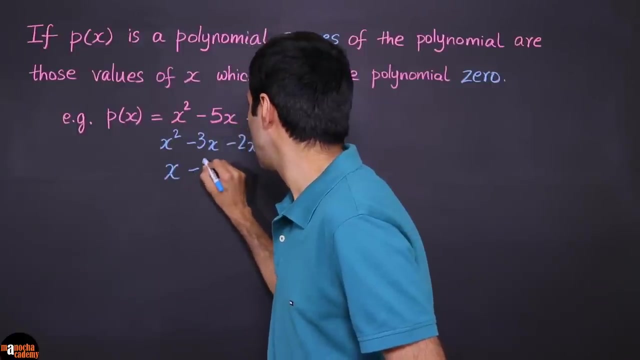 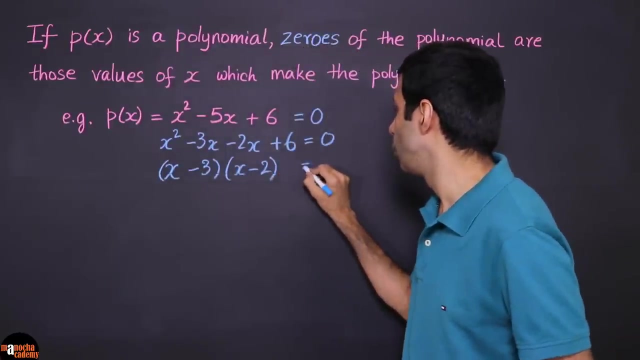 So let's do middle term breaking. So this is going to be x squared minus 3x minus 2x plus 6 equal to 0, right, And now can you see the factors. So if you factorize this, you're going to get x minus 3 multiplied by x minus 2 equals 0.. 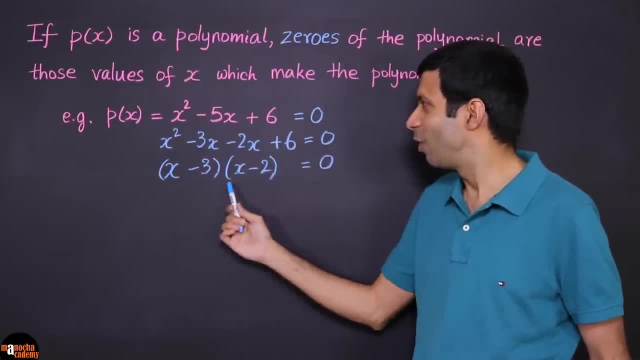 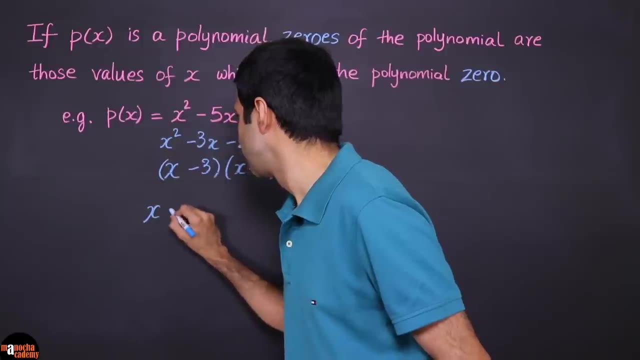 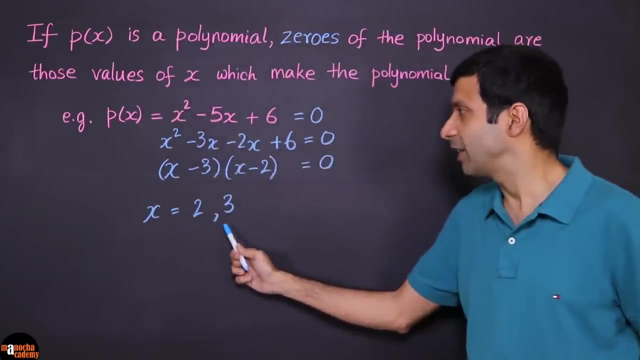 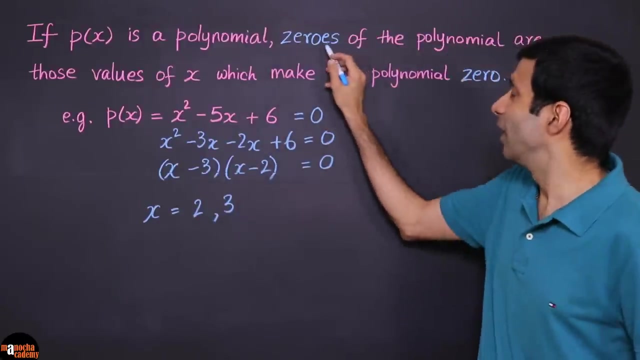 So either x minus 3 is 0 or x minus 2 is 0, right, Which means the values of x are going to be 2 or 3, right. So these values of x are going to make the polynomial 0, right, And these values of x, we said they are called the 0s. 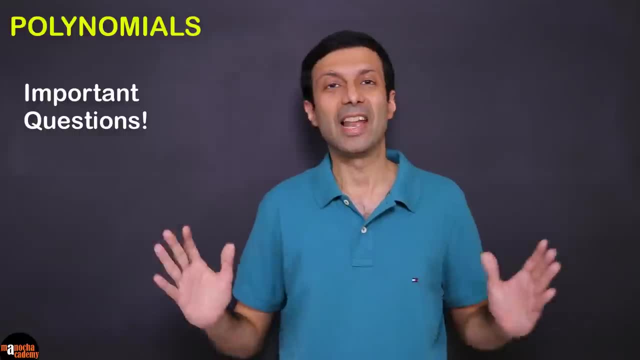 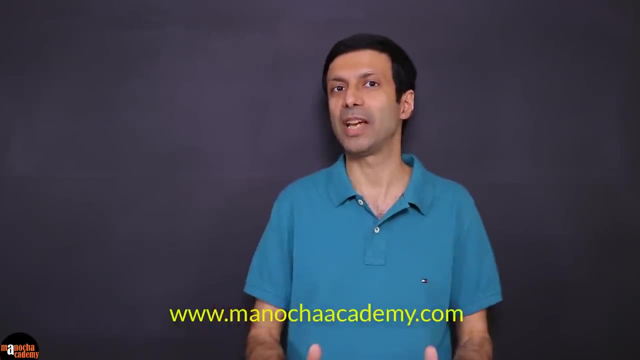 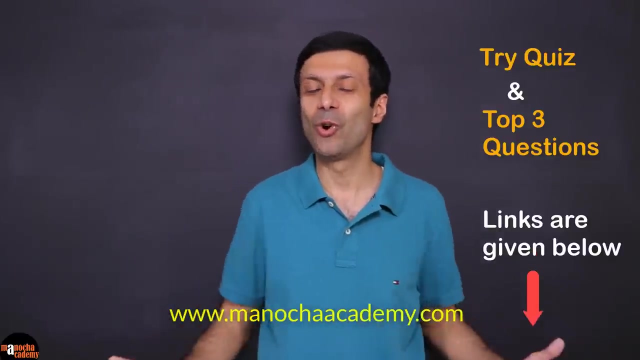 and tricks on how to solve the sums. And if you find this video useful, do hit the like button and share it out with your friends. And do check out my website, manochacademycom, for more questions for you to practice And friends. as you know, practice makes you perfect. 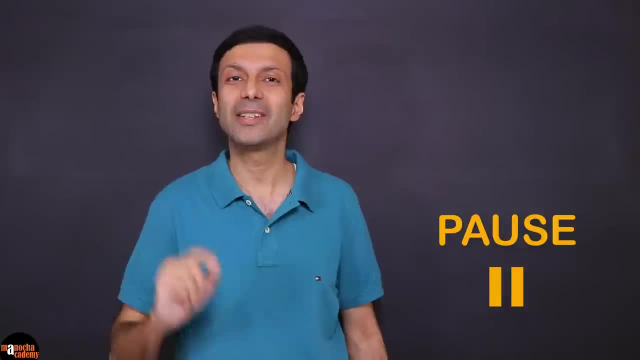 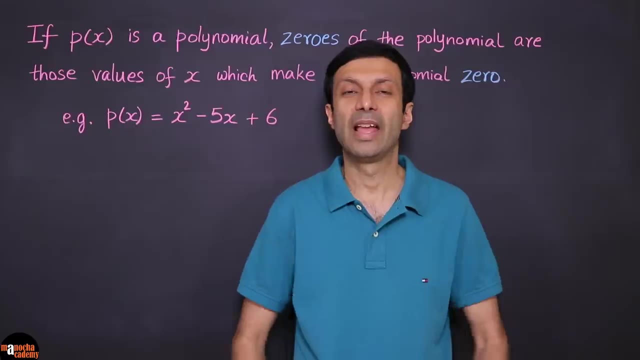 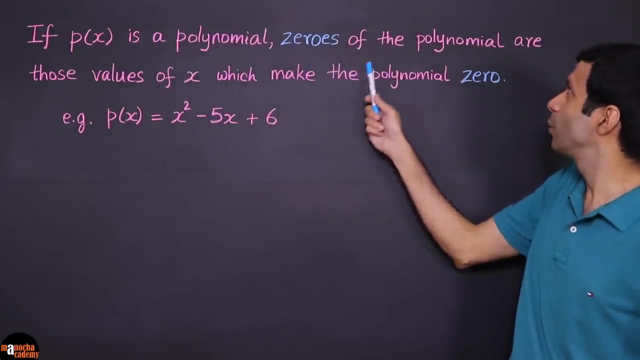 So I want you to pause the video right here and go and get a pen and paper so that we can solve the polynomials topic together. So let's dive right into it. Let's start with the first important concept, which is, if px is a polynomial, zeros of the polynomial are those values of x? okay, which make up the sum of the polynomials. So let's start with the first important concept, which is, if px is a polynomial, zeros of the polynomial are those values of x- okay- which make up the sum of the polynomials. So let's start with the first important concept, which is: if px is a polynomial, zeros of the polynomial are those values of x- okay- which make up the sum of the polynomials. 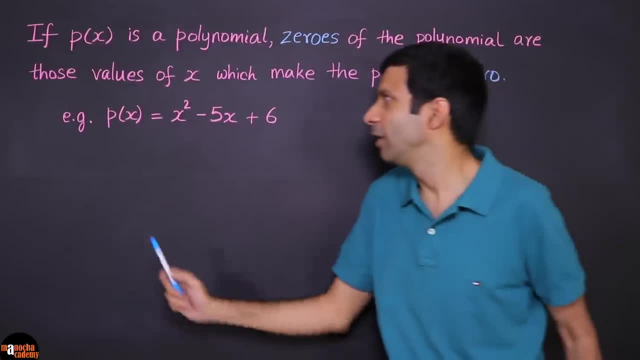 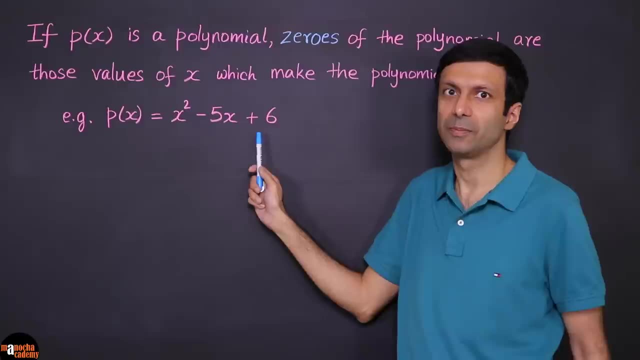 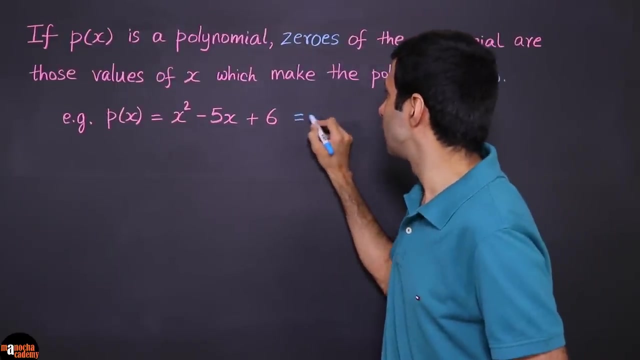 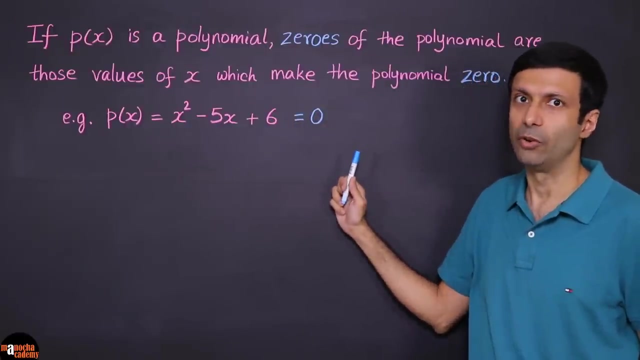 Let's take the polynomial zero, For example. let's take this polynomial: px equal to x squared minus 5x plus 6.. Now to find the zeros of this polynomial, we need to set this polynomial as 0.. So this will be our equation: x squared minus 5x plus 6, equal to 0.. 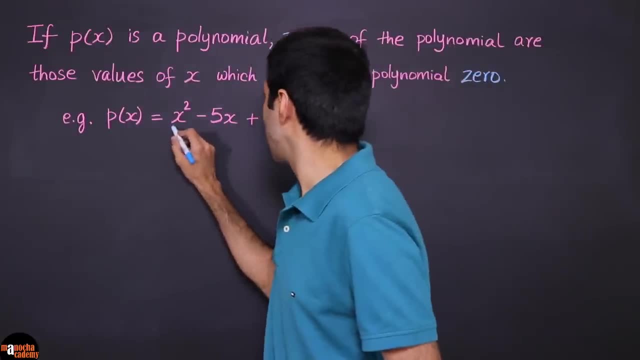 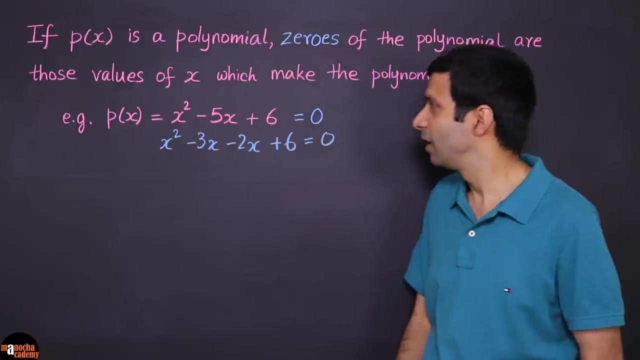 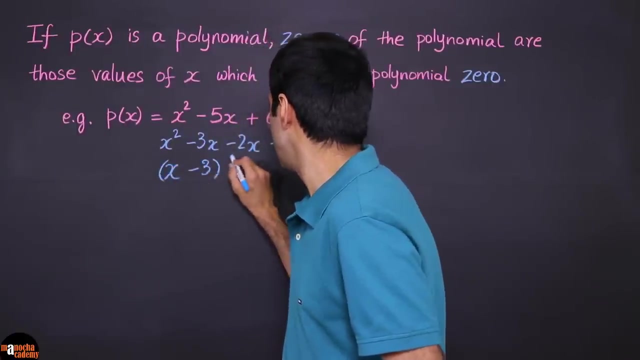 Now to solve this equation, we can factorize the left-hand side, So let's do middle term breaking. So this is going to be x squared minus 3x minus 2x plus 6, equal to 0, right, And now can you see the factors. So if you factorize this, you're going to get x minus 3, multiplied by x minus 2 equals 0.. 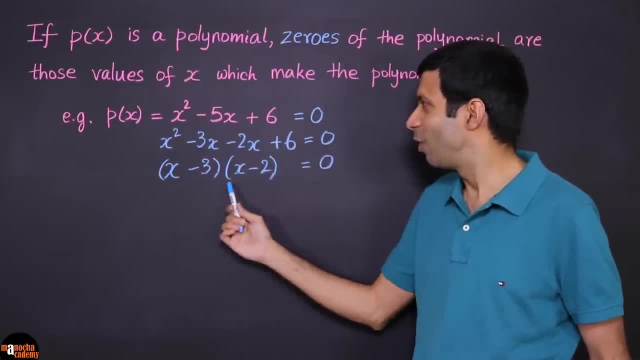 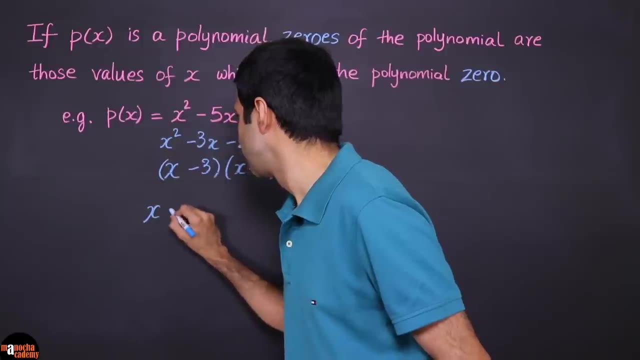 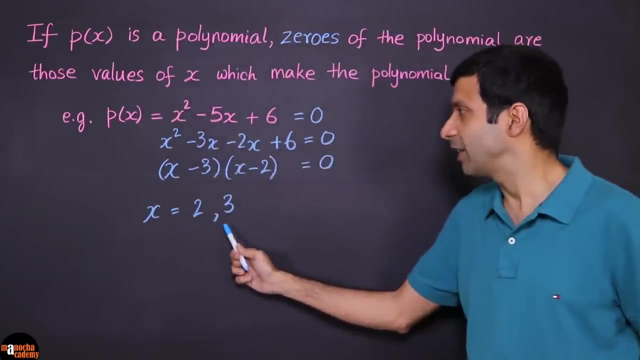 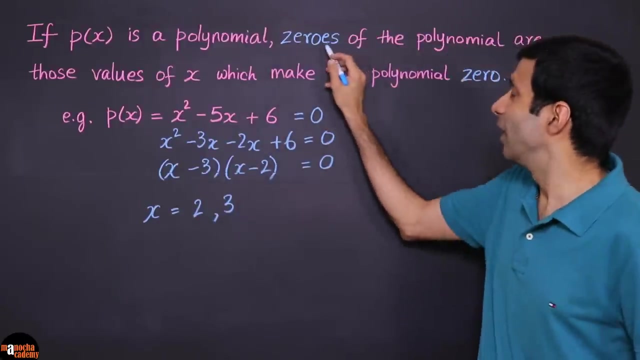 So either x minus 3 is 0 or x minus 2 is 0, right, Which means the values of x are going to be 2 or 3, right. So these values of x are going to make the polynomial 0, right, And these values of x, we said they are called the 0s. 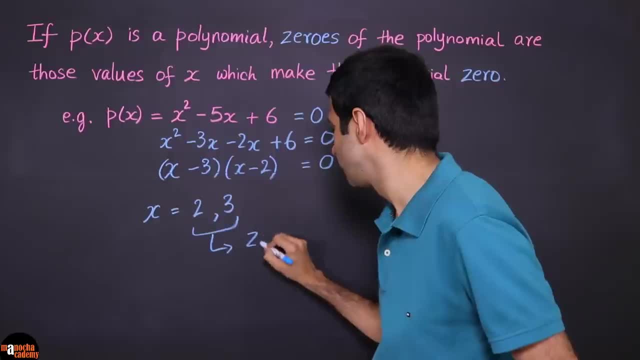 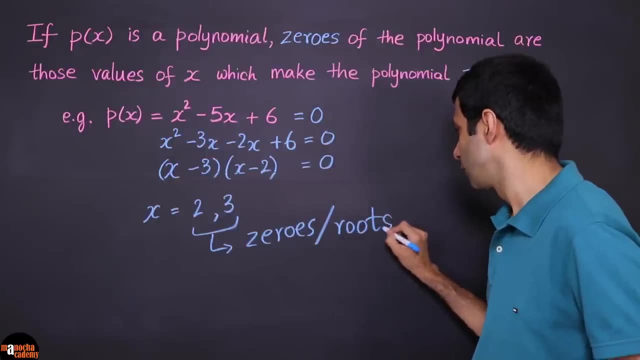 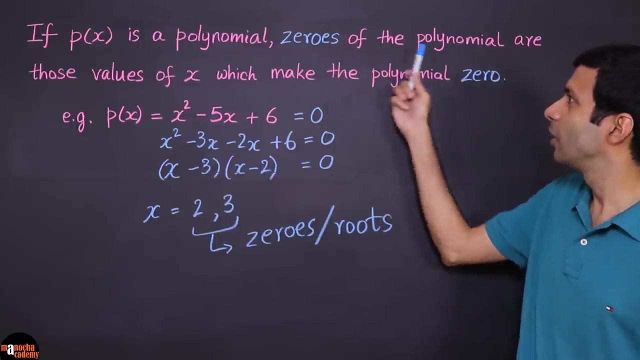 So these values of x are called the 0s, Or they're also known as the roots of the polynomial. So you need to know these two terms. They're either called the 0s or the roots, So it's very simple. So to find the 0s, we need to make the polynomial equal to 0.. 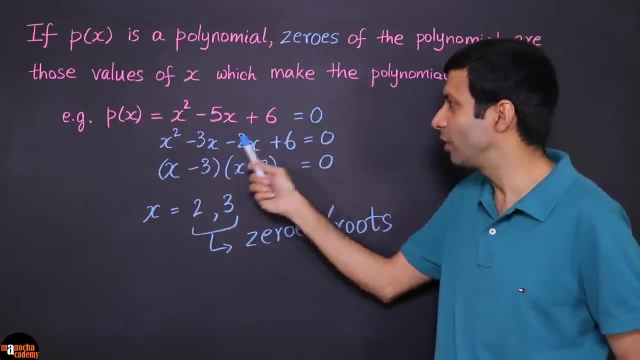 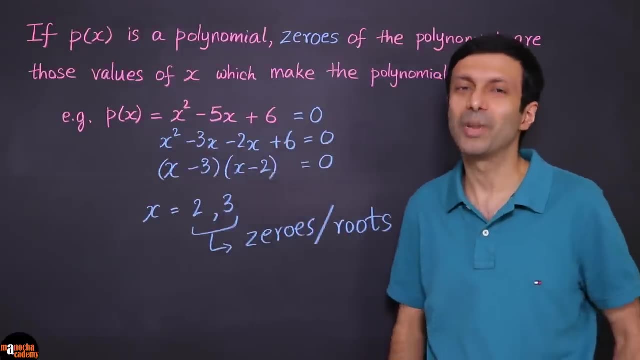 So polynomial px is set equal to 0. That's our equation, And the solution of that gives us the 0s, or the roots, which is those values of x. that makes the polynomial 0.. Now let's look at the next concept. 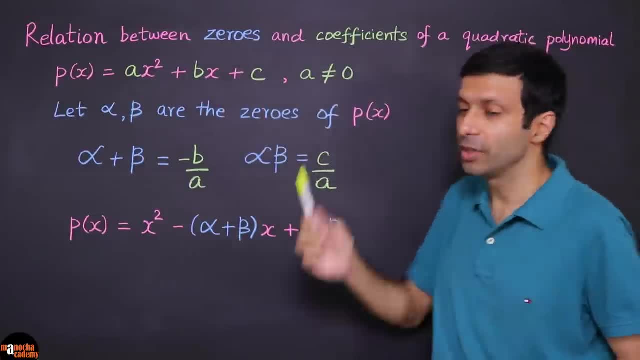 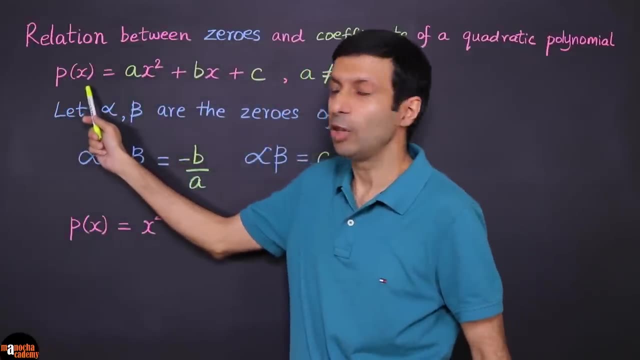 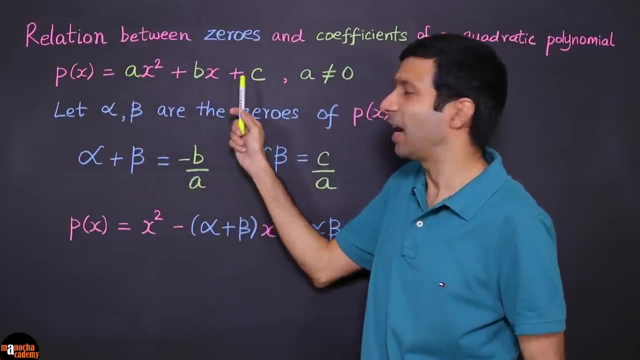 The relation between 0s and coefficients of a quadratic polynomial. So let's say our quadratic polynomial px equals ax squared plus bx plus c, where the coefficients are a, b and c right And the coefficient a is not equal to 0. Why? 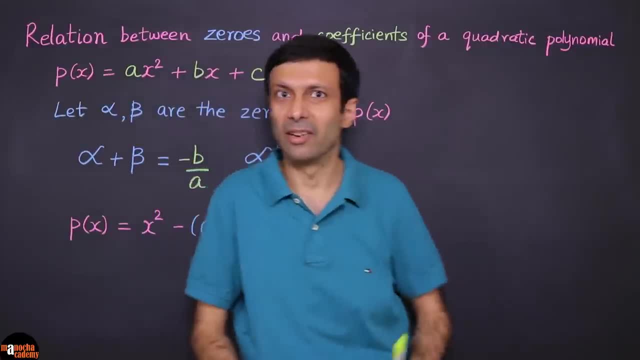 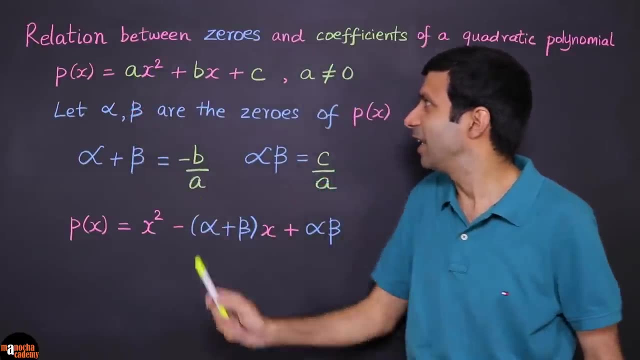 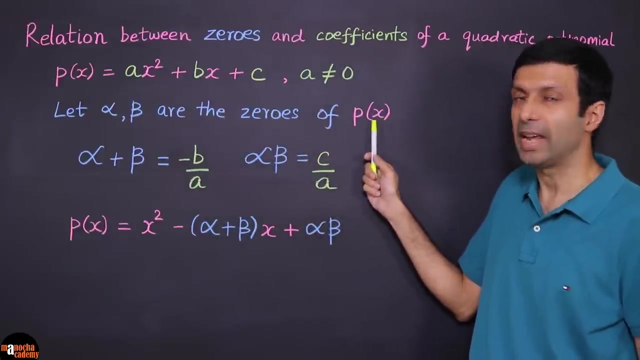 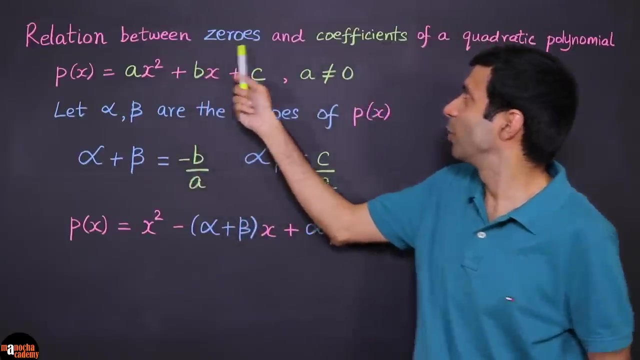 Because we want a quadratic polynomial, So we want that term x squared in there. So a should not be 0. And let's say that alpha and beta are the 0s, or the roots, of the quadratic polynomial px. Then there's this important relation between the roots and the coefficients. 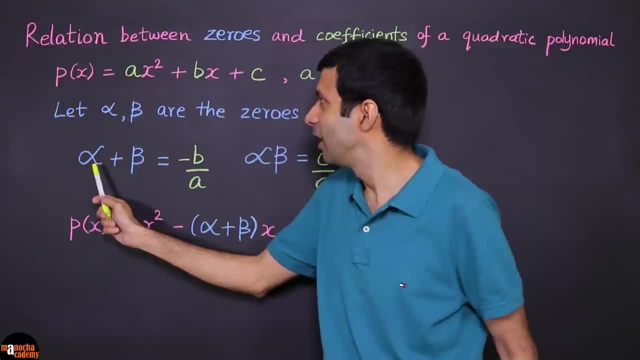 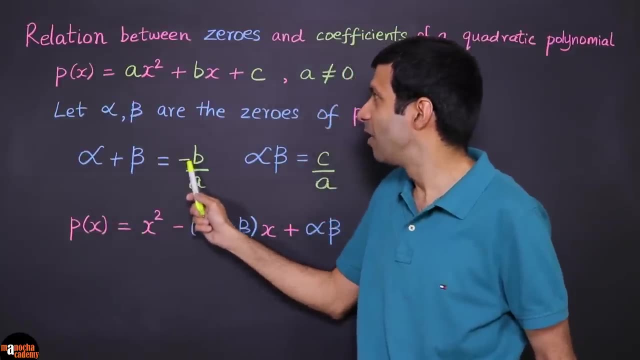 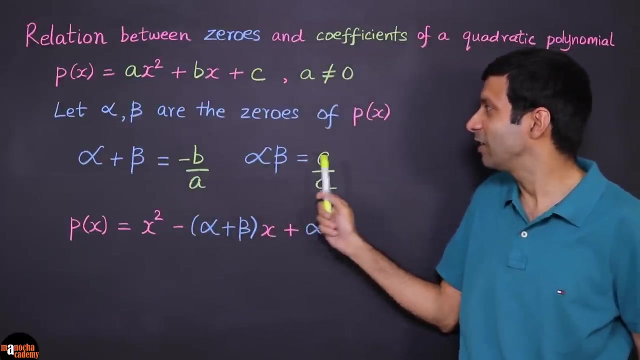 So between the 0s and the coefficients, And what is it? That? alpha plus beta is equal to minus b by a. So the sum of the roots is minus b by a. These coefficients And the product of the 0s is alpha. beta is equal to c by a. 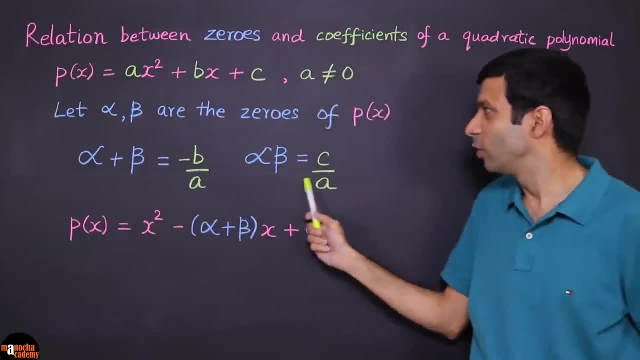 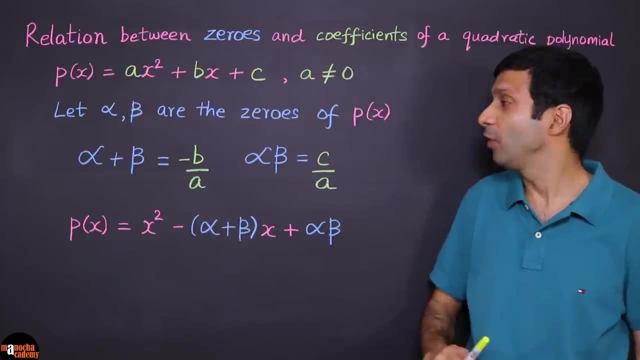 So these coefficients, So note these two important relations between the 0s and the coefficients of the quadratic polynomial. And if we know the 0s of the polynomial alpha beta, then we can write the quadratic polynomial as x squared minus b by a. 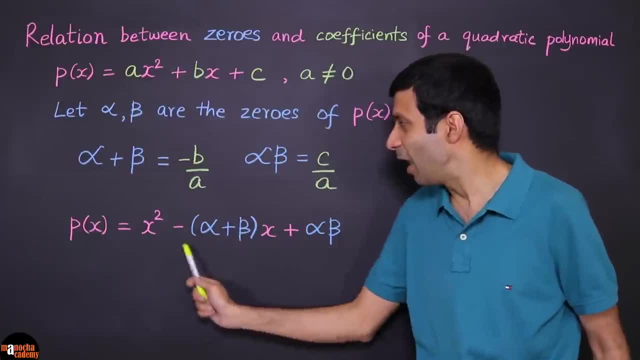 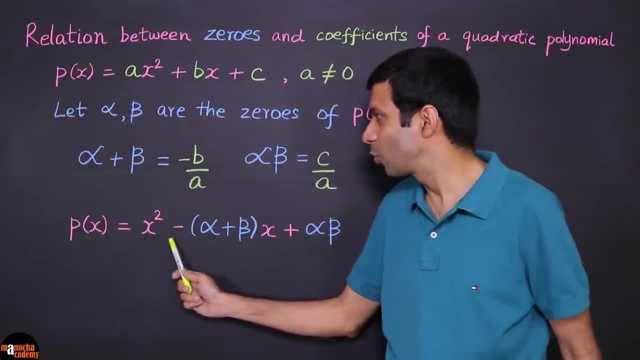 So that's our equation. So the sum of the roots is minus b by a. So the sum of the roots is minus alpha plus beta into x plus alpha beta, Right. So basically it's x squared minus sum of the roots times x plus the product of the roots. 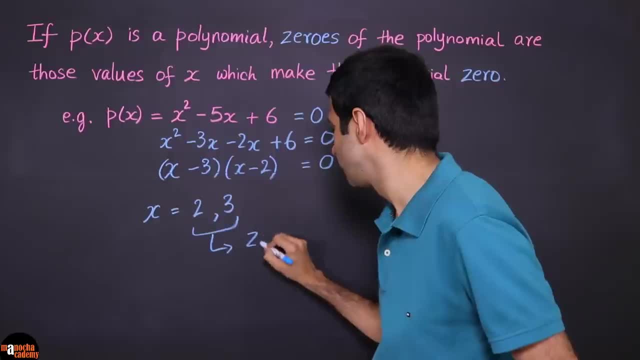 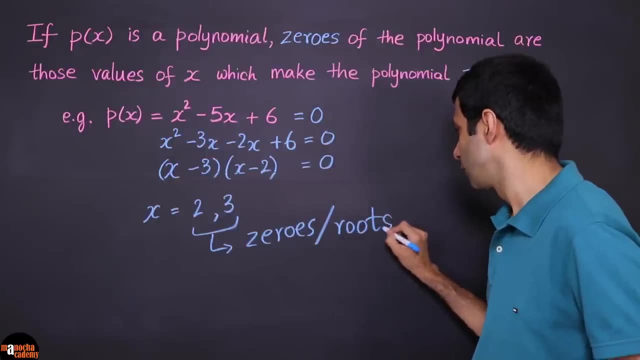 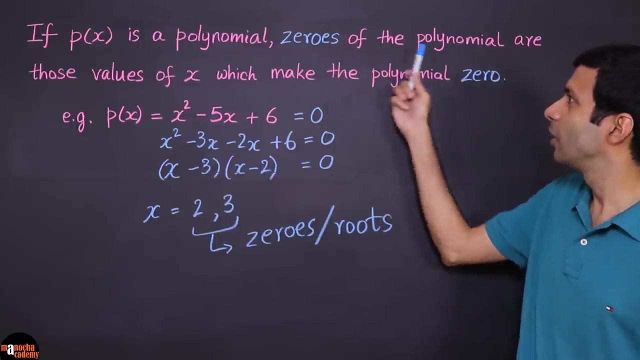 So these values of x are called the 0s, Or they're also known as the roots of the polynomial. So you need to know these two terms. They're either called the 0s or the roots, So it's very simple. So to find the 0s, we need to make the polynomial equal to 0.. 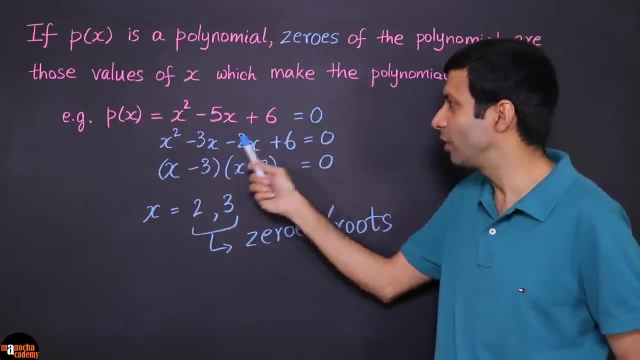 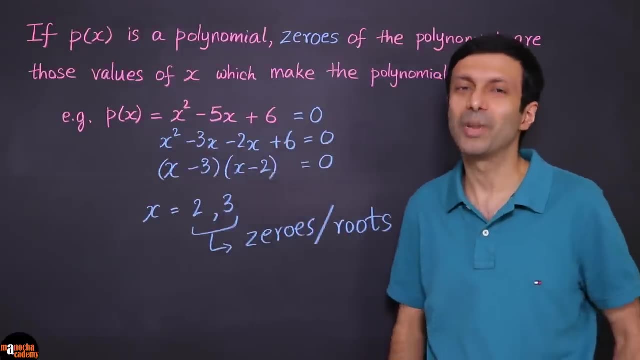 So polynomial px is set equal to 0. That's our equation, And the solution of that gives us the 0s, or the roots, which is those values of x. that makes the polynomial 0.. Now let's look at the next concept. 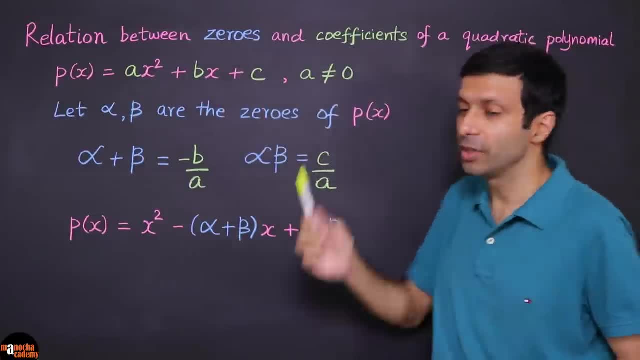 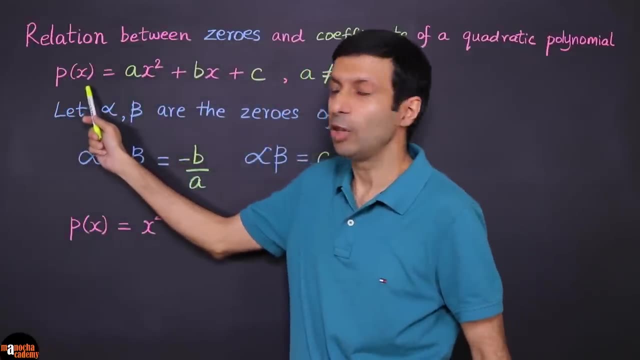 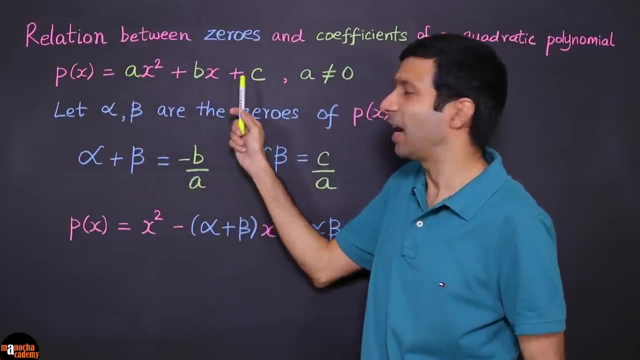 The relation between 0s and coefficients of a quadratic polynomial. So let's say our quadratic polynomial px equals ax squared plus bx plus c, where the coefficients are a, b and c right And the coefficient a is not equal to 0. Why? 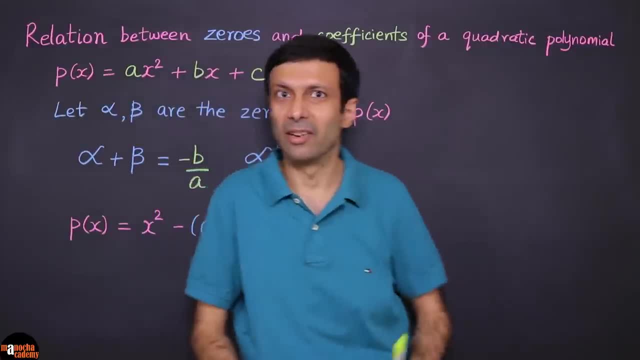 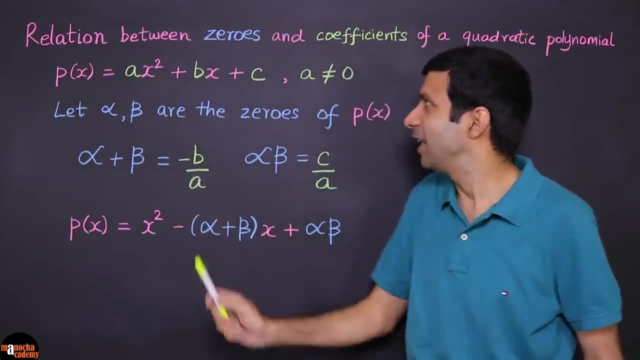 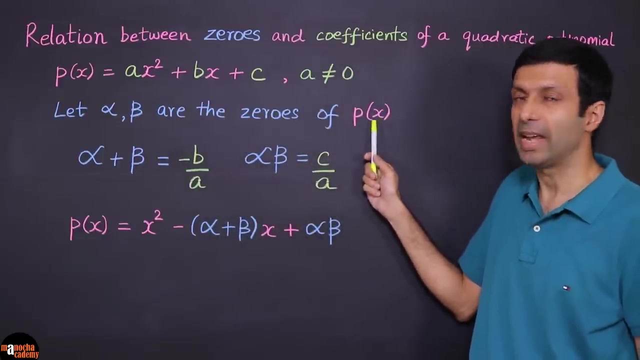 Because we want a quadratic polynomial Right, So we want that term x squared in there. So a should not be zero. Ok, And let's say that alpha and beta are the 0s, or the roots of the quadratic polynomial px. Then there is this important relation between the roots and the coefficients. 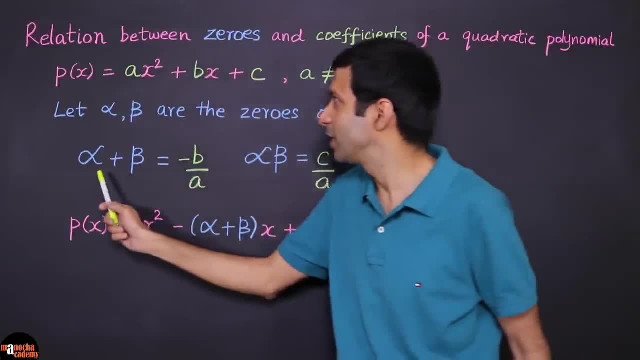 So with the 0s and the coefficients, and what is it? That alpha plus beta is equal to minus b by a. So whenever all of these 0s are the coefficients, Right? So then there's also that equation As I talked about earlier. with this equation, etcetera, 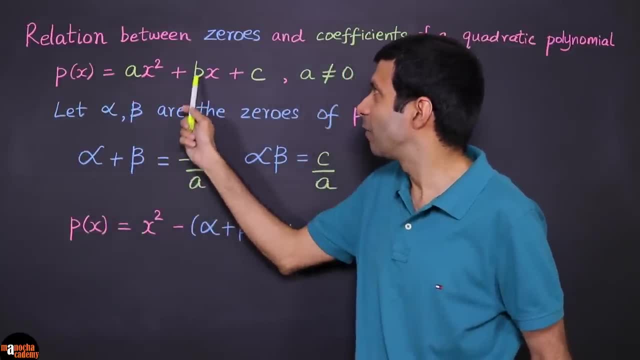 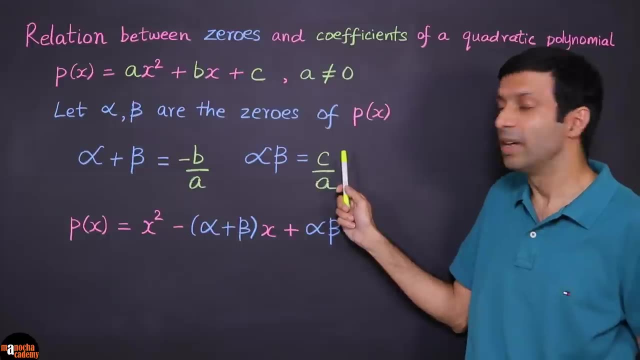 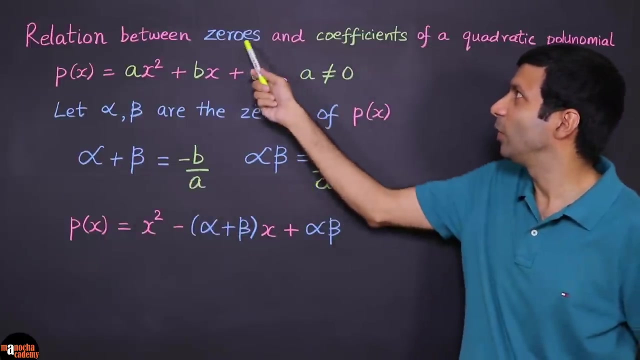 Samshu, growth without plus beta is equal to minus b by a, So the sum of the roots is minus b by a. these coefficients And the product of the zeros is alpha. beta is equal to c by a, So these coefficients. So note these two important relations between the zeros and the coefficients of the quadratic polynomial. 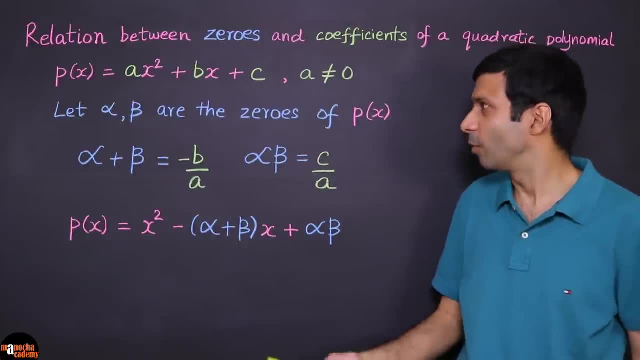 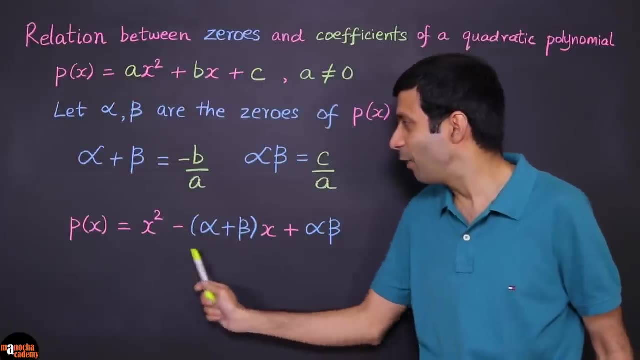 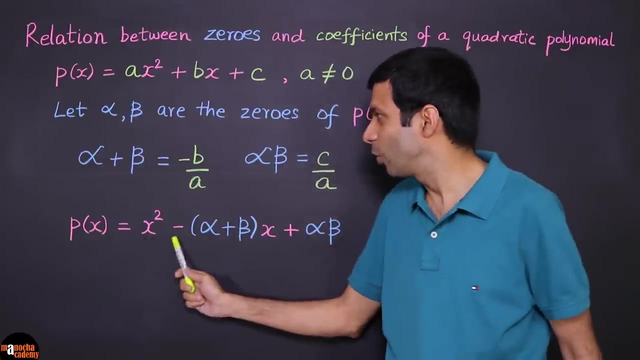 And if we know the zeros of the polynomial alpha beta, then we can write the quadratic polynomial as x square minus alpha plus beta into x plus alpha beta, right? So basically it's x square minus sum of the roots times x plus the product of the roots. 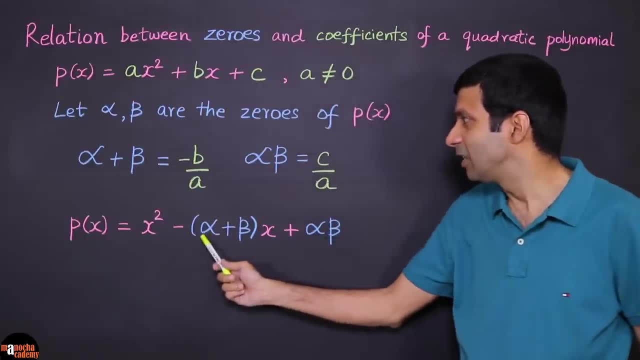 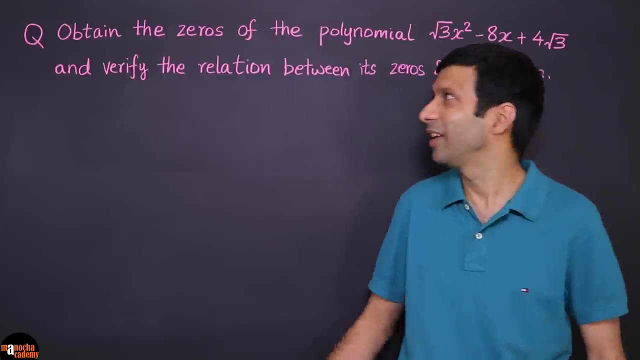 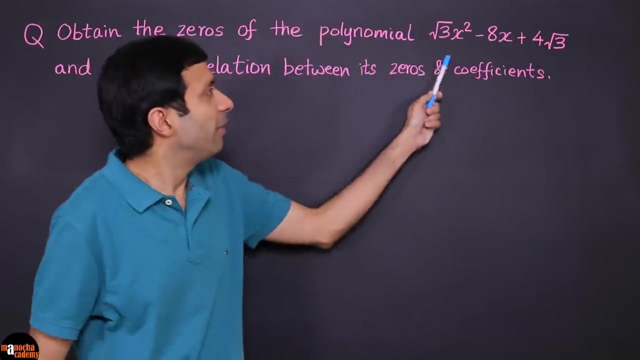 So we can write the quadratic polynomial in terms of the 0s here. So note this important formulae. Now let's take a look at this question. Obtain the 0s of the polynomial Root 3, x squared minus 8x, plus 4 root 3.. 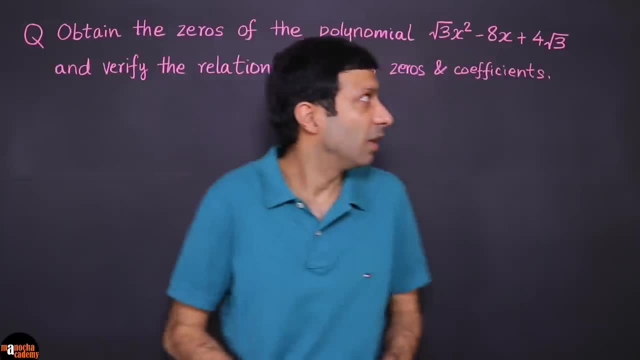 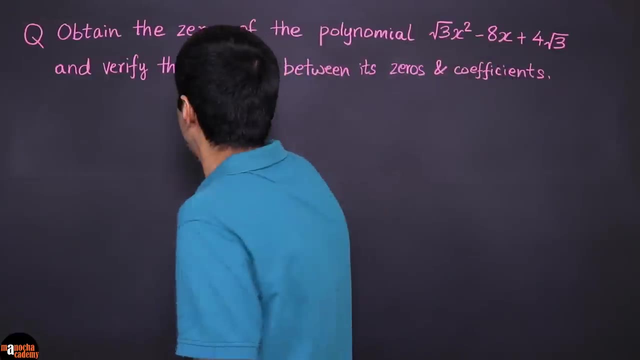 And verify the relation between its 0s and coefficients. Okay, So remember, we are going to copy down that polynomial And to find the 0s, we need to set it to 0.. So it's root 3 x squared. 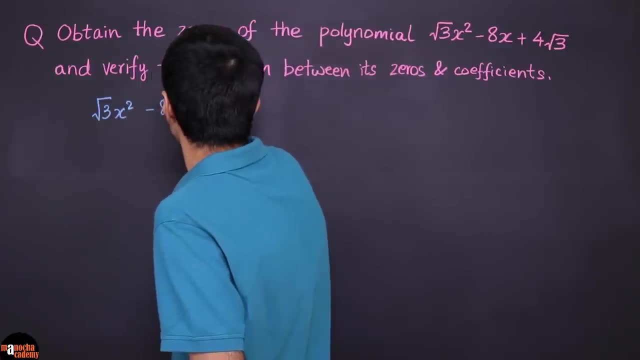 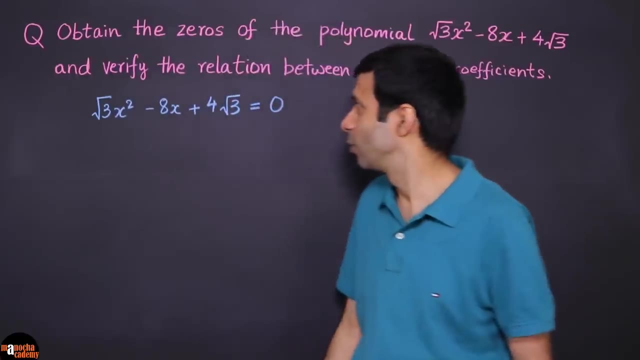 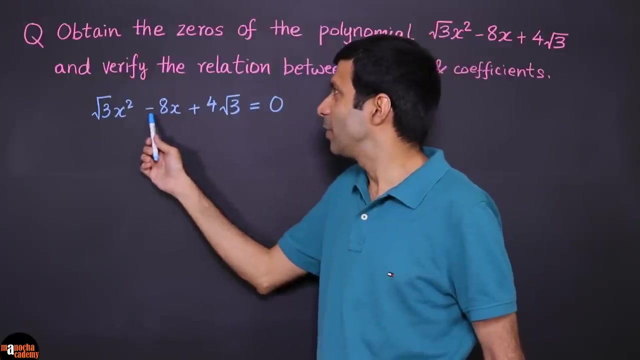 Right, Minus 8x Plus 4 root 3. And we'll set it equal to 0.. Okay, And now we can use middle term breaking to factorize this polynomial, So can you see that the sum is going to be minus 8.. 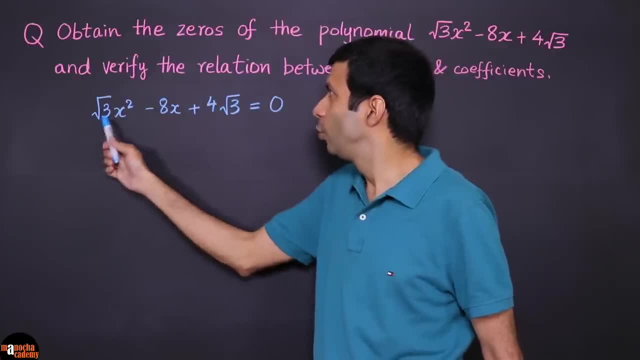 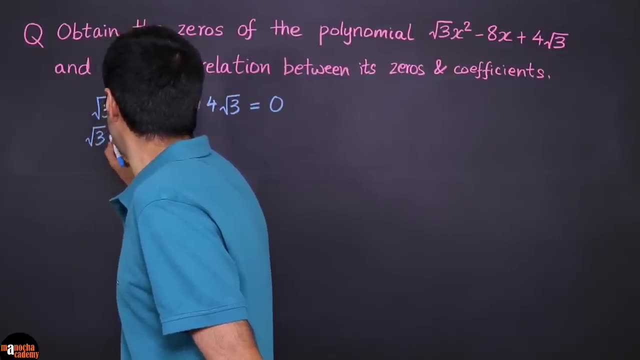 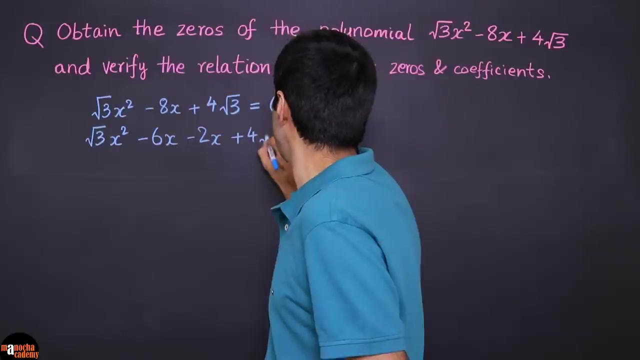 And the product is going to be 4 root 3 into root 3.. So that's 12.. So let's break the middle term like this: Root 3 x squared minus 6x minus 2x Plus 4 root 3.. 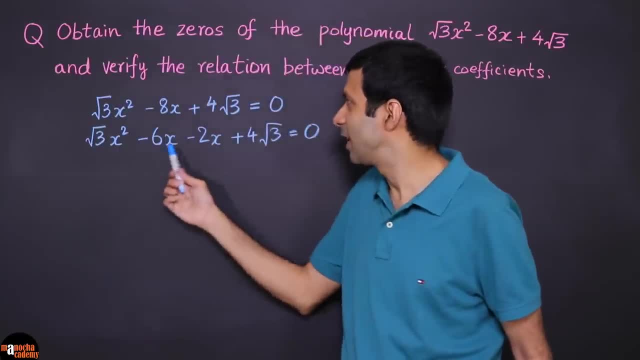 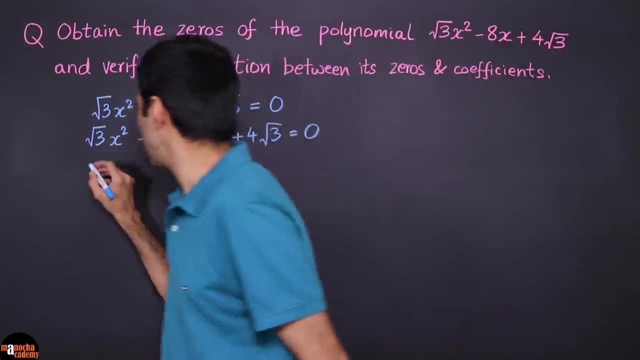 Equals 0. So can you see that the sum is minus 8.. And the product 6 into 2, is 12.. Okay, So now let's factorize this, So it's going to be root 3 x. 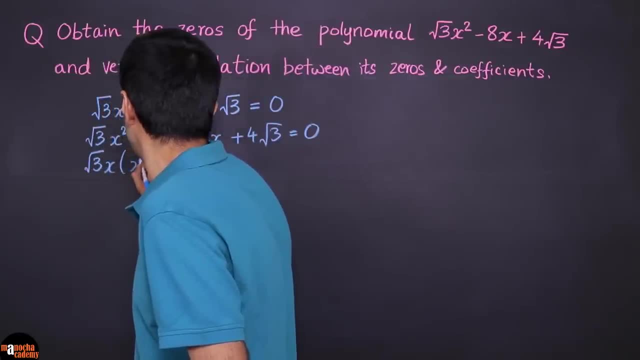 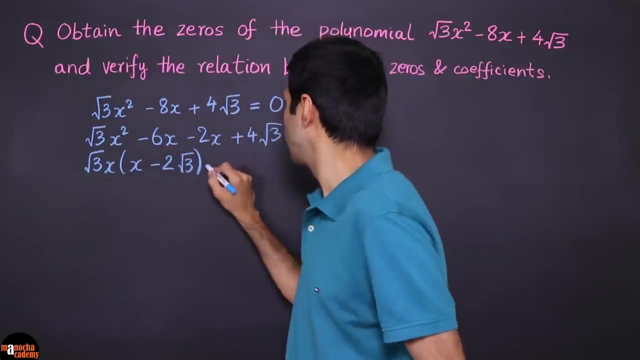 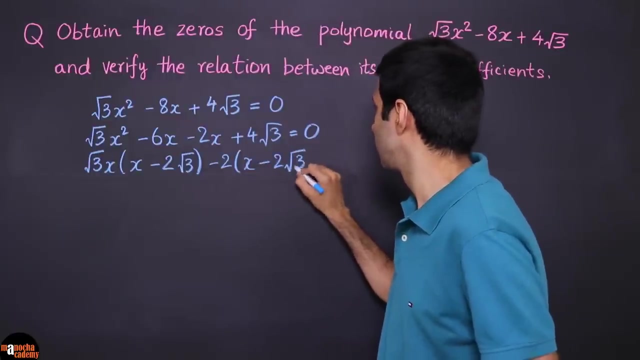 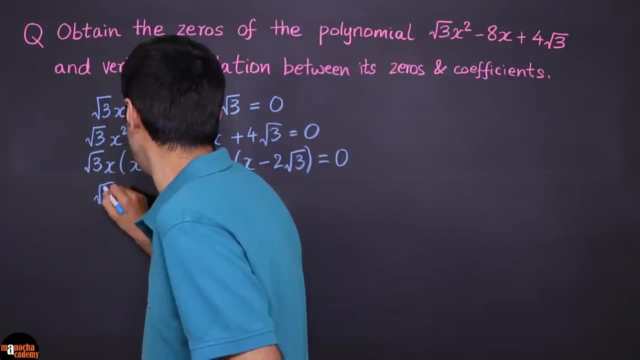 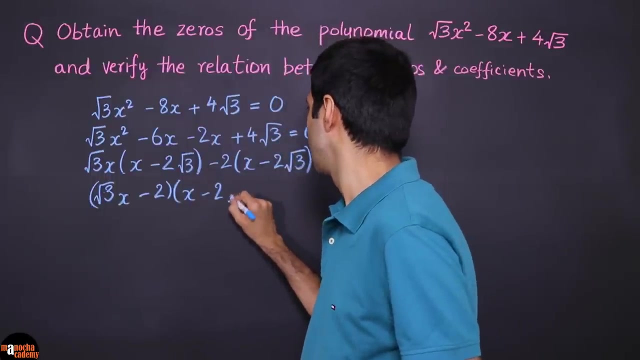 And this is going to be x minus 2 root 3.. And here we'll have a minus 2.. So x minus 2 root 3, again Right Equal to 0.. So if we group these, we're going to get the factors as root 3, x minus 2, into x minus 2. root 3 equals 0. 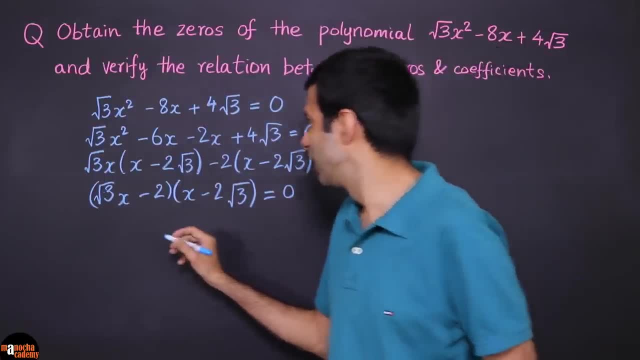 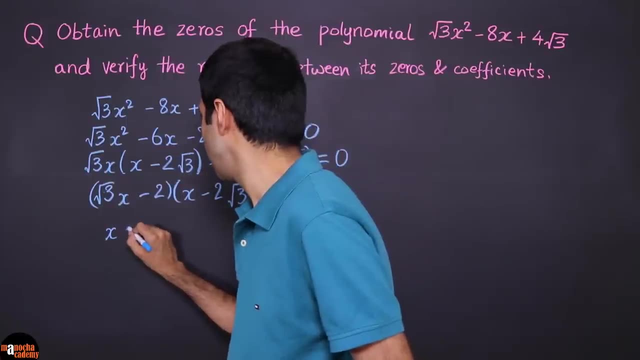 Okay, So what are the roots here? Or what are the 0s? So x is going to be. so either this is 0 or this is 0. And so we have x equals 2 by root 3 from this one. 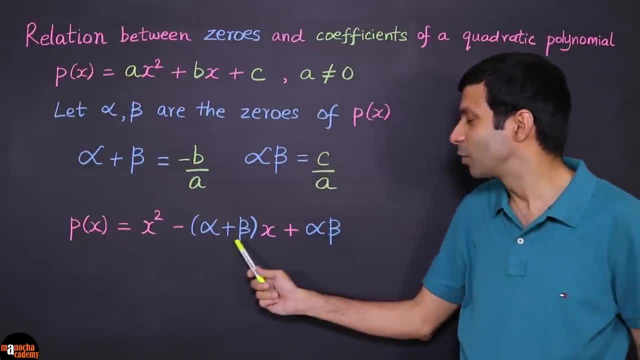 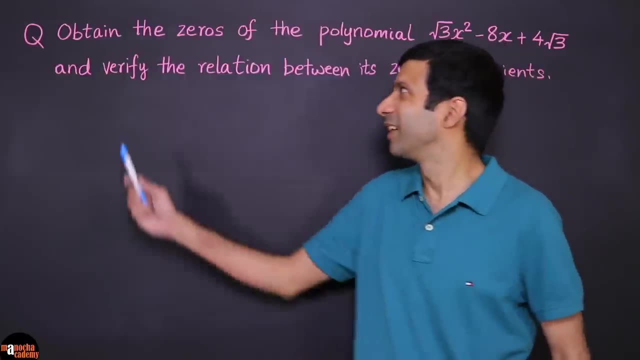 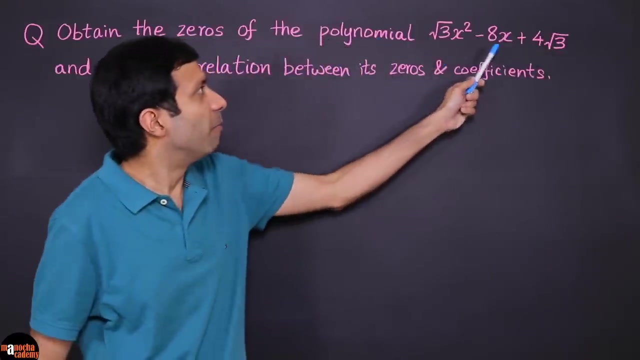 So we can write the quadratic polynomial in terms of the zeros here. So note this Important formulae. Now let's take a look at this question. Obtain the zeros of the polynomial root 3, x square minus 8x plus 4, root 3.. 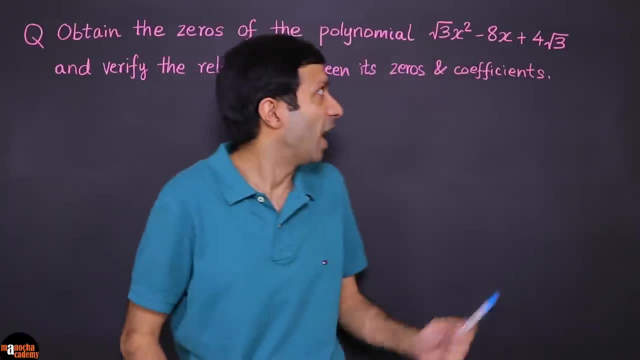 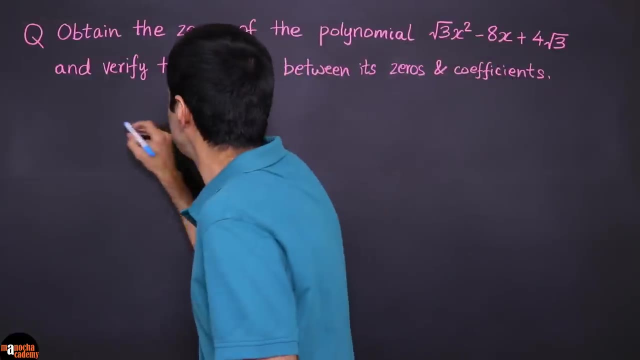 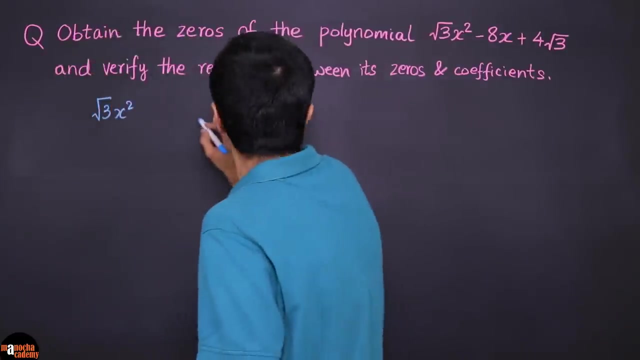 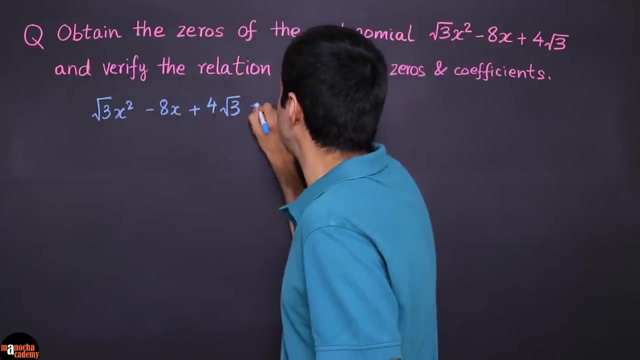 And verify the relation between its zeros and coefficients. Okay, So remember, we are going to copy down that polynomial And to find the zeros, we need to set it to zero. So it's root 3 x square Right, Minus 8x plus 4, root 3, and we'll set it equal to zero. 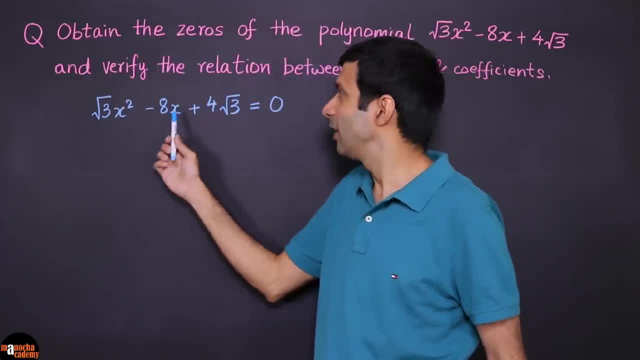 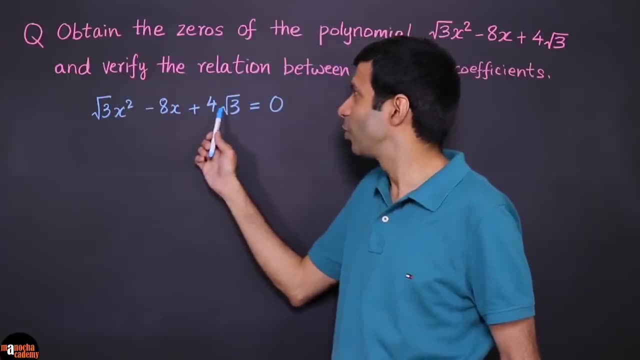 Okay, And now we can use middle term breaking to factorize this polynomial. So can you see that the sum is going to be minus 8 and the product is going to be 4 root 3 into root 3.. So that's 12.. 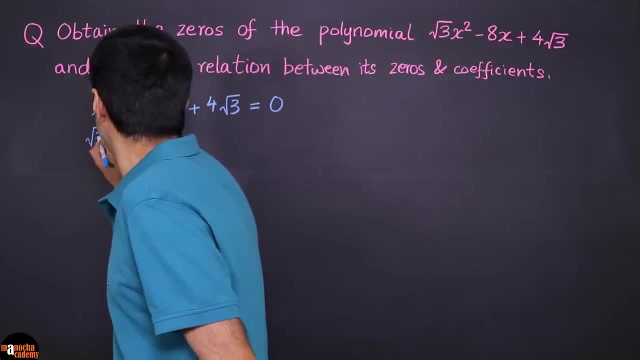 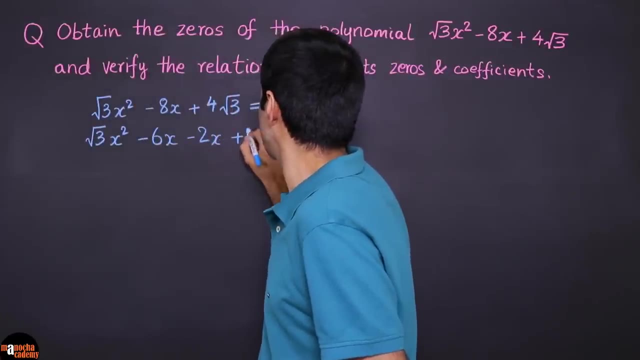 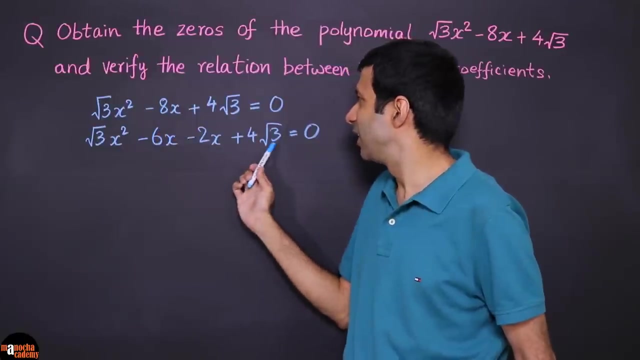 So let's break the middle term like this: Root 3 into root 3.. So it's going to be x square minus 6x minus 2x plus 4, root 3 equals zero. So can you see that the sum is minus 8 and the product 6 into 2, is 12.. 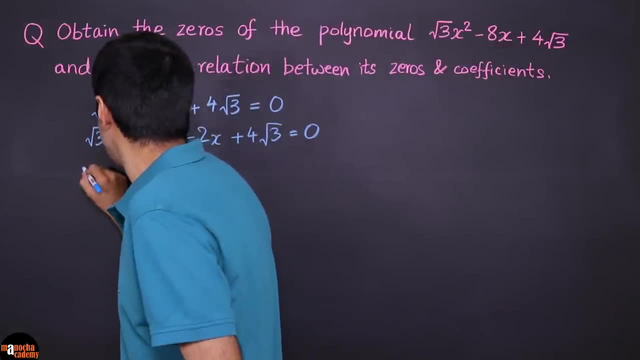 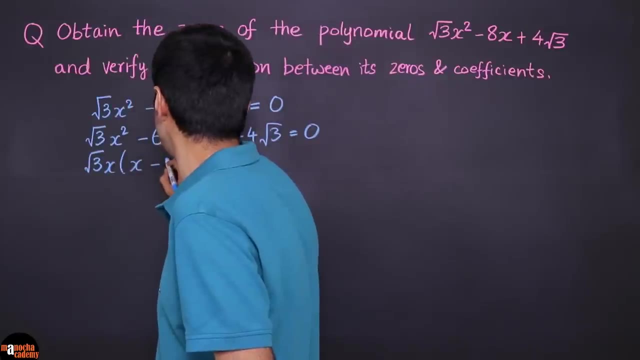 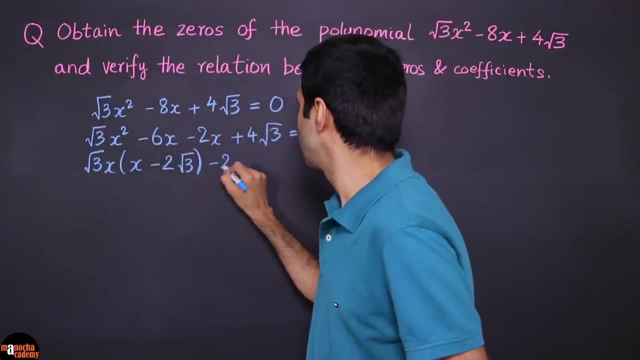 Okay, So now let's factorize this. So it's going to be root 3, x, And this is going to be x minus Okay, 2 root 3.. And here we'll have a minus 2.. So x minus 2 root 3 again. 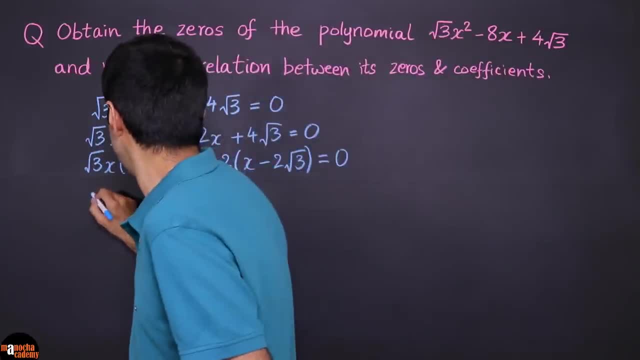 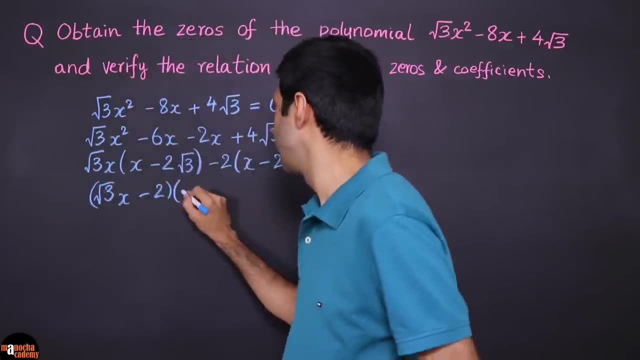 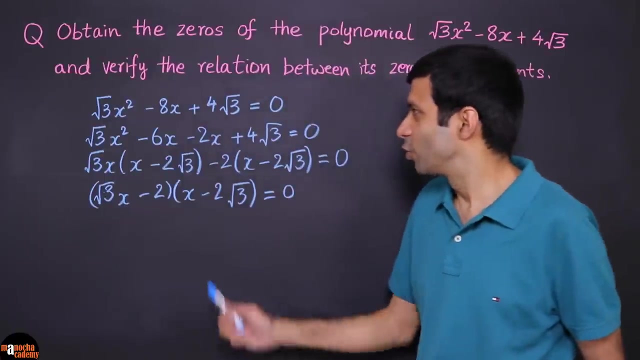 Equal to zero. So if we group these, we're going to get the factors as root 3, x minus 2, into x minus 2. root 3 equals zero. Okay, So what are the roots here, Or what are the zeros? 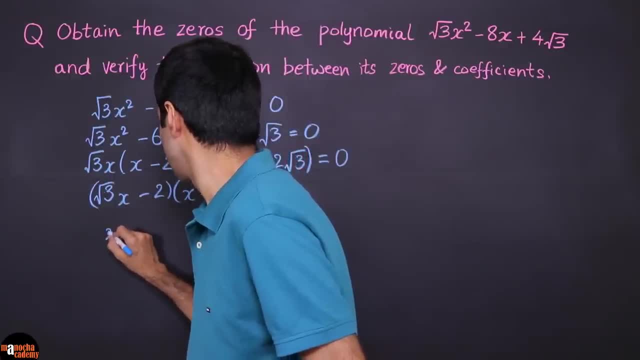 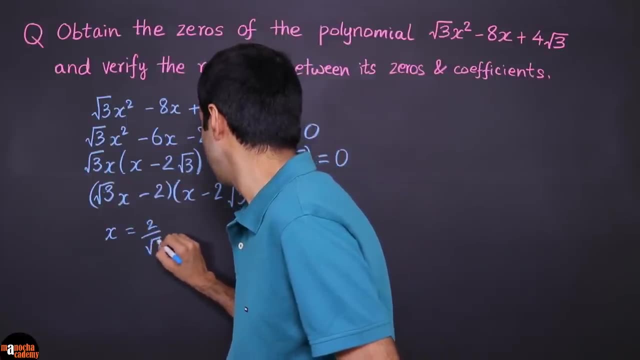 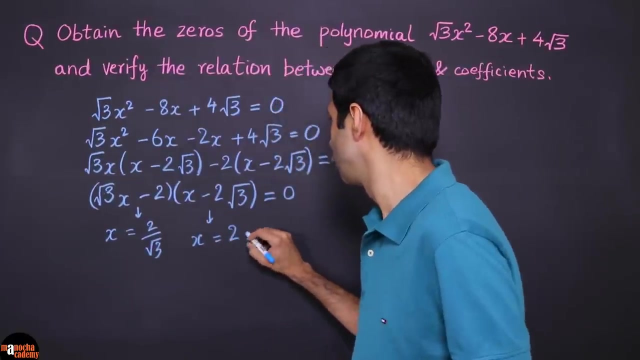 So x is going to be. So either this is zero or this is zero, And so we have x equals 2 by root 3. from this one, Right, And from this one also, we'll get x equal to 2 root 3.. 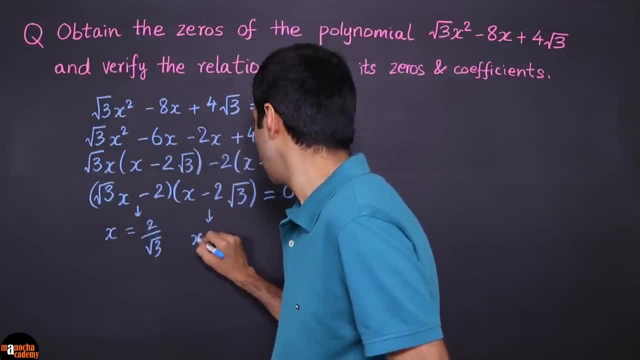 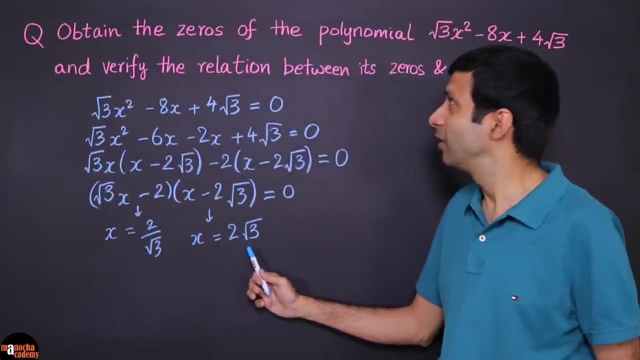 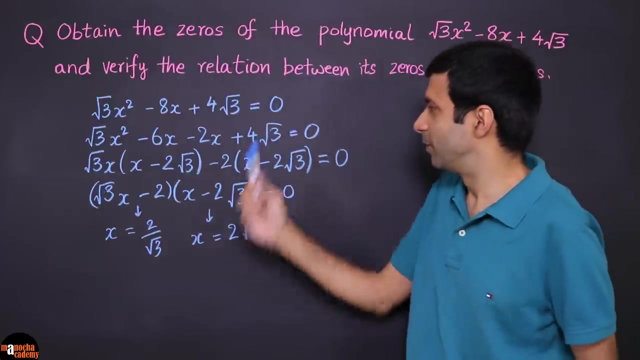 Right, And from this one also, we'll get x equal to 2 root 3.. Right, So these are the 0s of the polynomial of our quadratic polynomial, Right, So we found the 0s here. This is our answer. 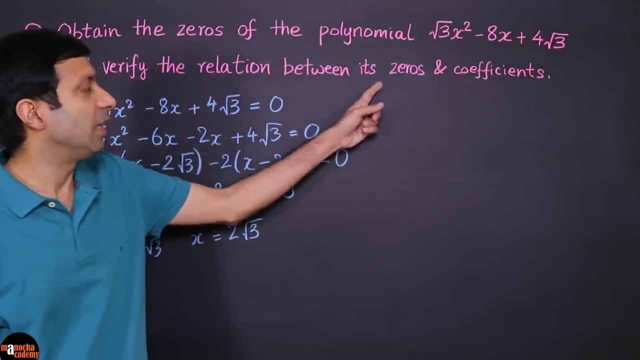 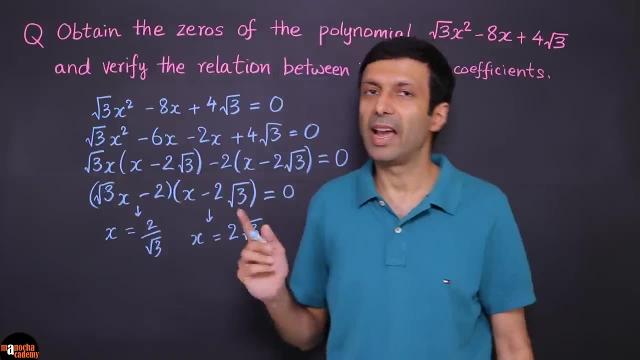 And now we need to verify the relation between the 0s and the coefficients. So remember the formula that we learned: Alpha plus beta equals minus b by a, And alpha beta equals c by a. So let's apply that. So what is our formula here? 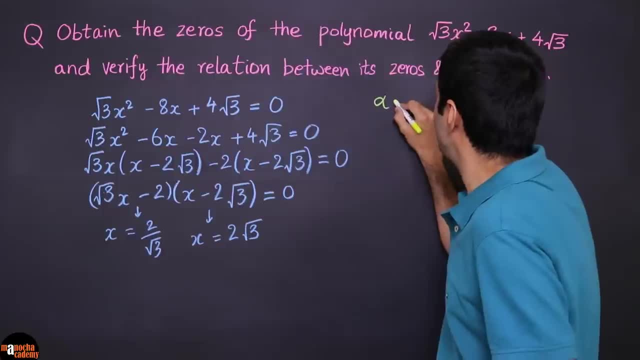 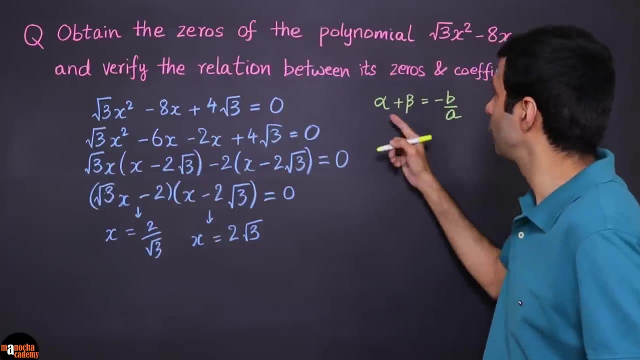 So let's write that down: Alpha plus beta equals minus b by a, Right? So that's going to be minus b by a. So what is the coefficient? So we are going to compare this with. remember what is the standard form of the polynomial. 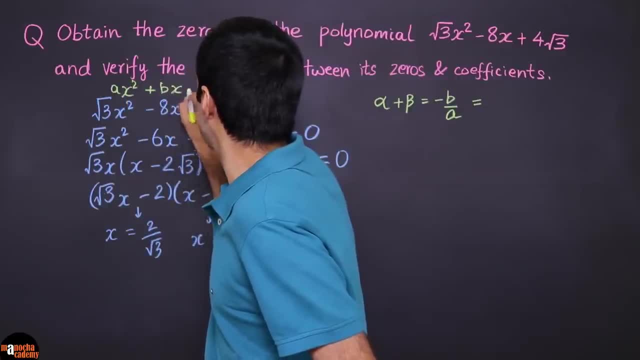 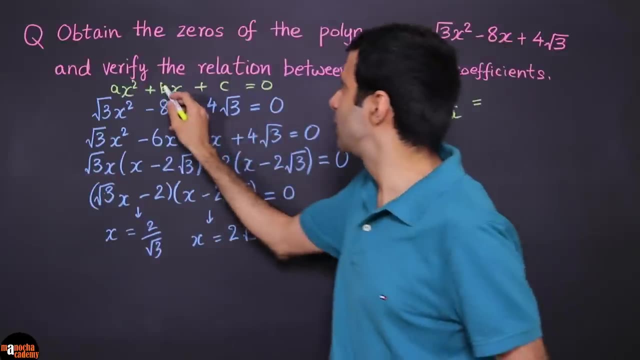 quadratic polynomial Ax squared plus bx plus c, Right, And that we had set equal to 0.. So here b is 8,, sorry, minus 8, and a is root 3.. Right, So this is going to be minus of. 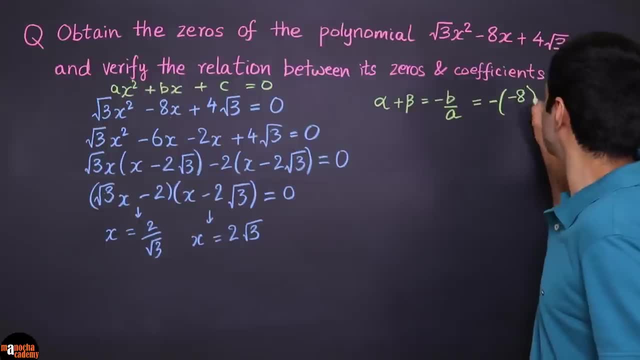 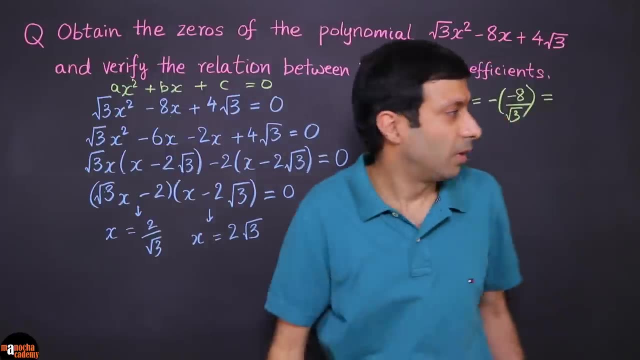 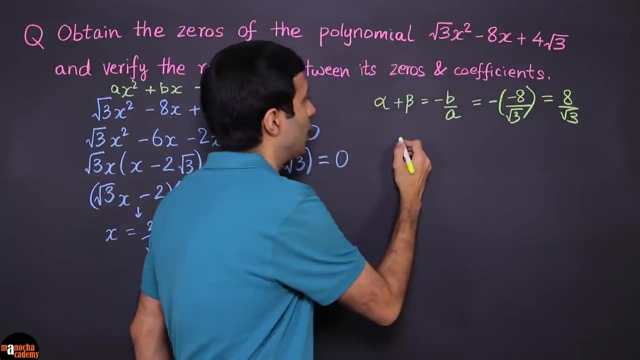 We have b as minus 8 here, And a is root 3.. So what is the sum of the 0s going to be? It's going to be 8 by root 3.. Okay, And now let's do the product of the roots. 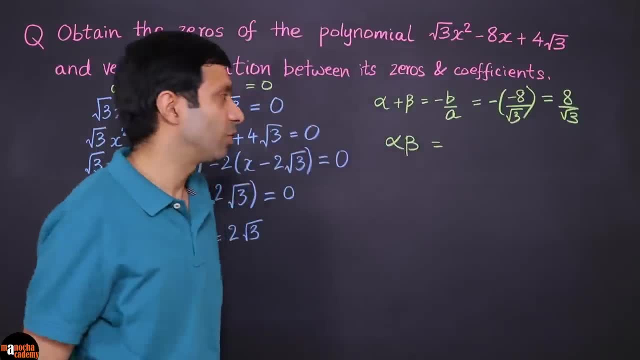 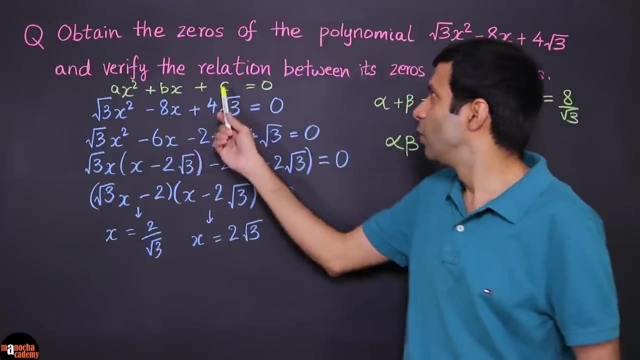 Alpha, beta. the product of the 0s, or the roots, is going to be c by a. That's our formula Right. So again, we need to use our coefficients c and a. So what is the coefficient c? It's basically 4 root 3.. 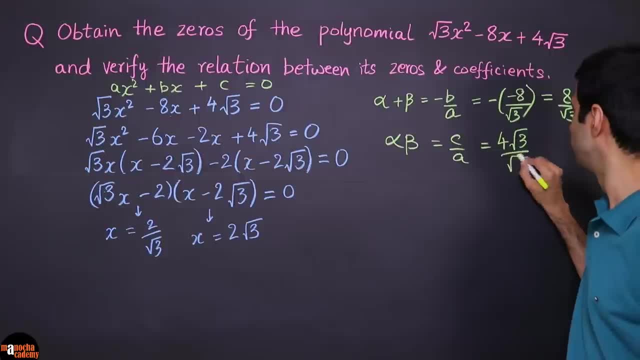 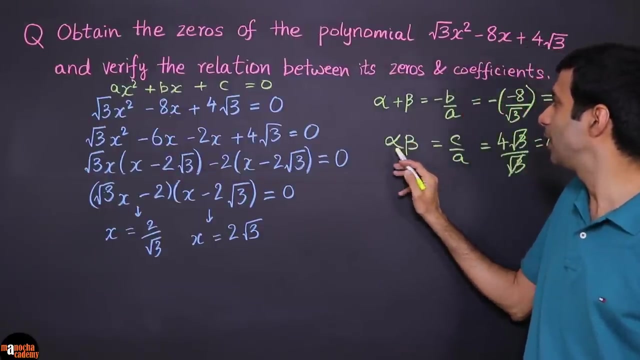 Right And a is root 3.. So root 3 cancels and the product of the 0s is 4.. Okay, And so to verify this relation, because we have used this relation right: Alpha plus beta and alpha beta. 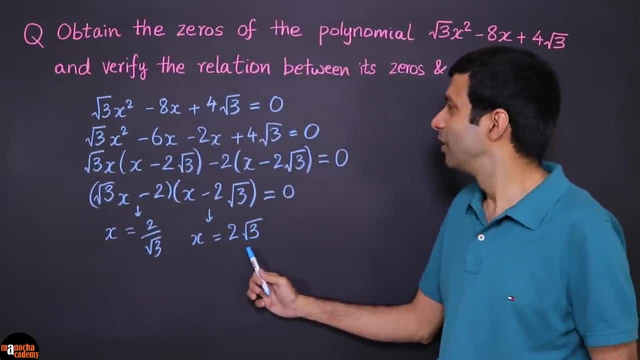 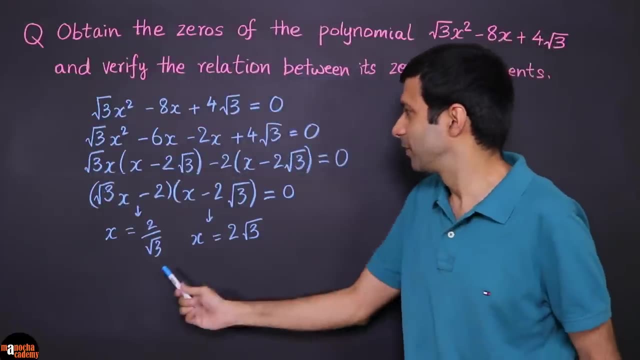 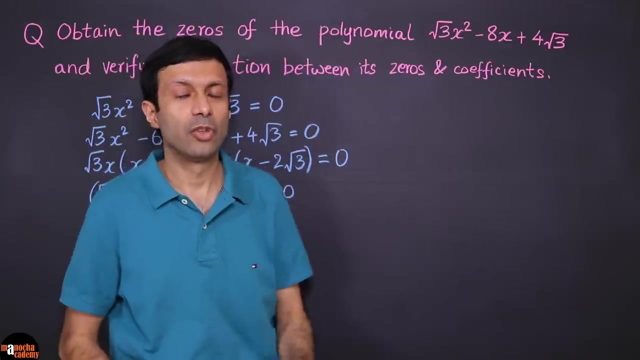 Right? So these are the zeros of the polynomial, Of our quadratic polynomial, Right? So we found the zeros here. This is our answer, And now we need to verify the relation between the zeros and the coefficients. So remember the formula that we learned: 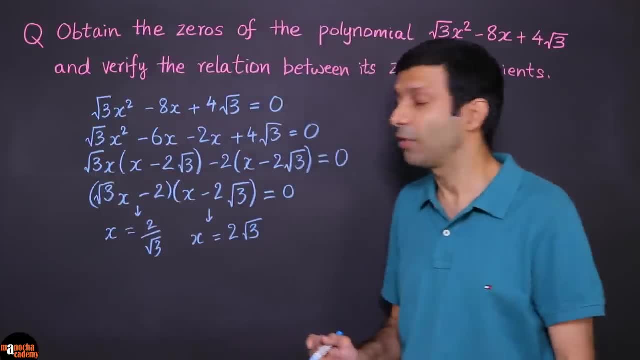 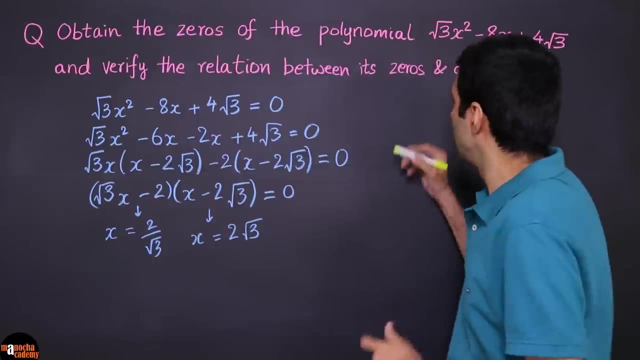 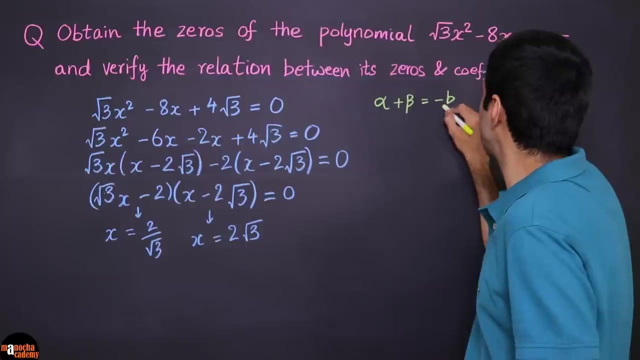 Alpha plus beta equals minus b by a, and alpha beta equals c by a. So let's apply that. So what is our formula here? So let's write that down: Alpha plus beta equals minus b by a Right, The sum of the roots. 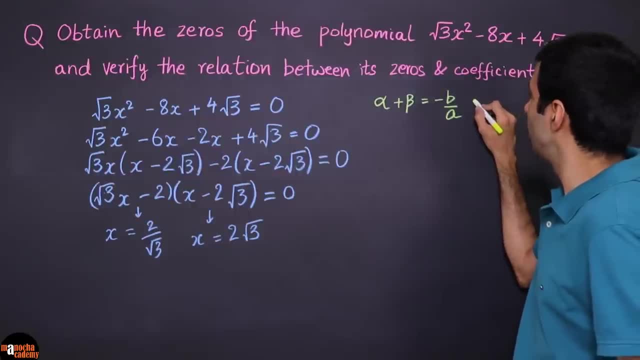 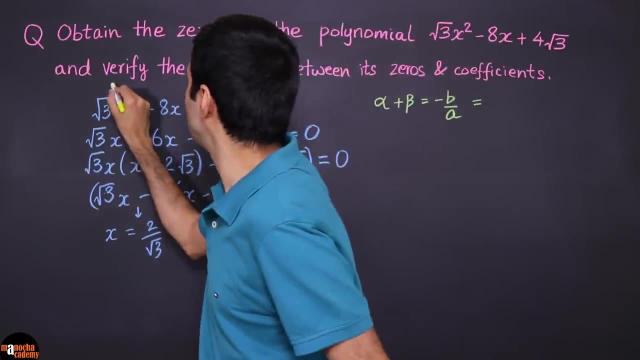 Or the sum of the zeros, And so that's going to be minus b by a. So what is the coefficient? So we are going to compare this with- remember what is the standard form of the polynomial Quadratic polynomial Ax squared plus bx, plus c. 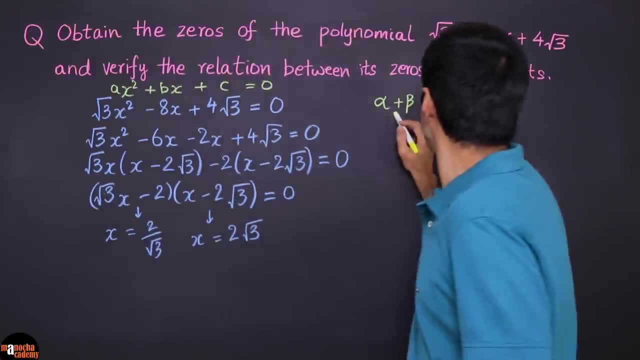 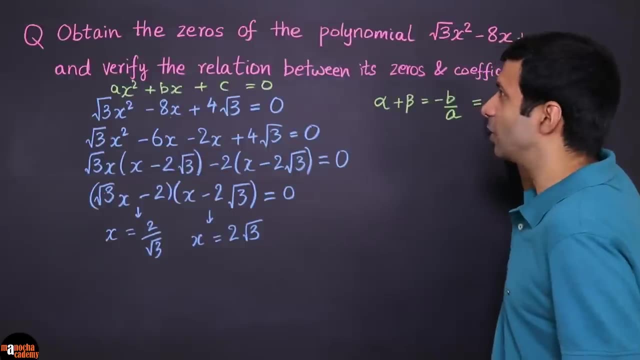 Right And that we had set equal to zero. So here b is 8.. Sorry, Minus 8.. And a is root 3. Right, So this is going to be minus of. We have b as minus 8 here. 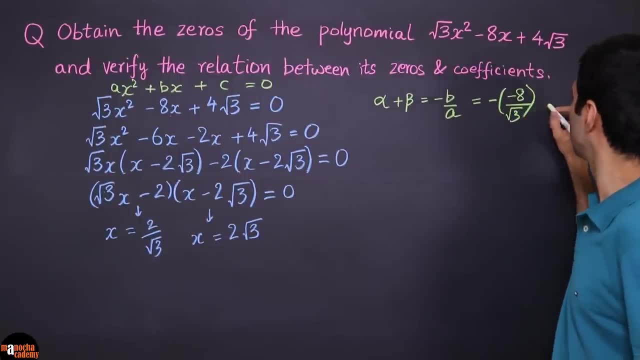 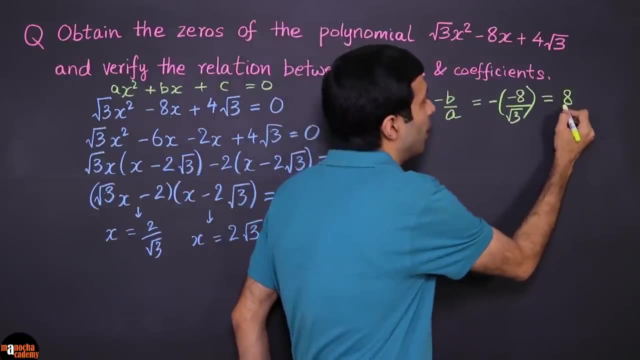 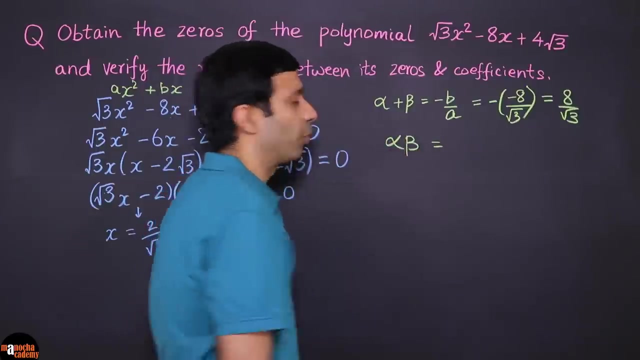 And a is root 3.. So what is the sum of the zeros going to be? It's going to be 8 by root 3.. Okay, And now let's do the product of the roots, Alpha, beta. the product of the zeros, or the roots, is going to be c by a. 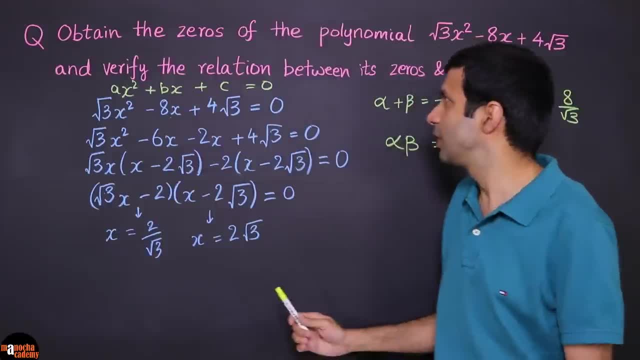 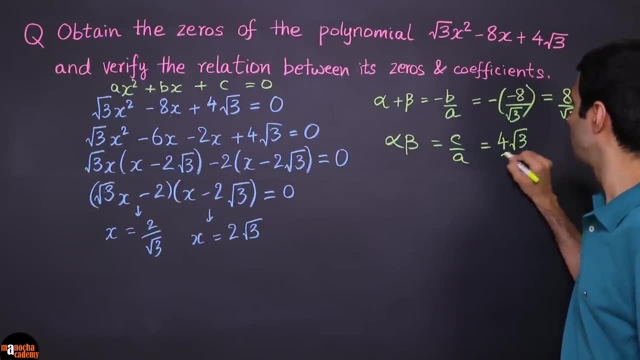 That's our formula, Right. So again we need to use our coefficient c and a. So what is the coefficient c? It's basically 4 root 3.. Right, And a is root 3.. So root 3 cancels. 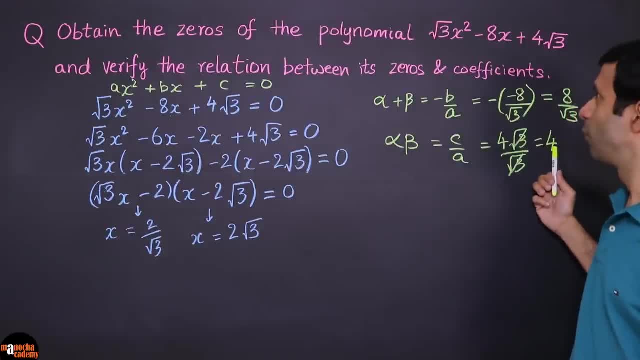 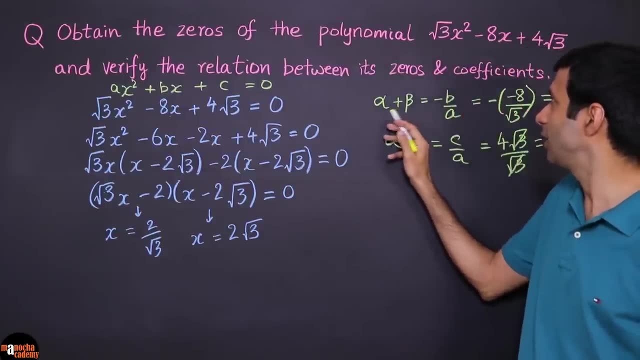 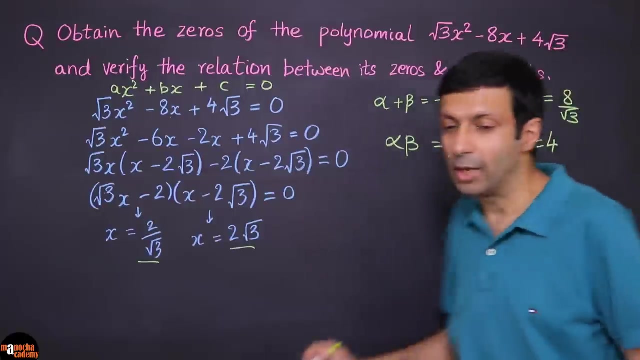 And the product of the zeros is 4.. Okay, And so, to verify this relation, because we have used this relation Right- Alpha plus beta and alpha beta- Since we know the zeros, So we are going to use it. So we are going to use it and check if these values that we got using the relation, are they right or not. 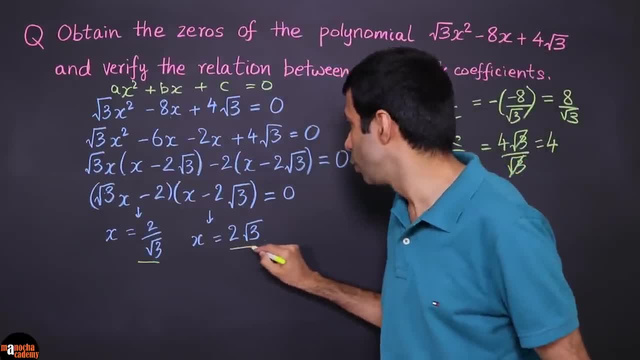 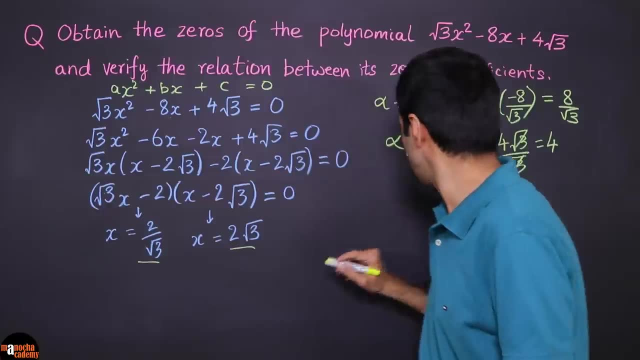 Since we know the 0s, so we are going to use it and check if these values that we have got using the relation, are they right or not. Okay, So that's pretty simple. So first thing you'll do is take alpha plus beta. 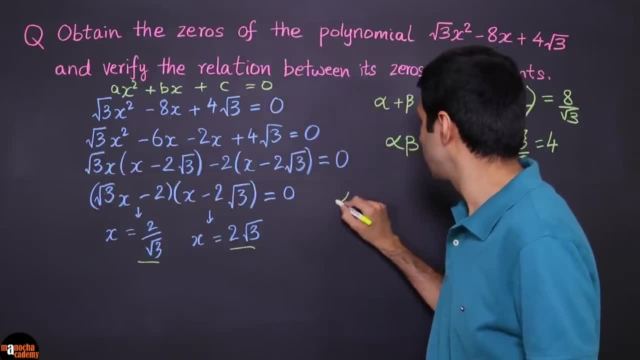 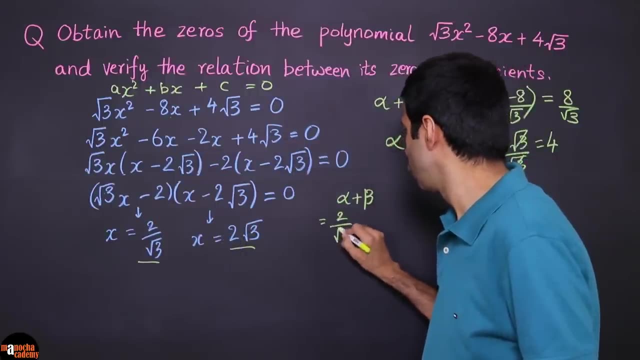 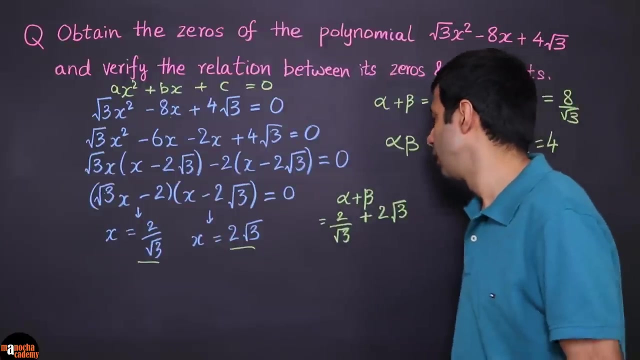 Okay, So that's pretty simple. So first thing you will do is take alpha plus beta. Let's do that. So that's going to be 2 by root 3 plus 2 root 3.. Right, Okay, And there, if we take the LCM as root 3.. 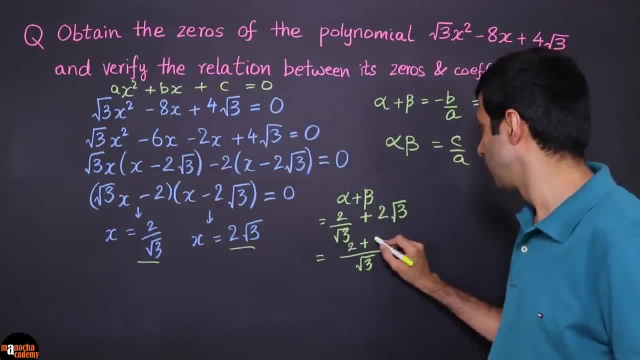 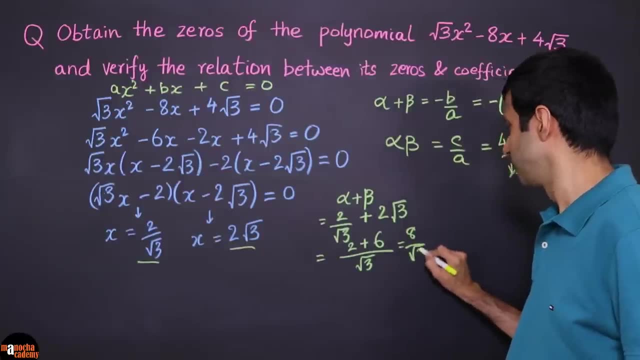 Okay, So 2 plus 2 root 3 into root 3.. That's going to be 6.. And we are going to get 8 by root 3.. Okay, So do we have the correct answer here? There you can see: alpha plus beta is 8 by root 3.. 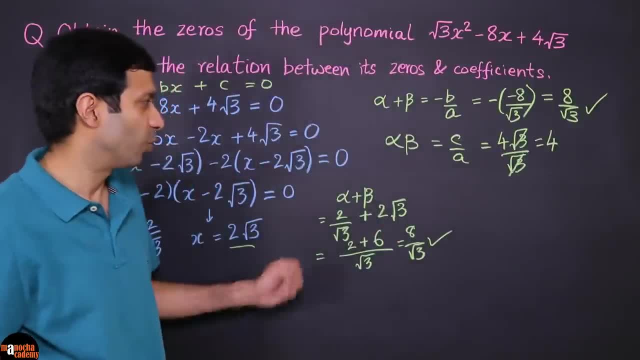 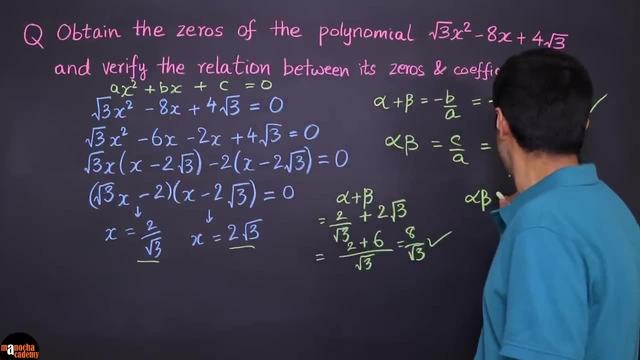 And that's what we have got from our relation minus b by a. So we have verified that. And now let's quickly verify the product of the zeros, Right? So we are going to solve for alpha beta, And that's pretty simple. 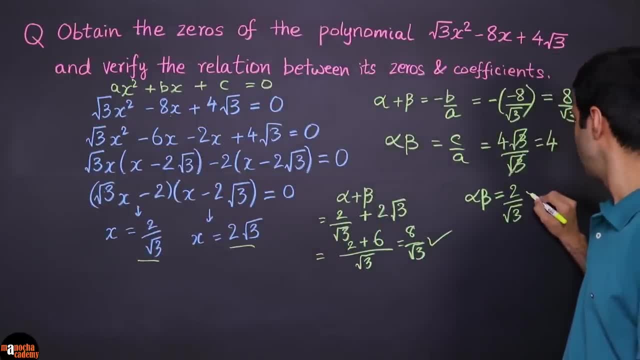 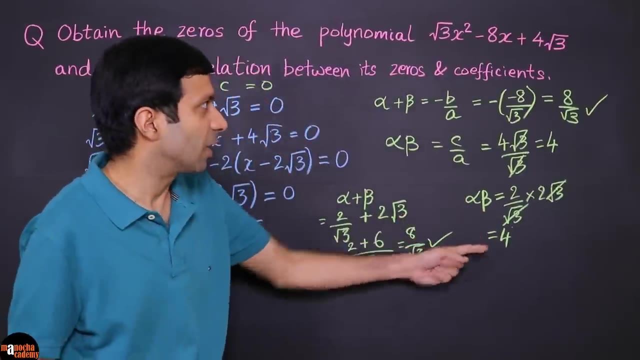 Because it's going to be 2 by root 3 into 2 root 3.. Okay, And so the root 3 gets cancelled there And we get 4.. So here, if you take a look, we got alpha beta by using the zeros as 4.. 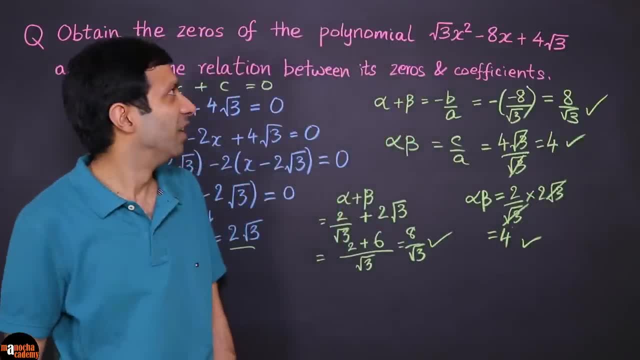 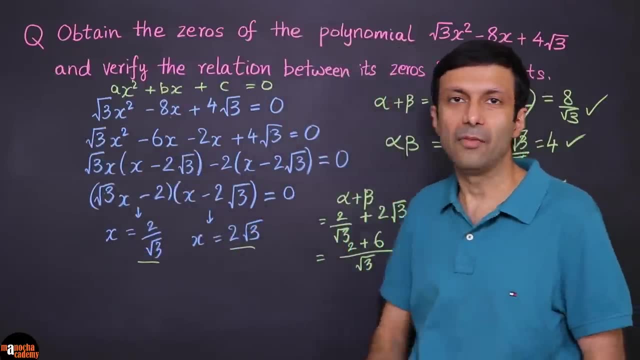 And that matches exactly what we got in our relation. So that's the main thing here in this question. First we use factorization and we solve for the zeros, And then we used our formula: alpha plus, beta minus b by a, alpha beta c by a. 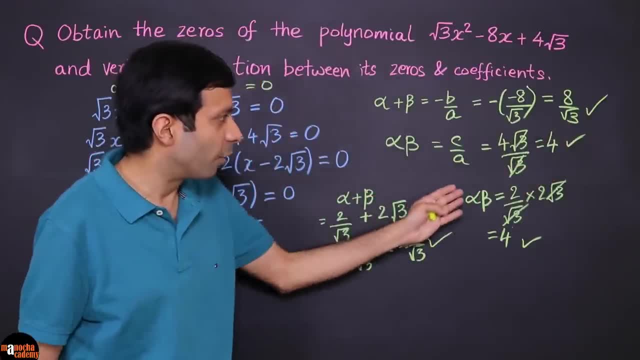 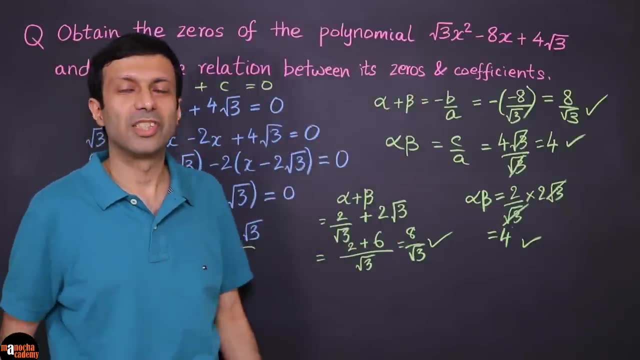 And got the values and verified that from the roots itself, And so you can see that it's matching. So the relation between the zeros and the coefficients is also verified here. So it's pretty simple, Right? Are you ready for the next question? 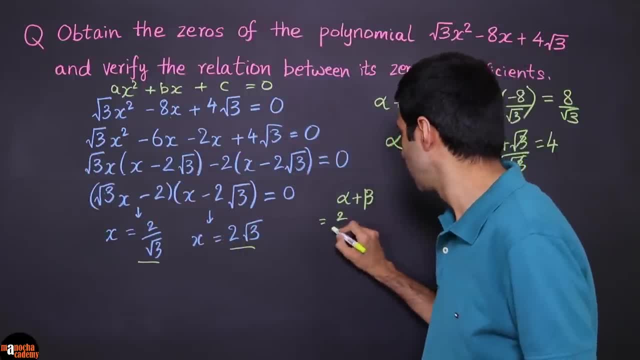 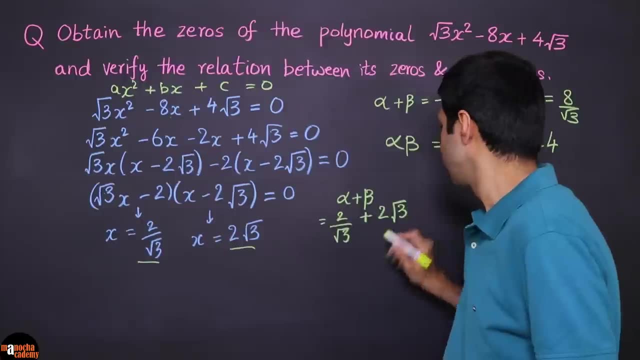 Let's do that. So that's going to be 2 by root, 3 plus 2 root 3.. Right, Okay. And then if we take the LCM as root, 3.. Okay, 2 plus 2 root 3 into root 3.. 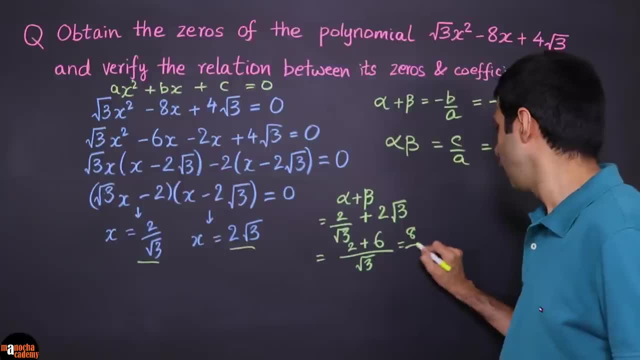 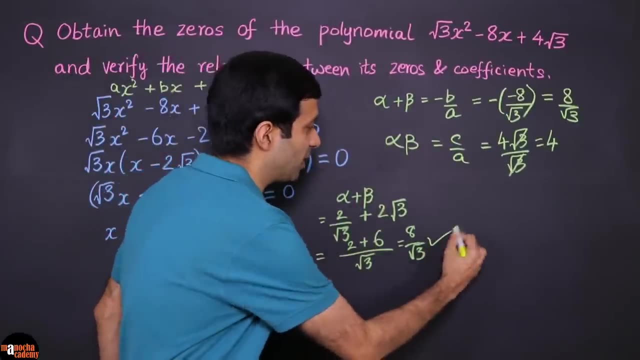 That's going to be 6. And we are going to get 8 by root 3.. Okay, So do we have the correct answer here? There you can see, alpha plus beta is 8 by root 3. And that's what we have got from our relation, minus b by a. 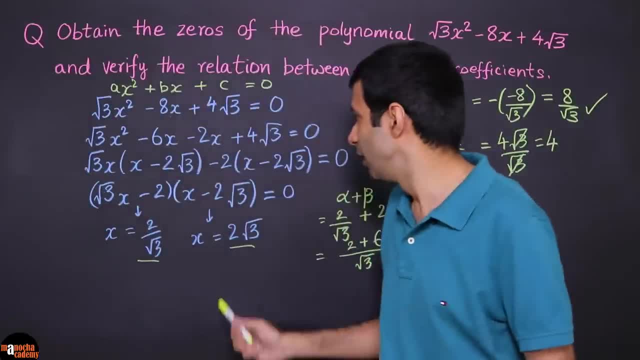 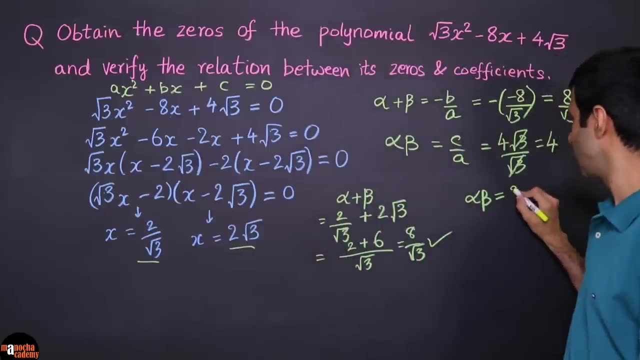 So we've verified that, And now let's quickly verify the product of the 0s Right? So we are going to solve for alpha beta, And that's pretty simple, Because it's going to be 2 by root, 3.. 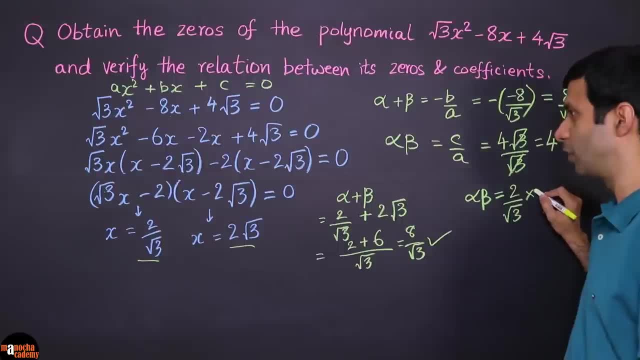 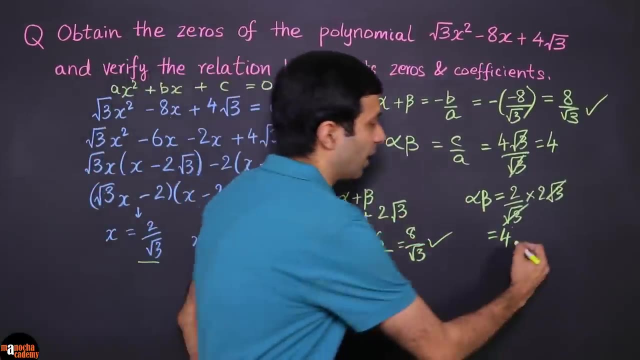 That's going to be 2 root 3 into sorry 2 by root 3 into 2 root 3.. Okay, And so the root 3 gets cancelled there And we get 4.. So here, if you take a look, we got alpha beta by using the 0s as 4.. 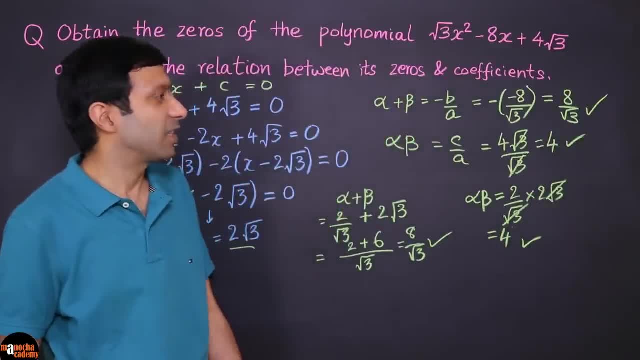 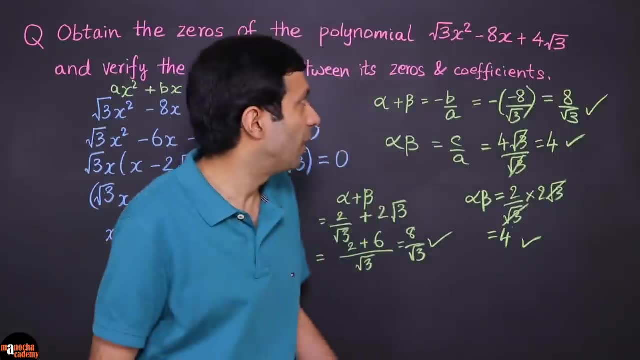 And that matches exactly what we got in our relation. So that's the main thing here in this question. First we use factorization and we solve for the 0s, And then we used our formula Alpha plus beta minus b by a. 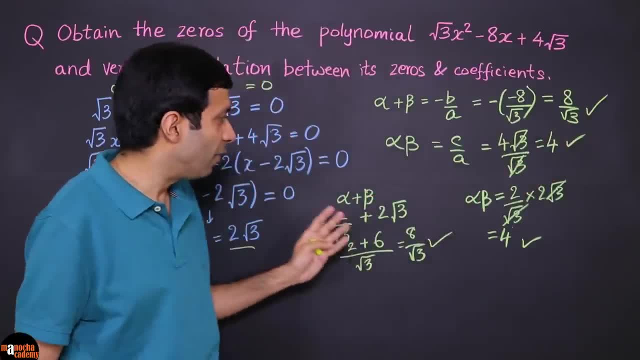 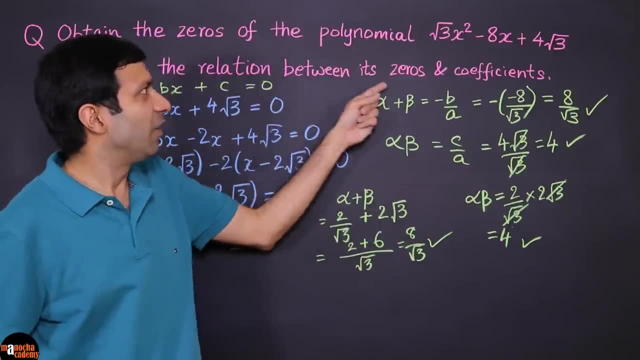 Alpha beta c by a And got the values and verified that from the roots itself, And so you can see that it's matching. So the relation between the 0s and the coefficients is also verified here. So it's pretty simple, Right. 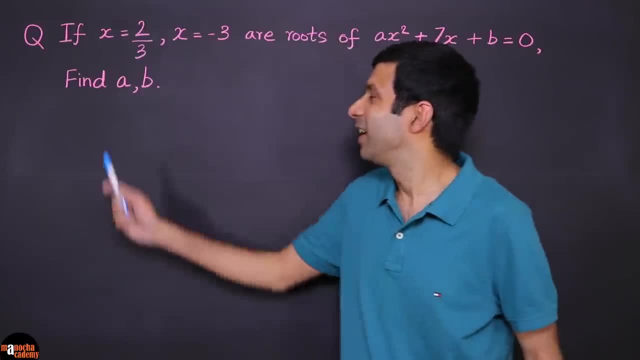 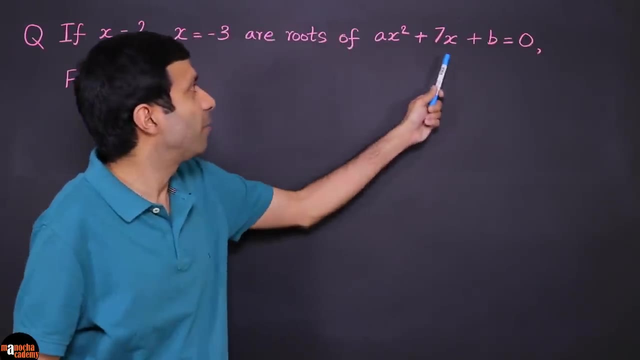 Are you ready for the next question? Here it is: If x equal to 2 by 3 and x equal to minus 3, are the roots of ax square plus 7x plus b equal to 0.. We need to find a and b. 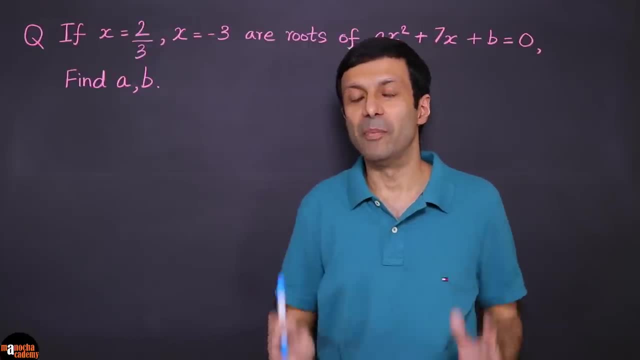 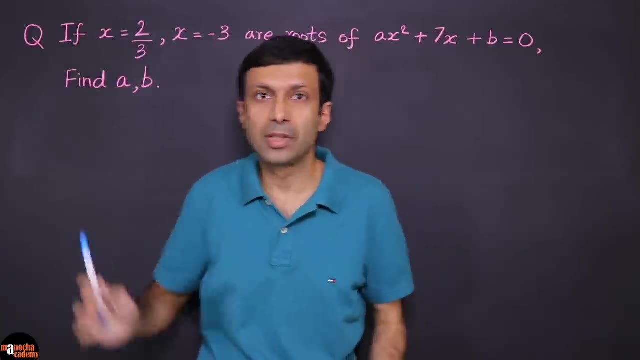 So how do we solve this? Remember the concept: If these are the roots or the 0s, that means these values. if we substitute it in our polynomial ax square plus 7x plus b, it's going to be 0.. 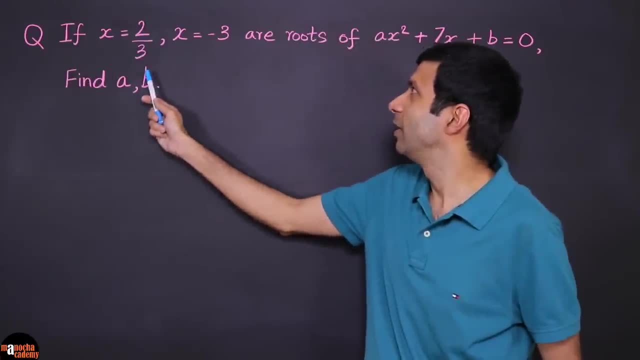 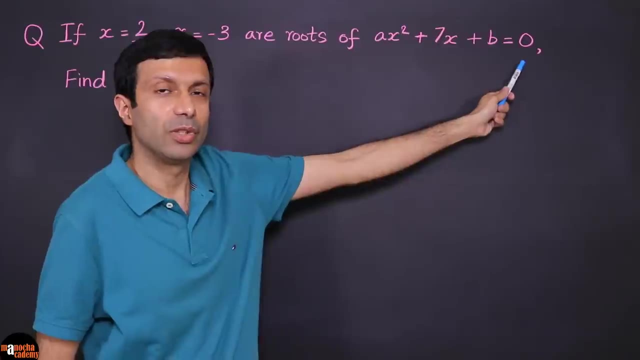 Here it is. If x equal to 2 by 3 and x equal to minus 3, are the roots of ax square plus 7x. Okay, If ax square plus 7x plus b equal to 0, we need to find a and b. 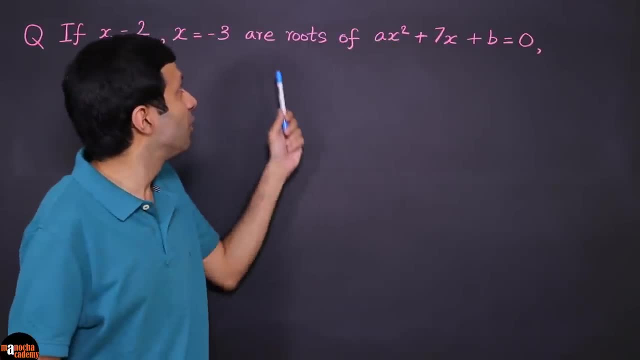 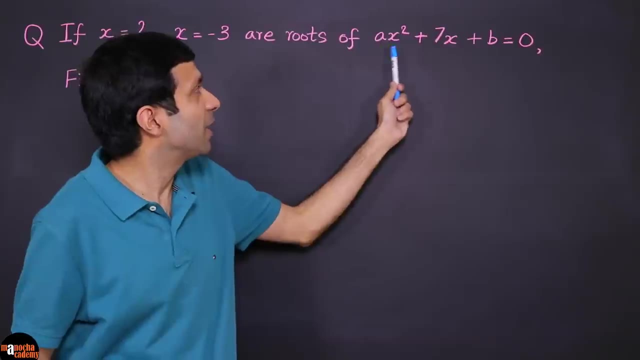 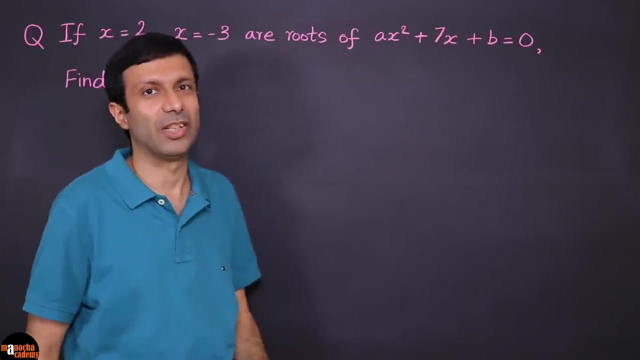 So how do we solve this? Remember the concept: If these are the roots or the zeros, that means these values. if we substitute it in our polynomial ax square plus 7x plus b, it's going to be 0. Which means it's going to satisfy this equation here. 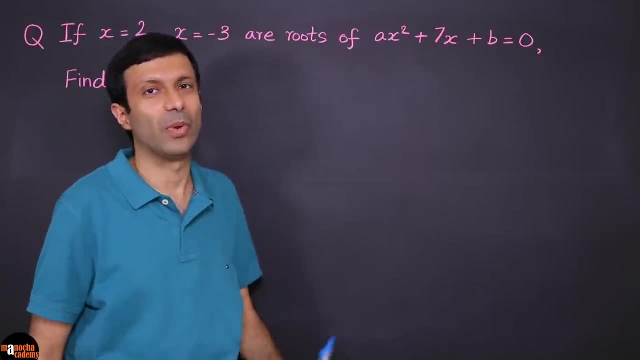 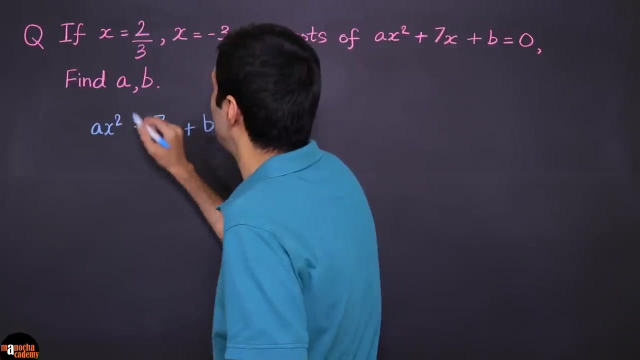 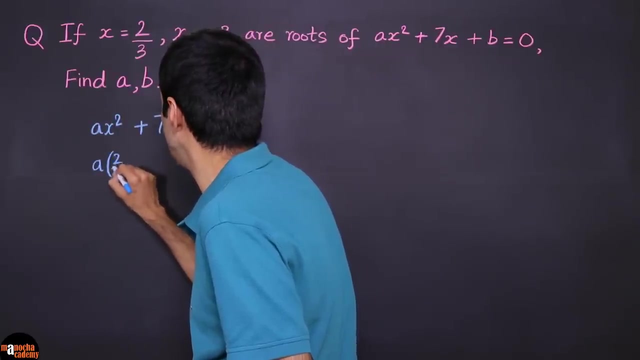 Which means it's going to satisfy this equation here. So let's write down our equation, Which is: ax square, Ax square Plus 7x, Right Plus b equal to 0.. And now let's simply substitute these values. So let's substitute the first value is going to be a into 2 by 3 whole square. 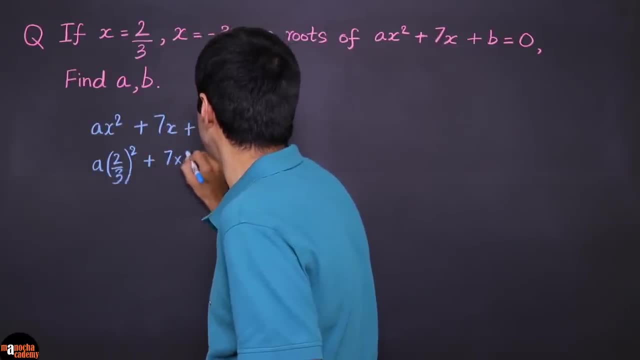 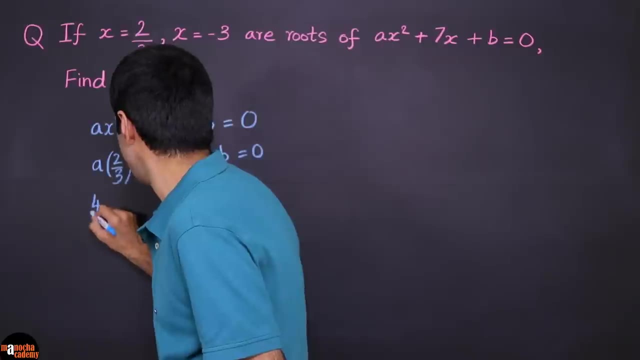 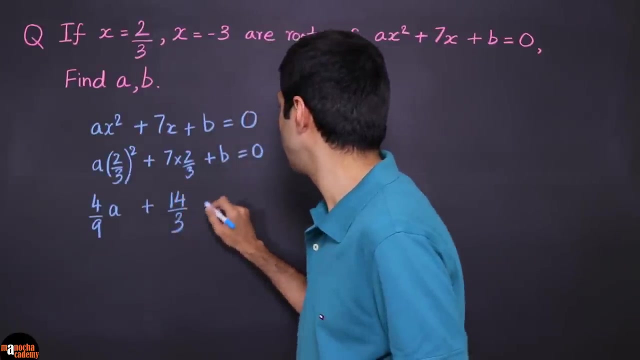 Right Plus 7 into 2 by 3. Plus b equals 0. So if we simplify that, we'll get 4 by 9, a Plus 14 by 3, b Plus 14 by 3. Sorry. 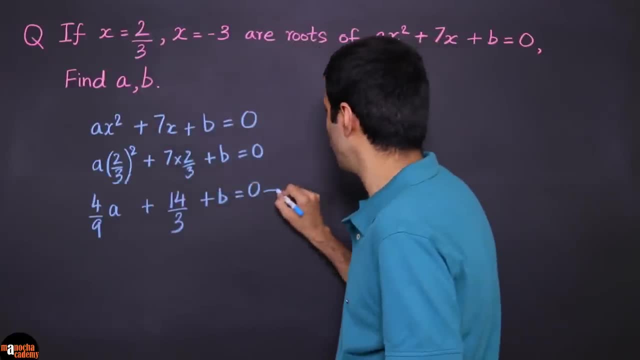 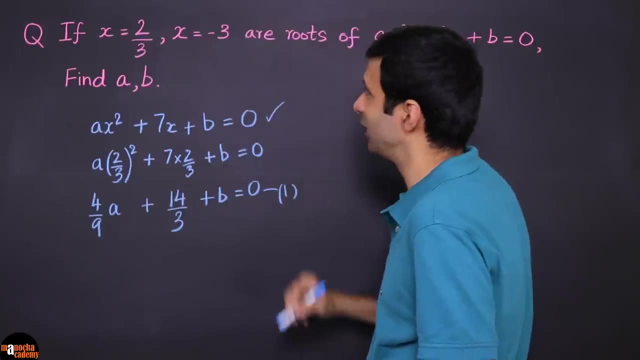 Plus b equals 0.. Okay, So this is our first equation. And now let's substitute the next value, x, equal to minus 3.. Again in this equation, Right? So what do we get? We are going to get a into minus 3, whole square. 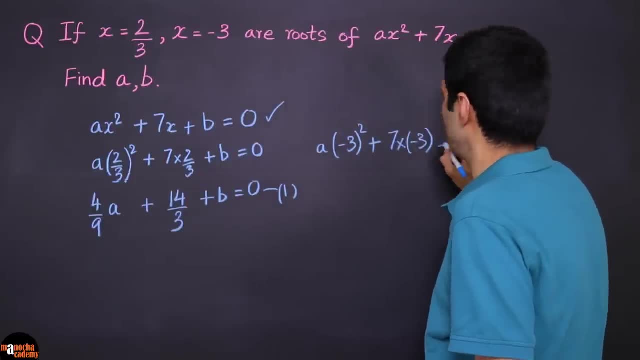 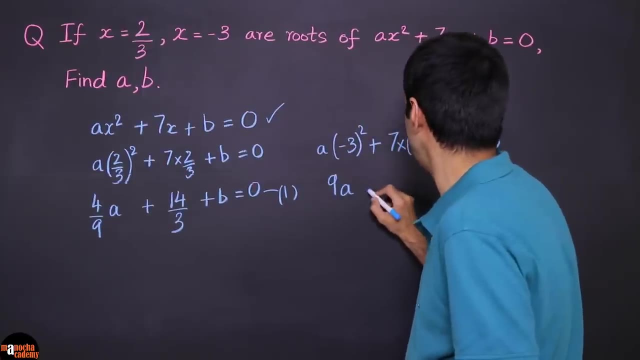 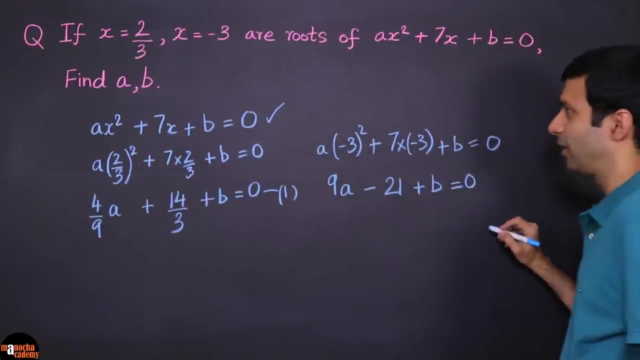 Plus 7 into minus 3.. Plus b equals 0.. Right, And so if we simplify this, we get 9 a minus 21.. Right, Plus b equal to 0. And that's our second equation here. Okay. 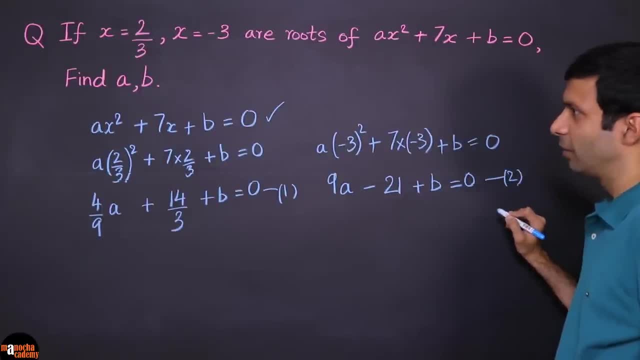 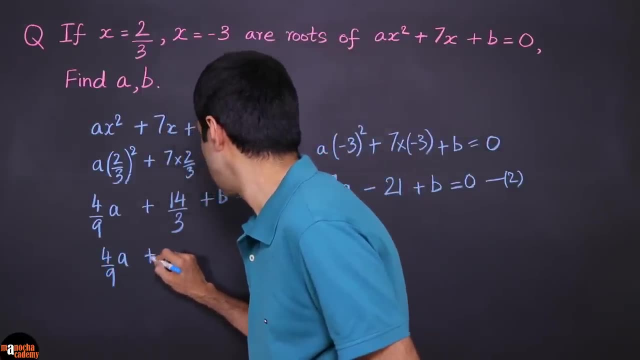 And we can rearrange and write this equation as: 4 by 9 a Plus b equals Minus 14 by 3.. Plus b equals Minus 14 by 3.. Right, So that was our first equation rearranged. 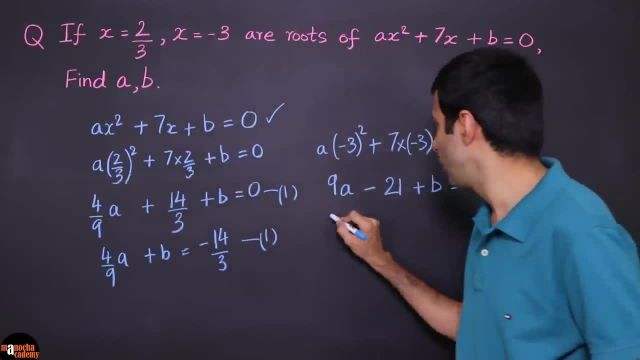 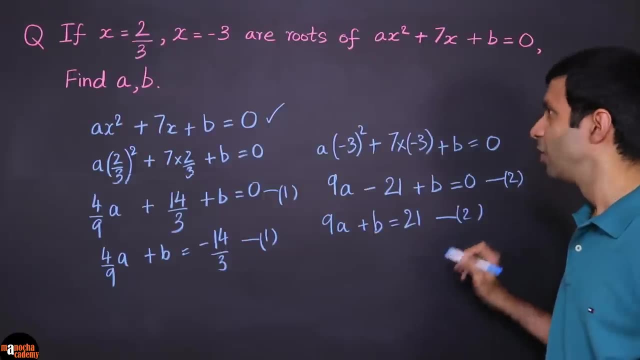 And, similarly, here we have 9 a Plus b Equals 21.. Okay, So now it's pretty simple, Because we need to find a and b And, as you can see, We have two equations. So right, So we have a pair of linear equations. 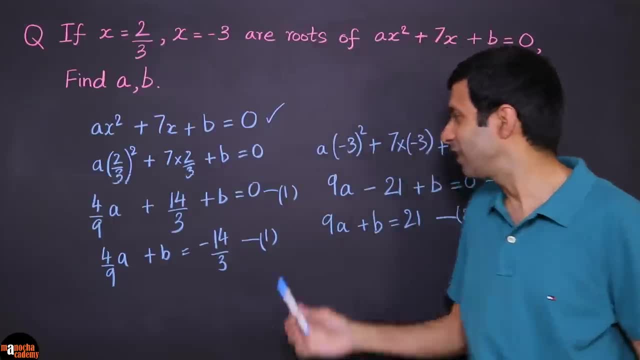 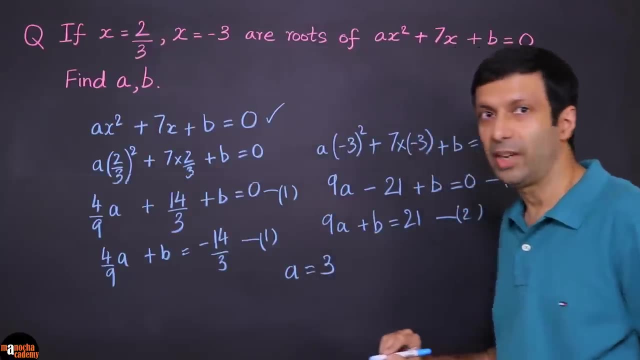 Two linear equations in two variables. So you can simply solve that. And if you go ahead and solve it, You're going to get the values. So try this out yourself. You're going to get a equal to 3. And b equal to minus 6.. 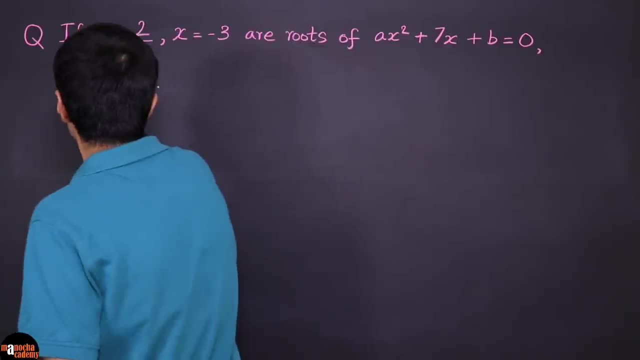 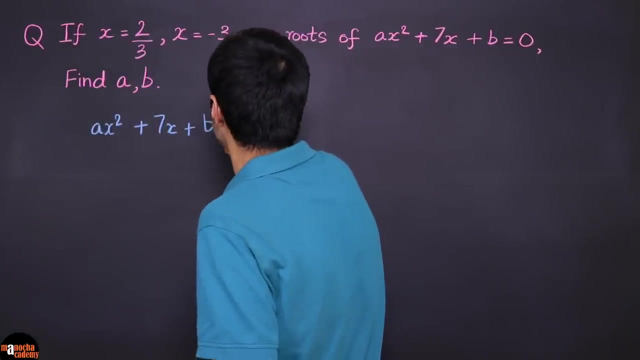 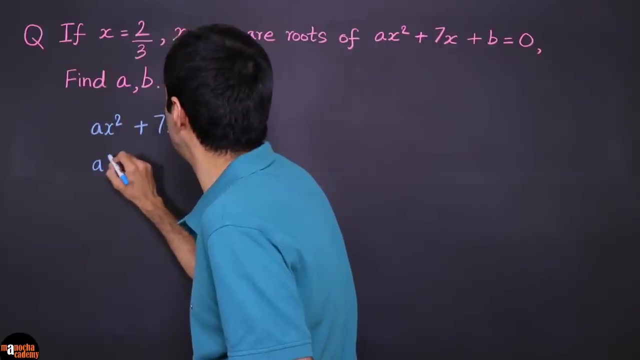 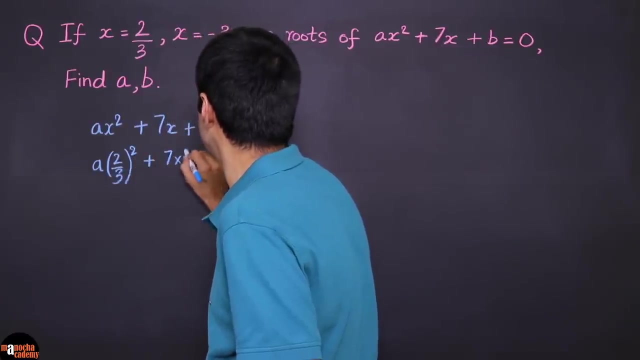 So let's write down our equation, Which is: ax square plus 7x right plus b, equal to 0.. And now let's simply substitute these values. So let's substitute. The first value is going to be a into 2 by 3 whole square right plus 7 into 2 by 3 plus b equals 0.. 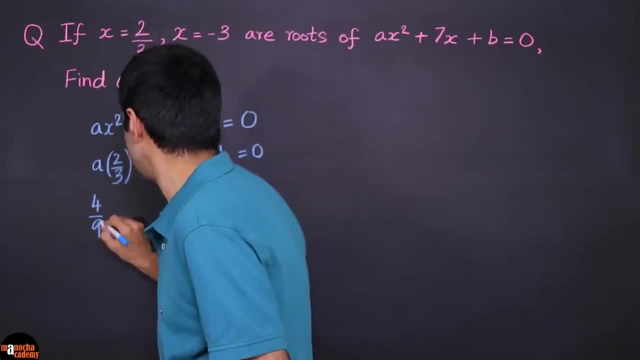 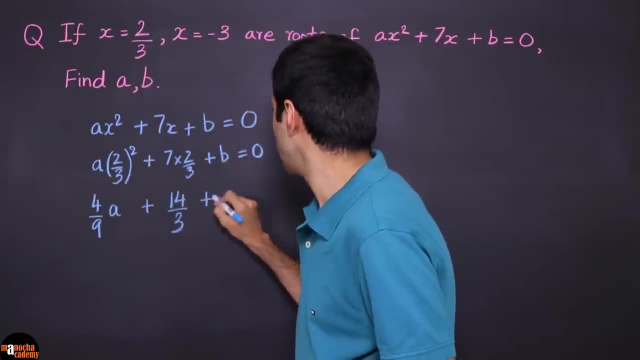 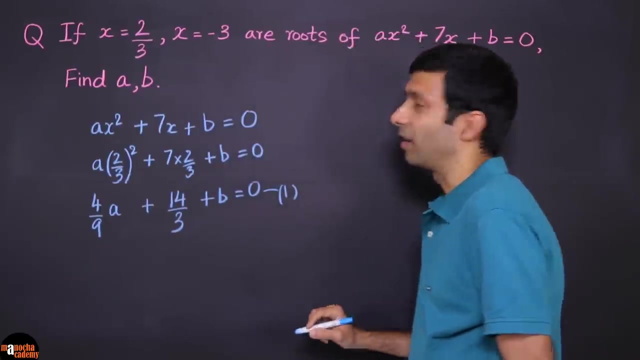 So if we simplify that, we'll get 4 by 9ax, 4 by 9a, plus 14 by 3b, plus 14 by 3, sorry, plus b equals 0.. Okay, So this is our first equation. 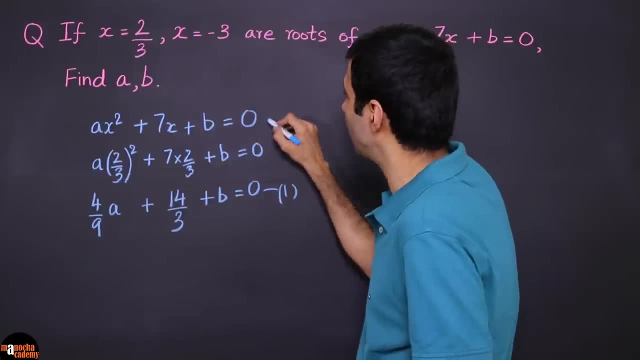 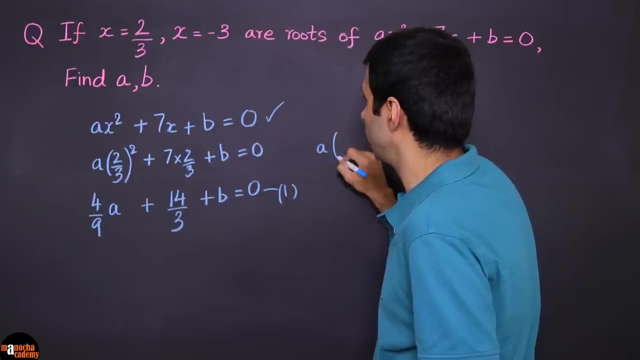 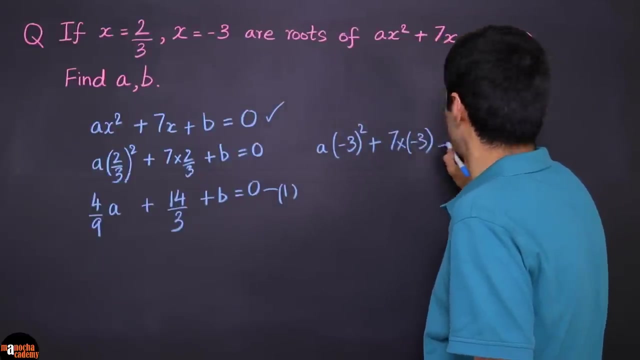 And now let's substitute the next value, x, equal to minus 3, again in this equation, right? So what do we get? We are going to get a into minus 3, whole square Plus 7 into minus 3, plus b equals 0.. 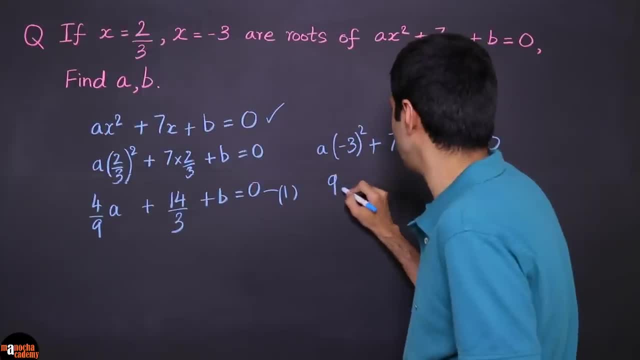 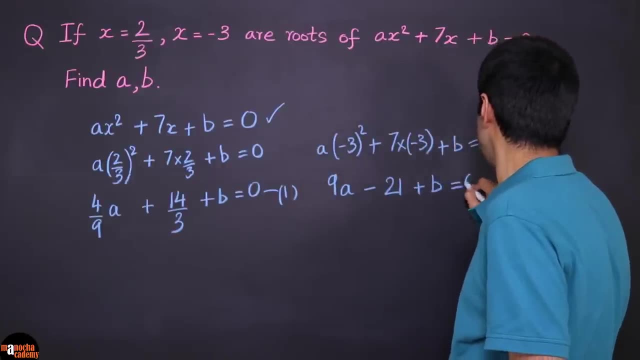 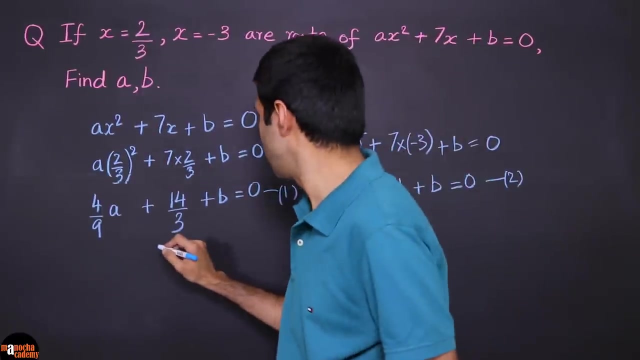 Right, And so if we simplify this, we get 9a minus 21,. right plus b equal to 0.. And that's our second equation here, Okay, And we can rearrange and write this equation as 4 by 9a. 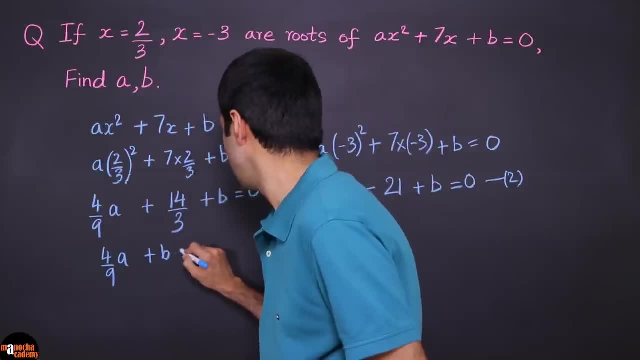 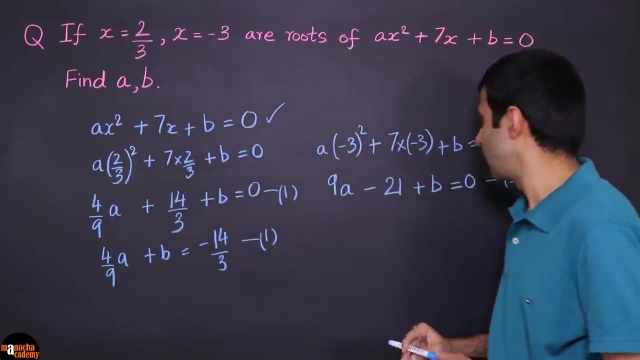 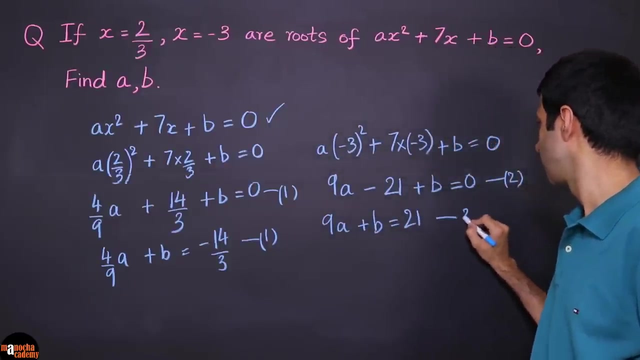 9a plus b equals minus 14 by 3, right? So that was our first equation rearranged, And similarly, here we have 9a plus b equals 21.. Okay, So now it's pretty simple, because we need to find a and b. 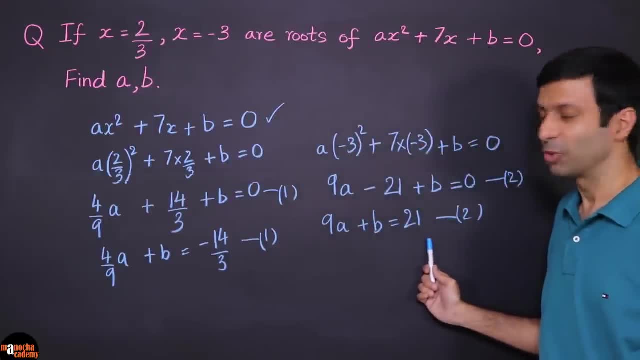 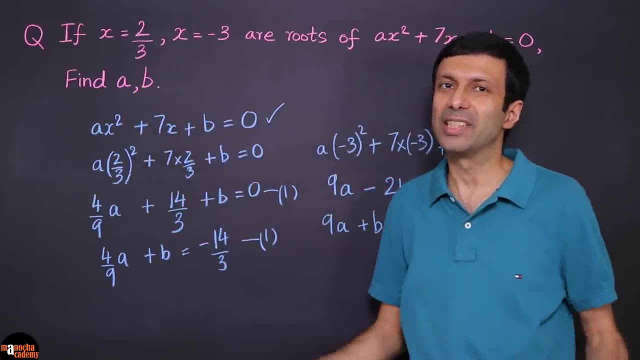 And, as you can see, we have two equations right. So we have a pair of linear equations, Two linear equations in two variables. So you can simply solve that And if you go ahead and solve it, you're going to get the values. 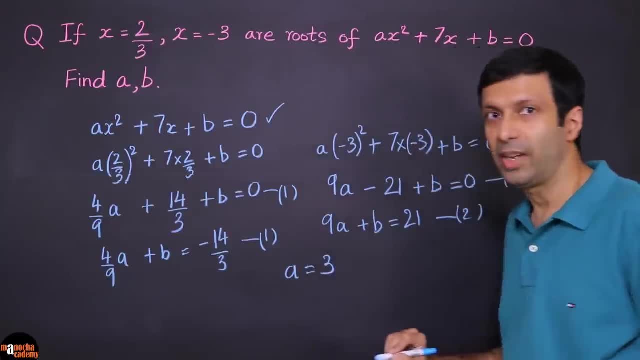 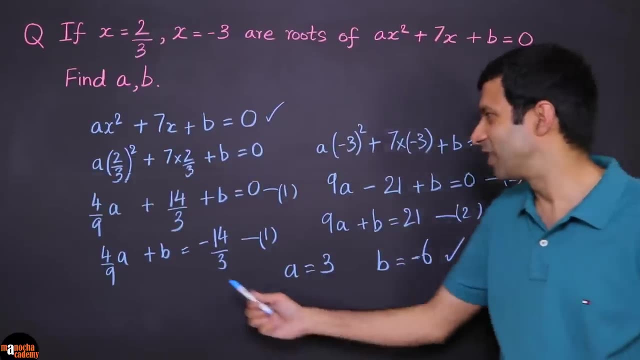 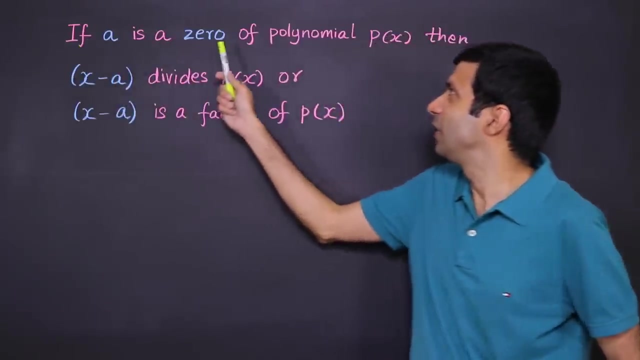 So try this out yourself. You're going to get a equal to 3 and b equal to minus 6.. So that's going to be our answer if you solve these two equations. Note this important point that if a is a 0 of a polynomial px. 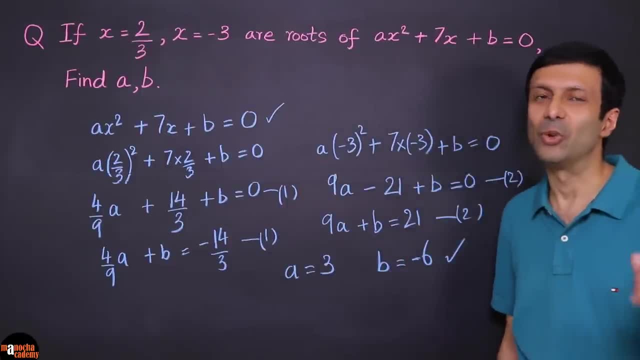 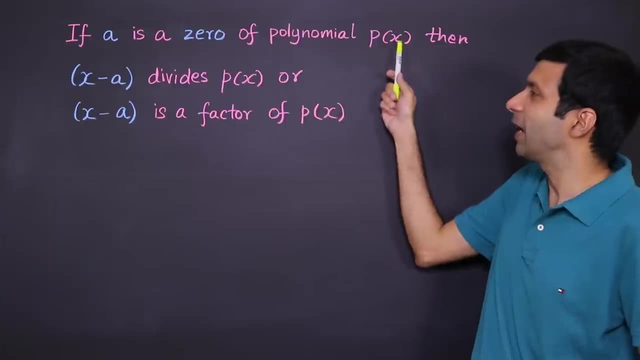 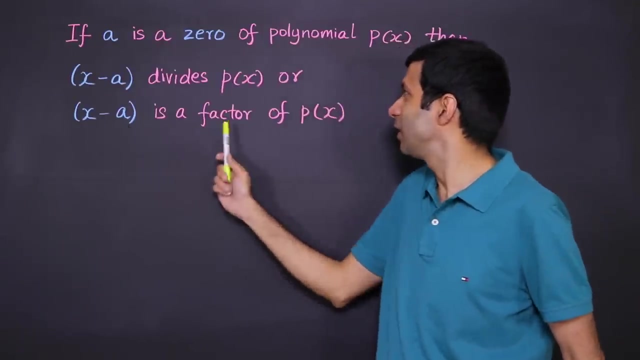 So that's going to be our answer If you solve these two equations. Note this important point That if a is a 0. Of a polynomial px, Then x minus a Divides px, Or we can say Factor of px. 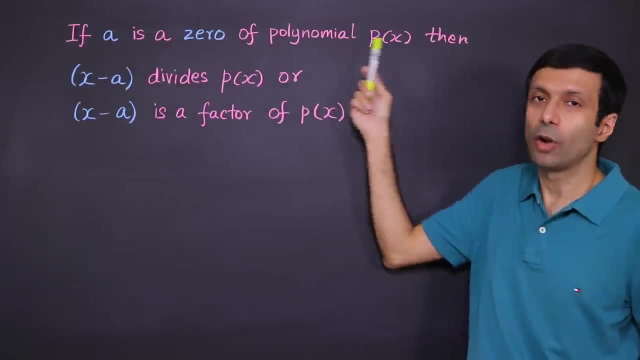 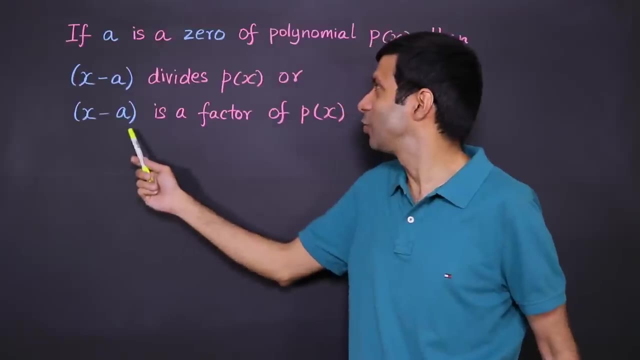 For example, Let's say 2 is a 0 of a polynomial px. Then we can say that x minus 2. Divides px, Or x minus 2 is a factor of px. Now let's solve this question. 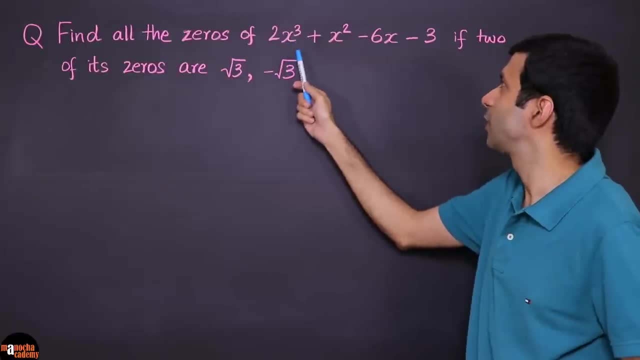 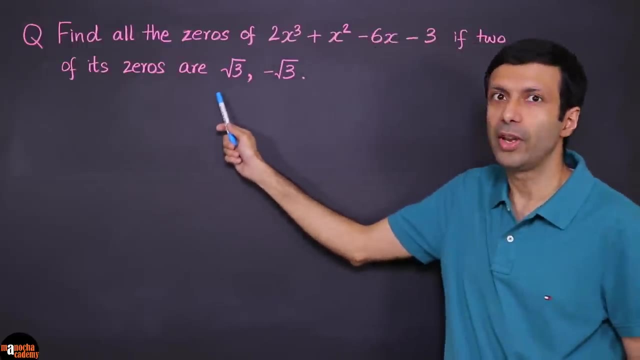 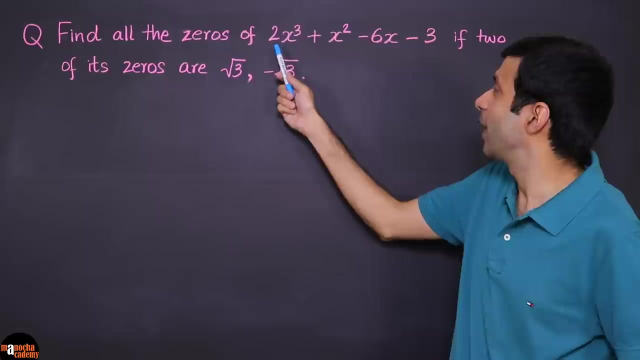 Find all the zeros Of 2x cube Plus x square, Minus 6x minus 3.. If two of its zeros Are root 3.. So how do we do this question? First, let's Write down our polynomial. 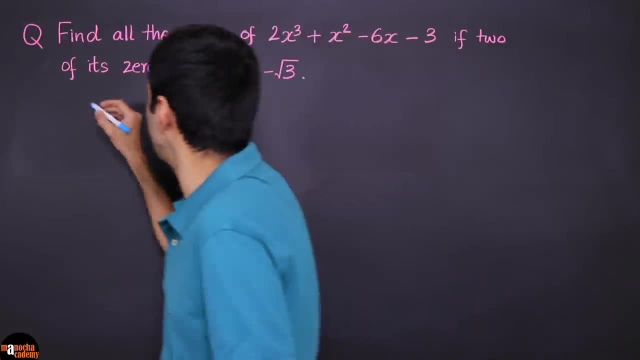 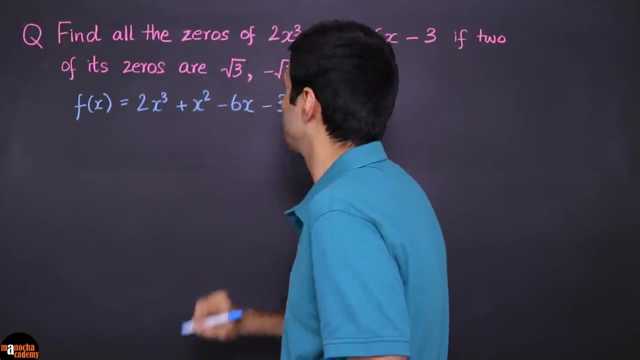 So can you see it's a Cubic polynomial here, So let's write that down. So let's say the polynomial fx Is 2x cube Plus x, square Minus, 6x Minus 3.. Okay, 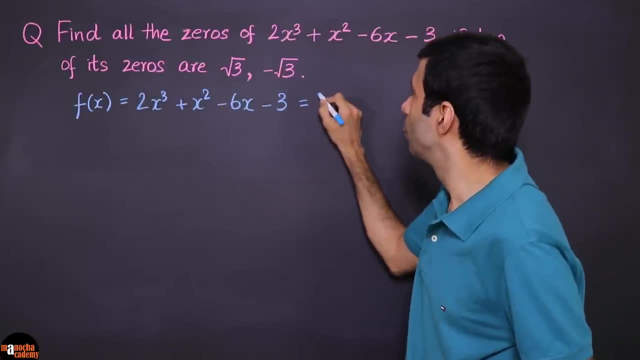 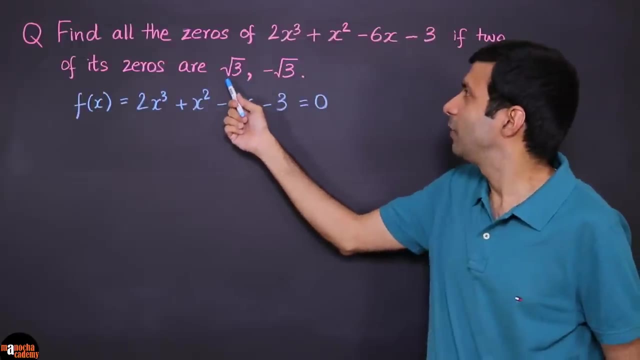 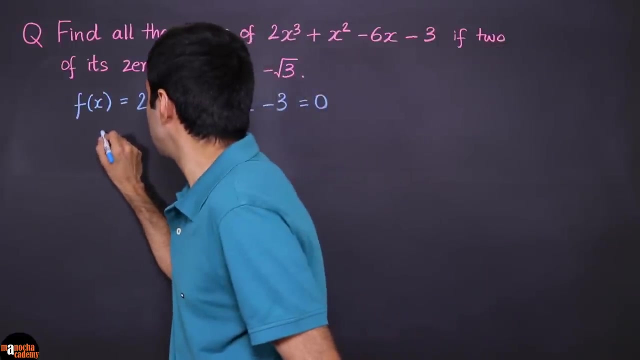 And since we want to find the zeros of the polynomial, We are going to Equate the polynomial as 0.. Now we've been given that We have these two zeros, Root 3. And minus root 3.. So we can say that: 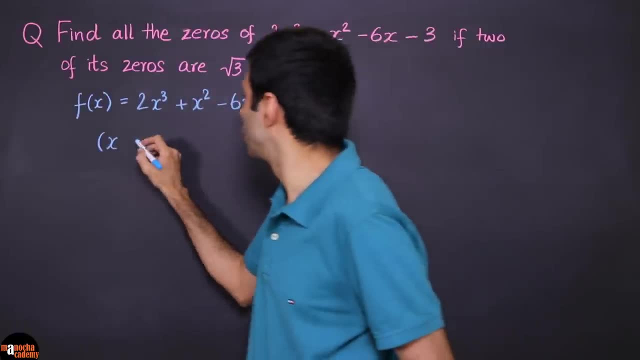 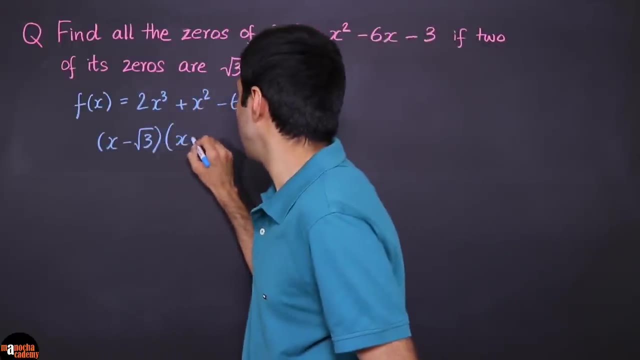 x minus the Zeros of the roots, So it's going to be x minus root 3.. And x minus of minus root 3 will be x plus root 3.. So can we say that These are factors of fx? 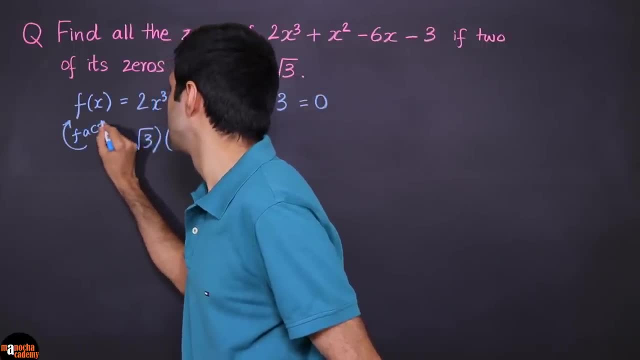 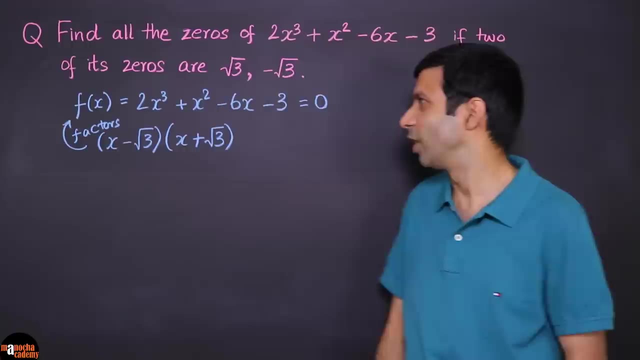 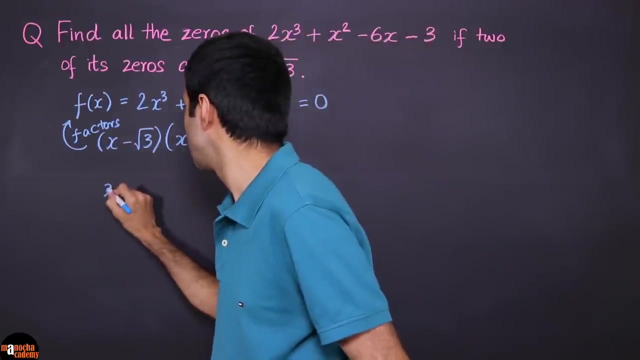 Right, So these are Factors of fx Because they divide it. Right, Because these are the zeros of this polynomial. So now, if we multiply this, So it's going to be- you can use A plus b into a minus b. 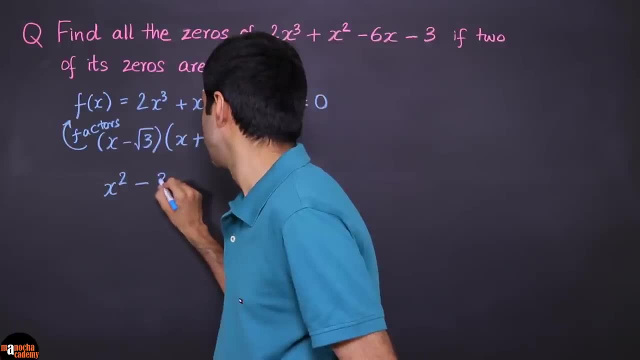 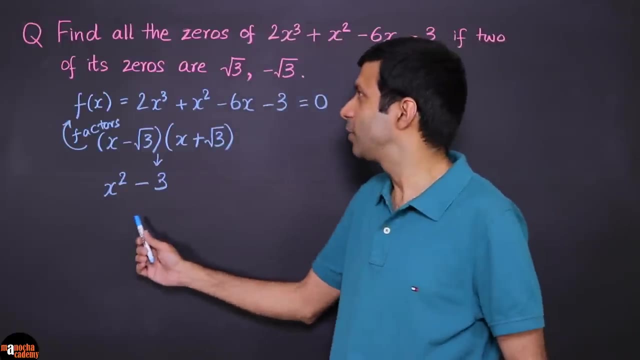 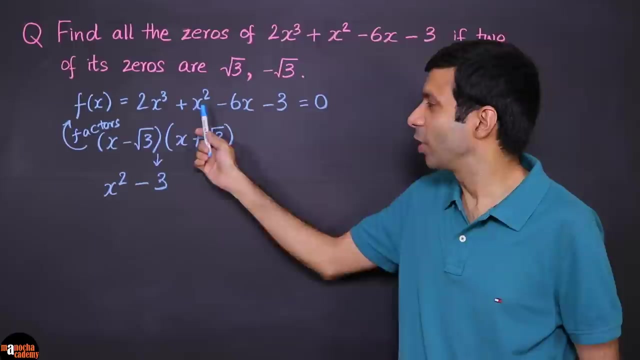 And it's going to be x square Minus 3.. Multiplying these two out, We get x square minus 3.. So x square minus 3.. Of this polynomial fx That means This is: This polynomial can be divided by this: 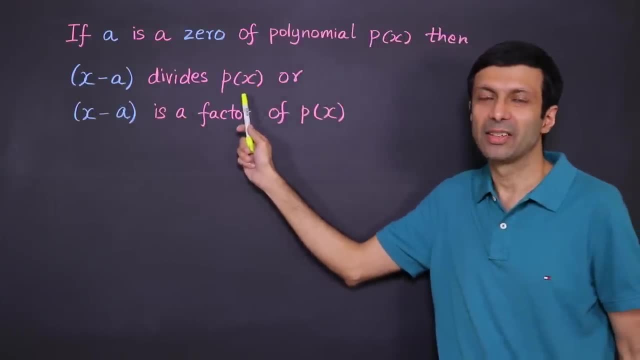 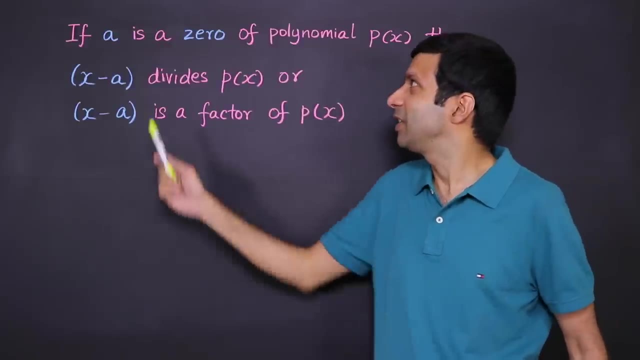 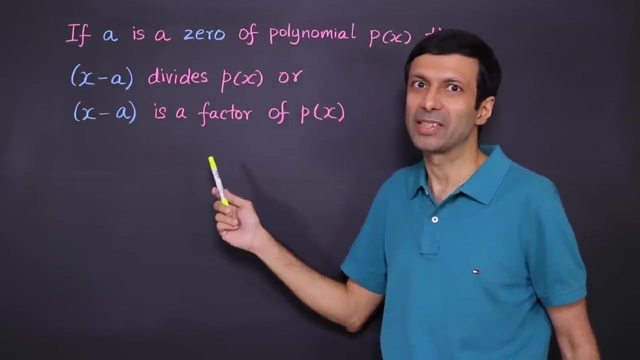 then x minus a divides px. Or we can say x minus a is a factor of px. For example, let's say 2 is a 0 of a polynomial px, Then we can say that x minus 2 divides px, Or x minus 2 is a factor of px. 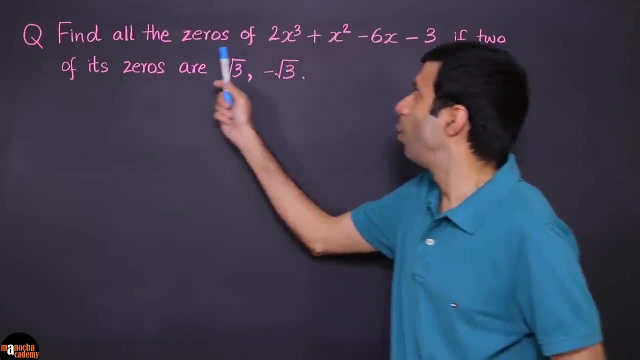 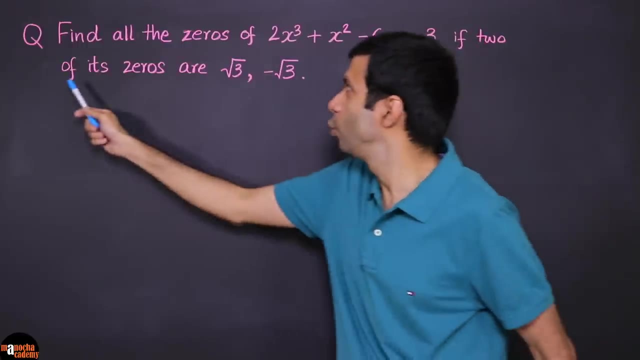 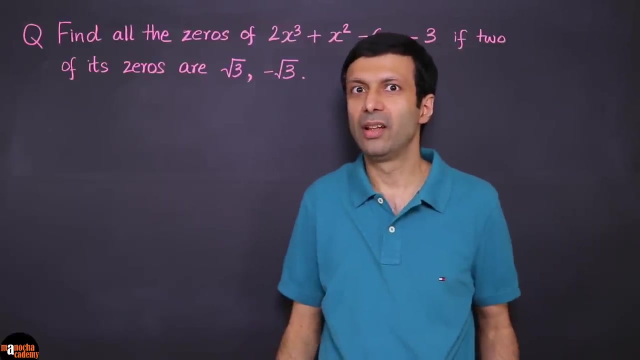 Now let's solve this question. Find all the 0s of 2x cubed plus x squared, minus 6x minus 3, if two of its 0s are root 3 and minus root 3.. So how do we do this question? 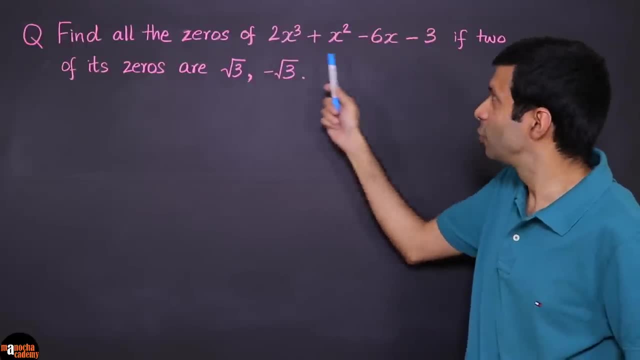 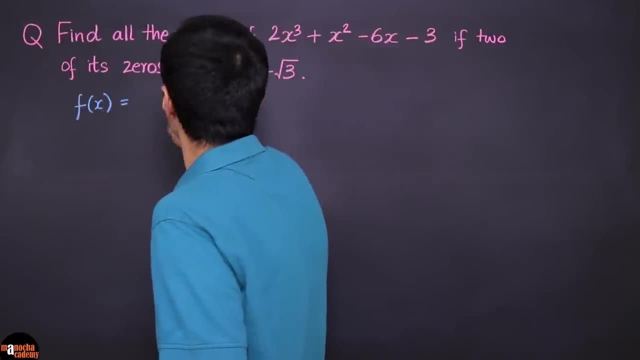 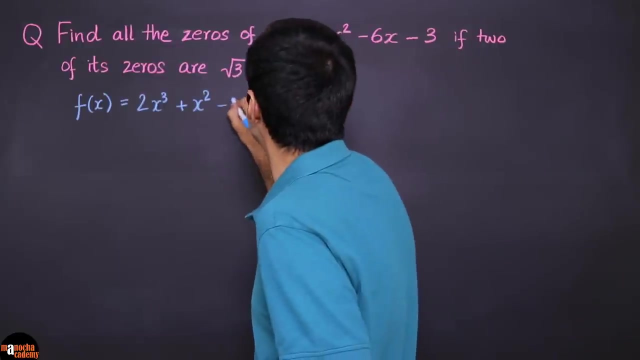 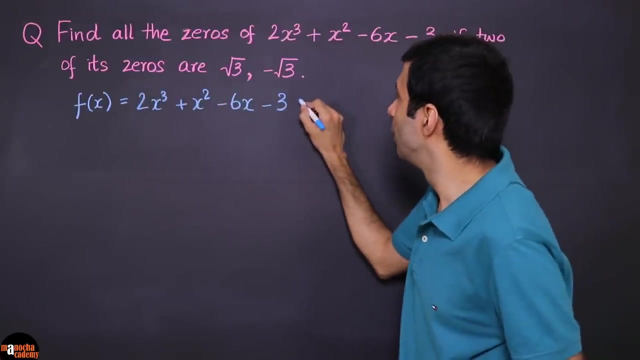 First let's write down our polynomial. So can you see? it's a cubic polynomial here, So let's write that down. So let's say, the polynomial fx is 2x cubed plus x squared minus 6x. And since we want to find the 0s of the polynomial, 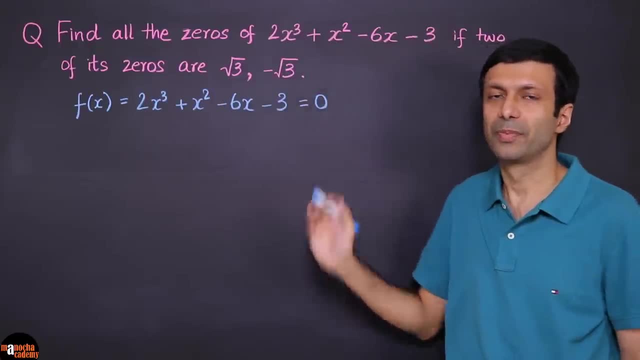 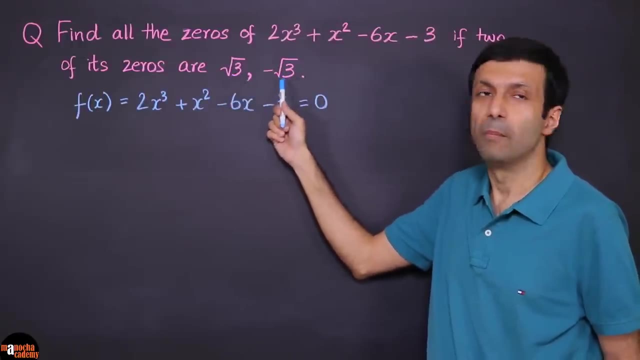 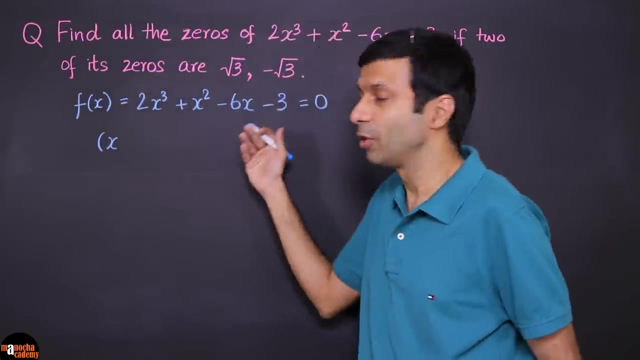 we are going to equate the polynomial as 0.. Now we've been given that we have these two 0s, root 3 and minus root 3.. So we can say that x minus the 0s of the roots, so it's going to be x minus root 3,. 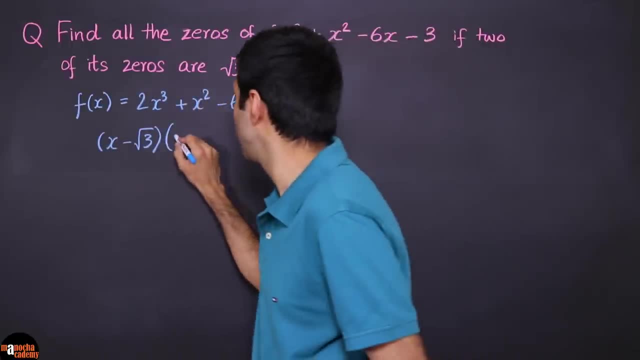 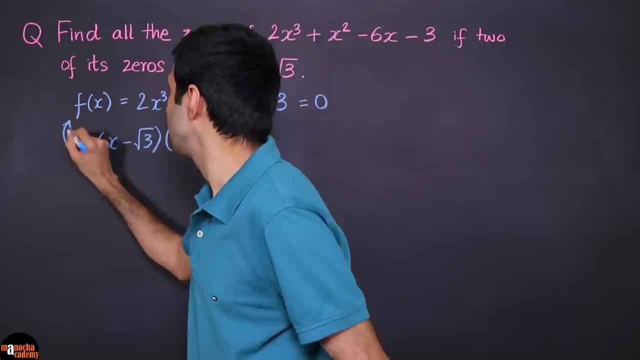 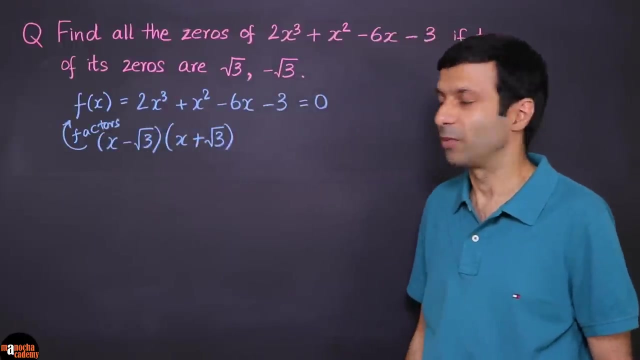 and x minus of minus root 3 will be x plus root 3.. So can we say that these are factors of fx? right? So these are factors of fx because they divide. it right, Because these are the 0s of this polynomial. 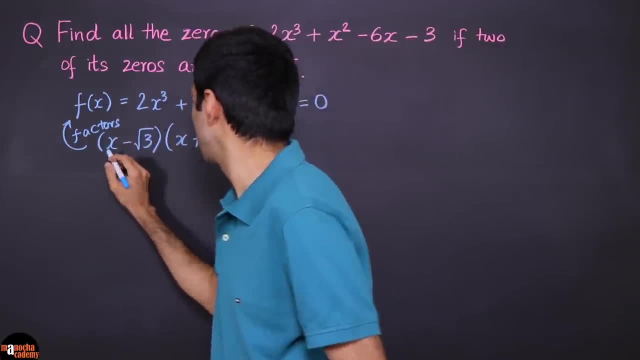 So now, if we multiply this, so it's going to be, you can use a plus b into a minus b and it's going to be x squared, So it's going to be x squared minus 3.. Multiplying these two out, we get x squared minus 3.. 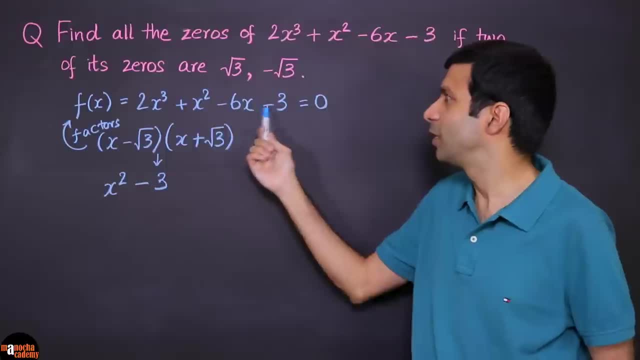 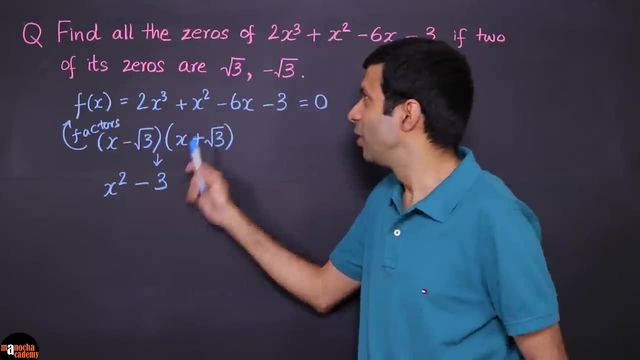 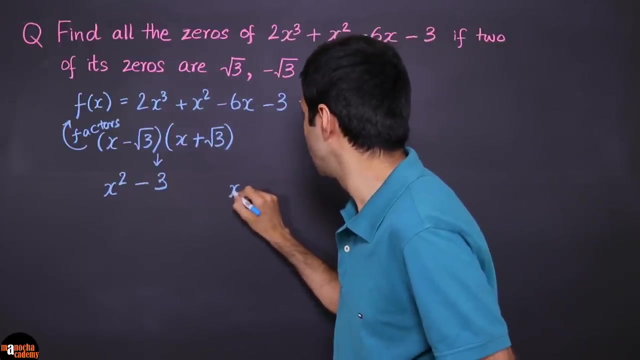 So x squared minus 3 is a factor of this polynomial fx. That means this polynomial can be divided by this right. So if we divide these two, so if we divide the polynomial by x squared minus 3, so let's write it like this: 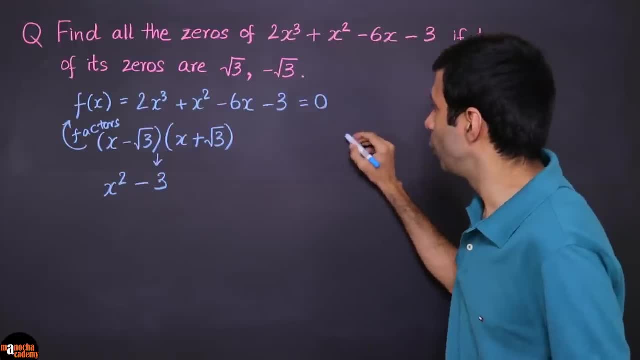 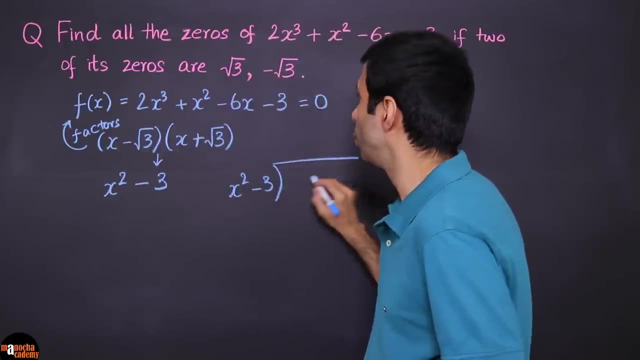 Right. So if we divide these two, So if we divide the polynomial by x square minus 3.. So let's write it like this: So x square minus 3.. If we sit and do this division, So 2x cube. 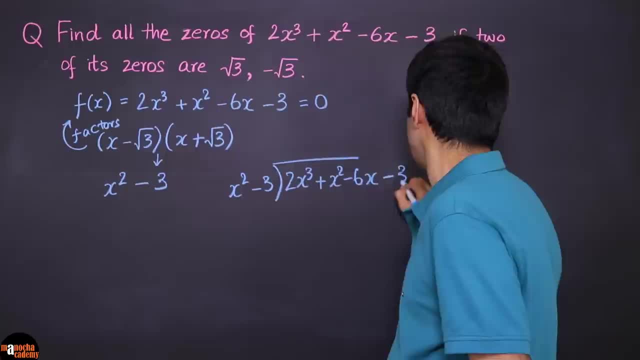 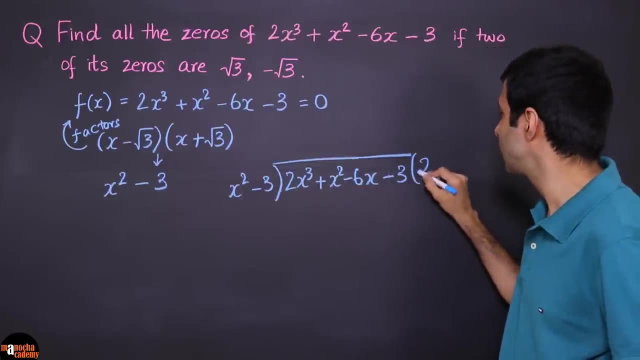 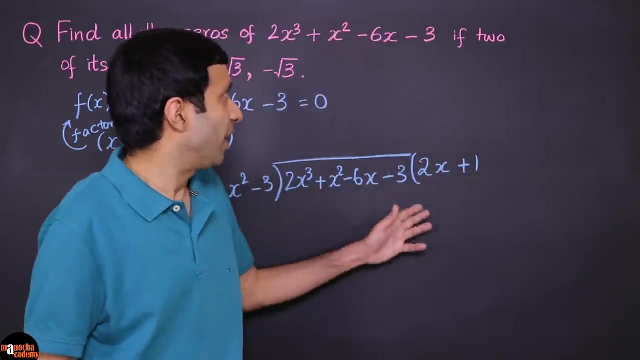 Plus x square Minus, 6x Minus 3.. Right, And you solve this. You're going to get the quotient as 2x plus 1.. Okay, So now how can we find the Other zero? 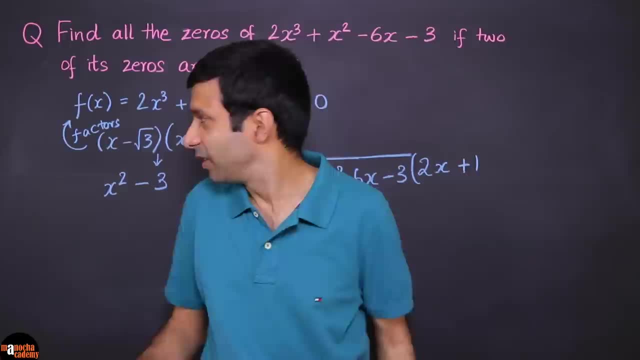 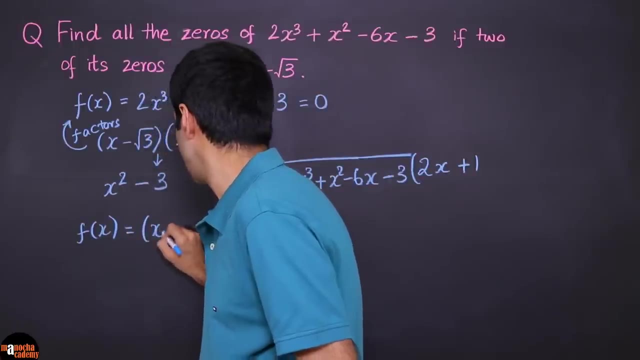 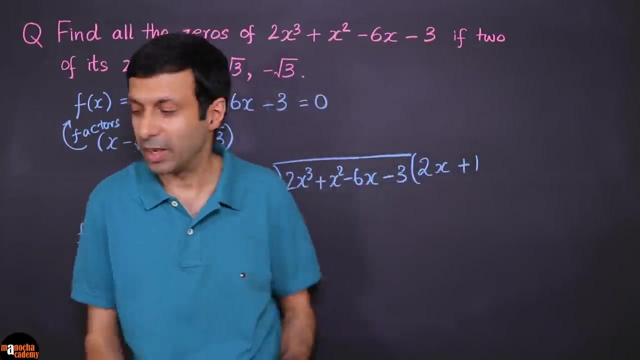 So we've got the quotient as 2x plus 1.. This means We can write this polynomial fx as: fx equals x square Minus 3. Multiplied by our quotient here, Which is 2x plus 1.. 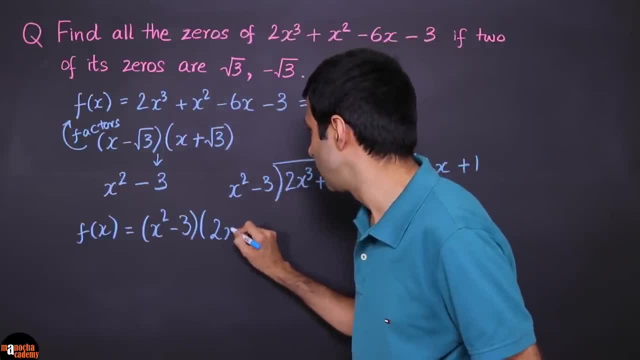 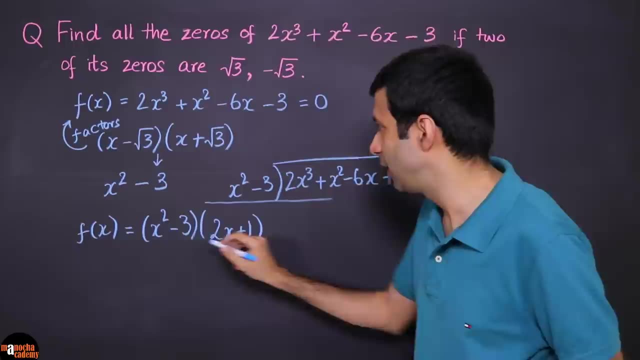 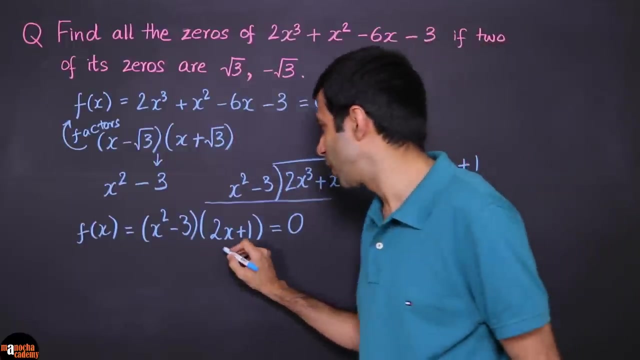 Right. So we're going to Multiply this Right, And this is equal to 0.. I'm just going to draw a line here, Right, To separate these, And this is equal to 0.. Right, Which means that this factor. 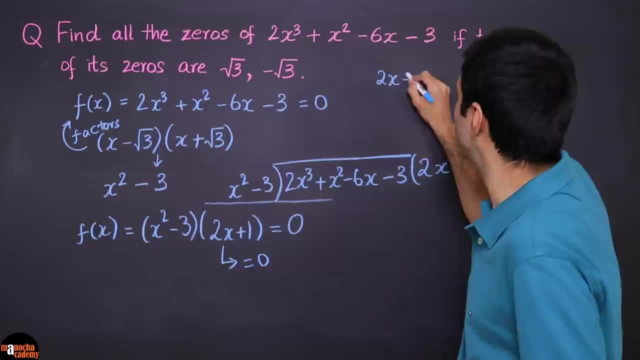 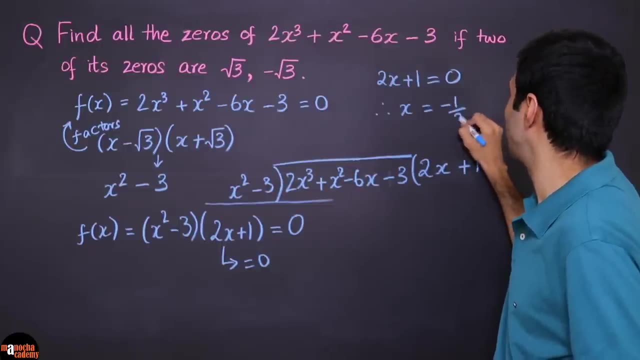 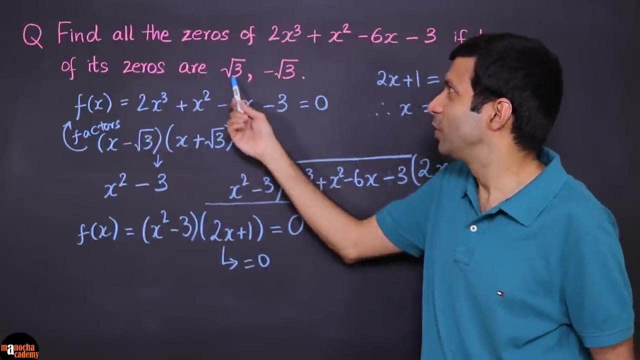 2x plus 1. Is equal to 0. So we can say, Therefore, x equal to Minus half Right. So that's the other zero of this Polynomial Right. So using these two We found the. 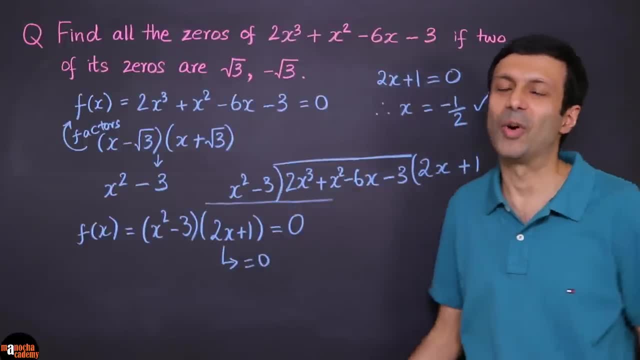 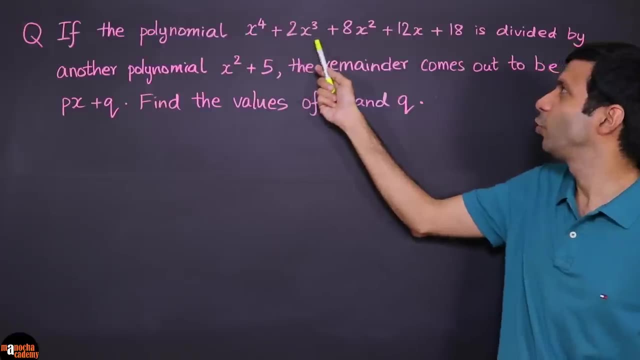 x square minus 3.. And we divided it by that And we easily got the other zero Of this polynomial Ready for our next question. If the polynomial 8x square plus 12x plus 18. Is divided by: 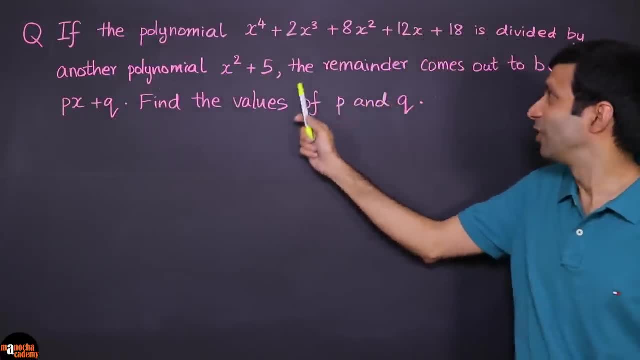 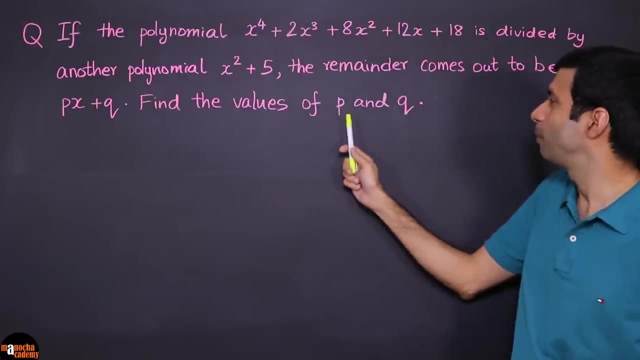 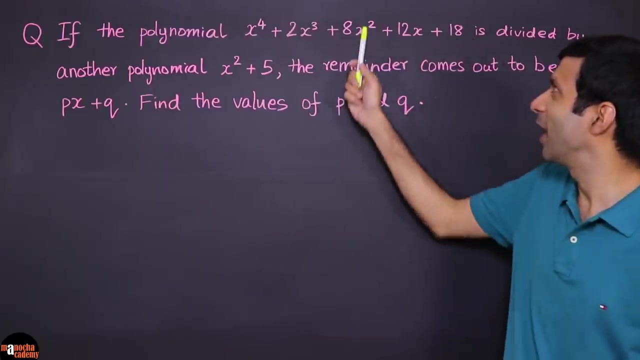 Another polynomial, x, square plus 5.. The remainder comes out to be Of the form: px plus q. Find the values Of p and q. So how do you solve this question? It's pretty simple: You just need to divide. 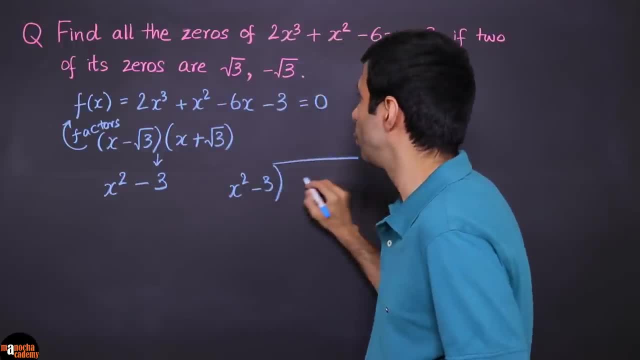 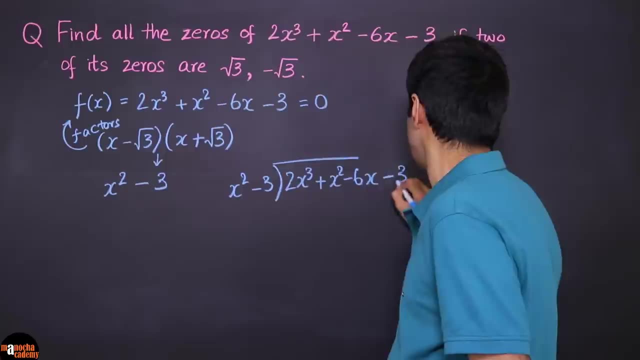 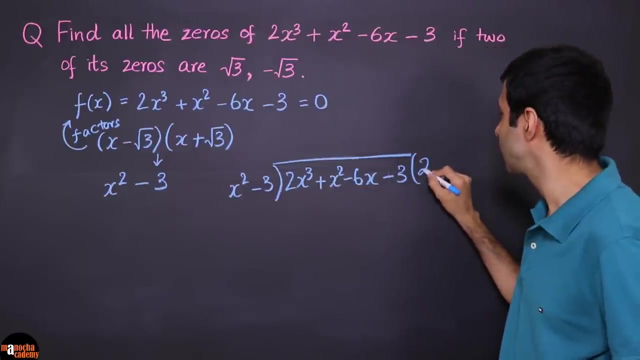 So x squared minus 3,. if we sit and do this division, so 2x cubed plus x squared minus 6x minus 3, right? So if you sit and divide this and you solve this, you're going to get the quotient as 2x plus 1, okay. 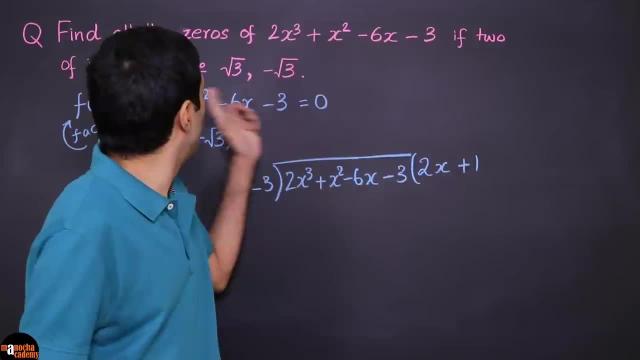 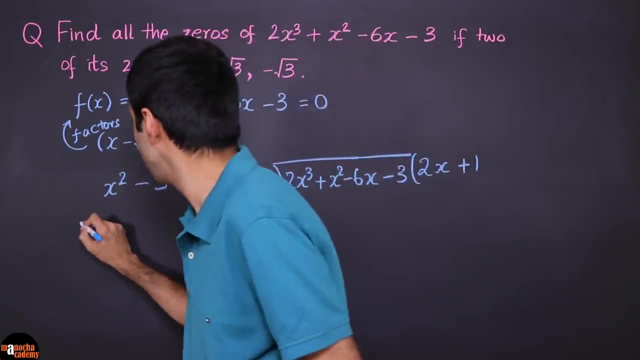 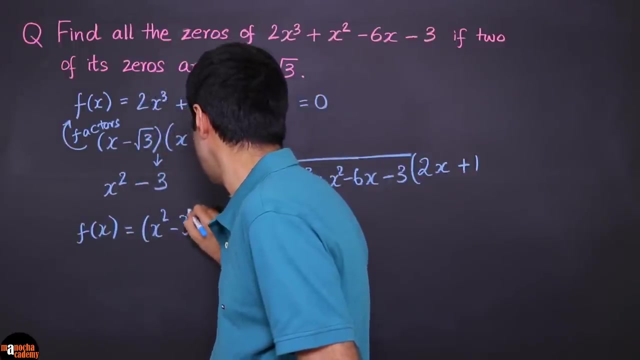 So now, how can we find the other 0?? So we've got the quotient as 2x plus 1.. This means we can write this polynomial fx as: fx equals x squared minus 3, multiplied by our quotient here, which is 2x plus 1, right? 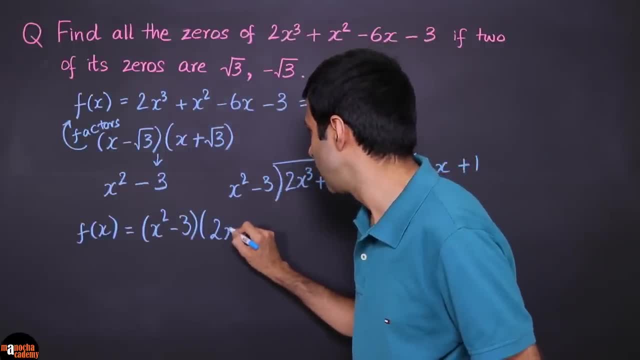 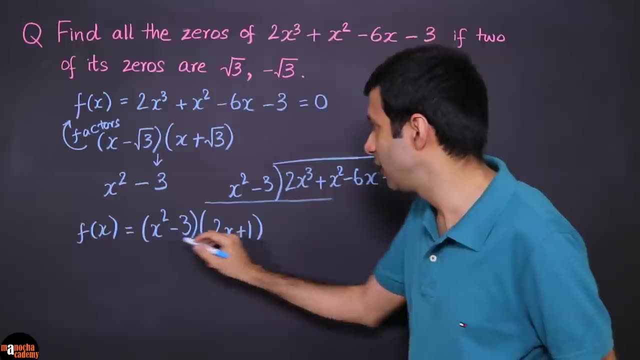 So we're going to multiply this right, And this is equal to 0.. I'm just going to draw a line here right to separate these, And this is equal to 0, right, Which means that this factor 2x plus 1,. 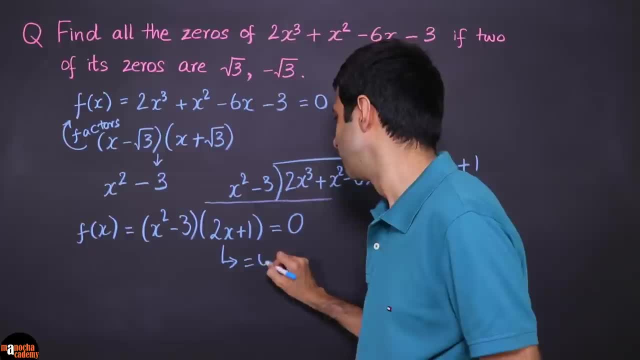 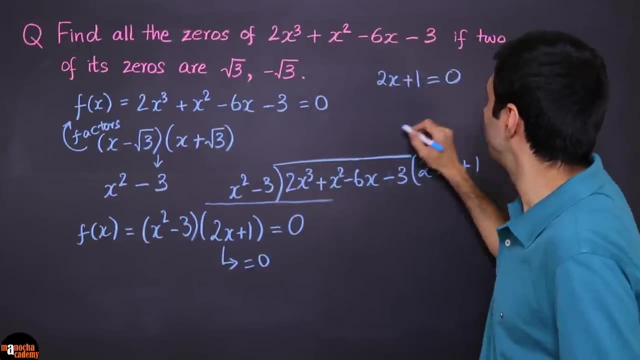 is equal to 0. So we can say, if we have 2x plus 1 equal to 0, we can write that down here: 2x plus 1 is 0. Therefore, x equal to minus half right. 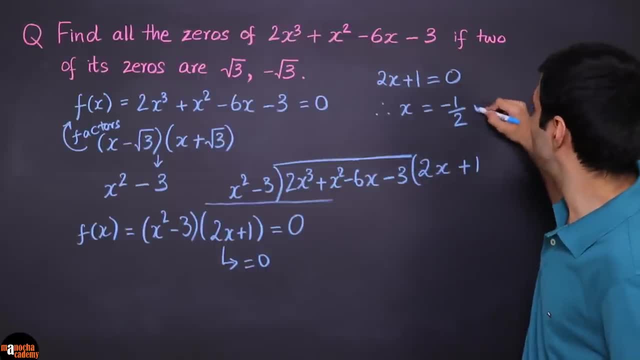 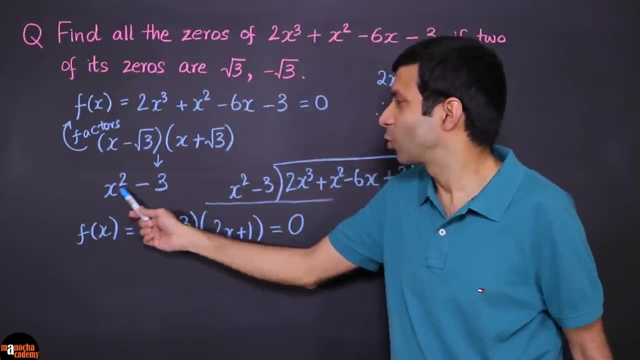 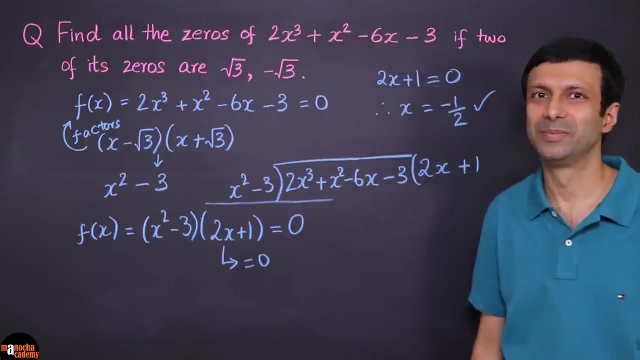 So that's the other 0 of this polynomial right. So using these two, we found the x squared minus 3, and we divided it by that and we easily got the other 0 of this polynomial Ready for our next question. 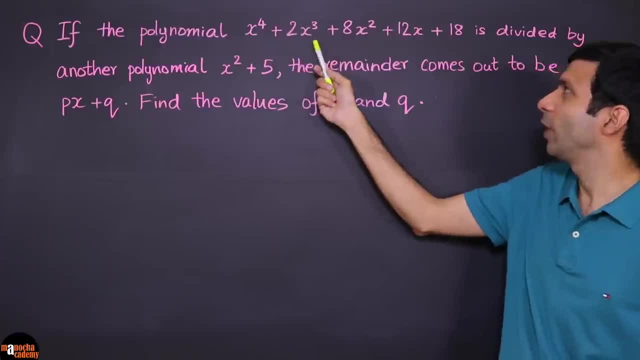 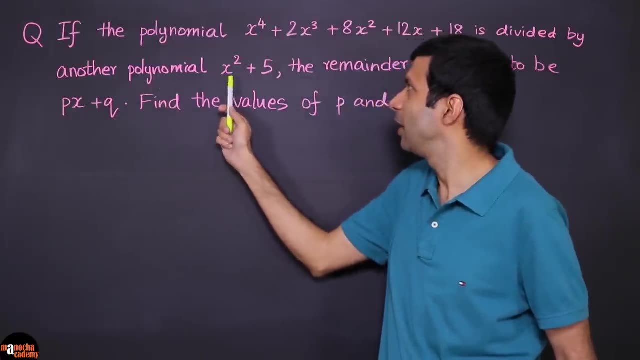 If the polynomial x to the power 4 plus 2x cubed plus 8x squared plus 12x plus 18, is divided by another polynomial x squared plus 5, the remainder comes out to be of the form px plus q. 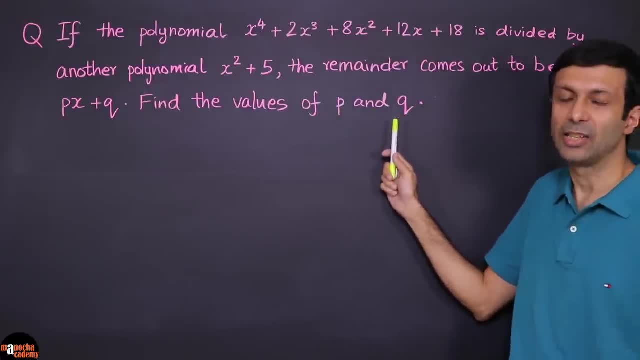 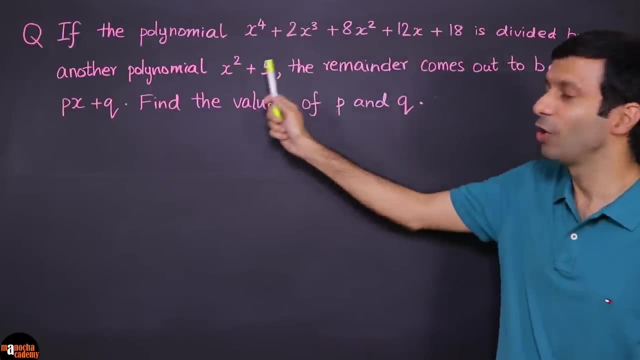 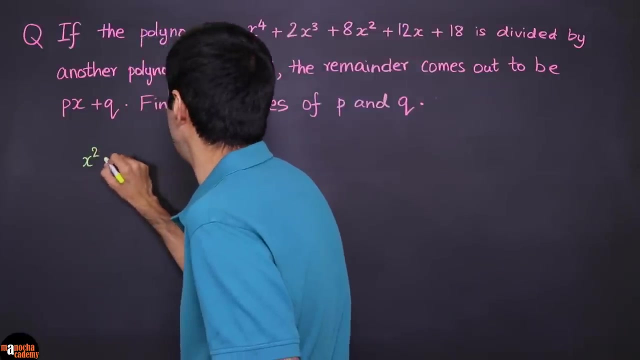 Find the values of p and q. So how do you solve this question? It's pretty simple: You just need to divide this polynomial with this one. So let's write it down. So this is going to be our divisor: right x squared plus 5,. 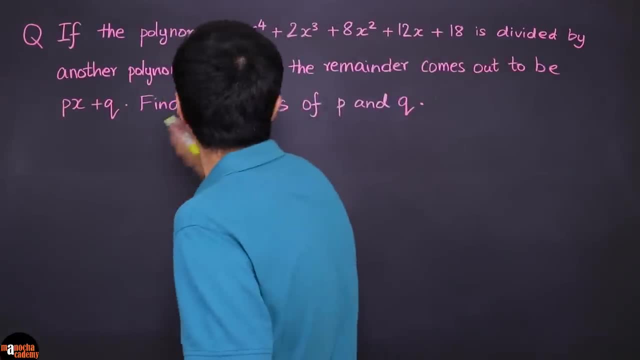 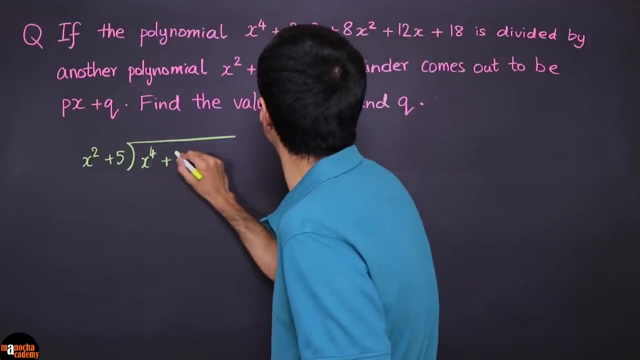 This polynomial with this one. So let's write it down. So this is going to be our divisor, Right Plus 5.. And we need to divide This long polynomial x to the power 4.. So just write it down. 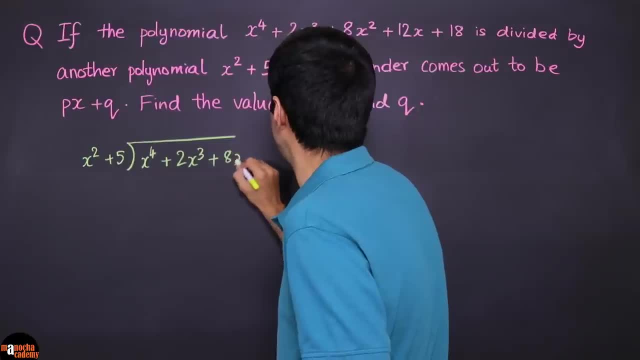 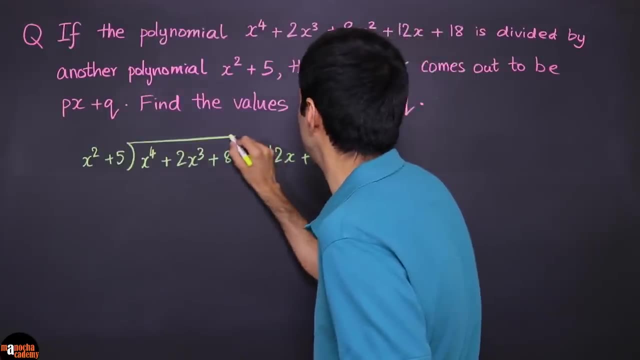 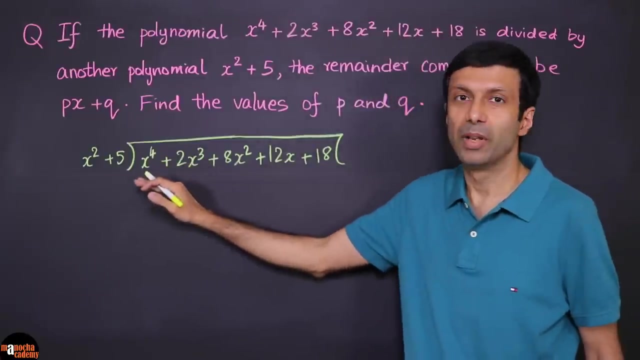 Plus 2x cube, Plus 8x square, Plus 12x Plus 18.. And so Let me extend this line Right up to here, Okay, And so you need to sit and do this division, Right, And I'm not going to do it here. 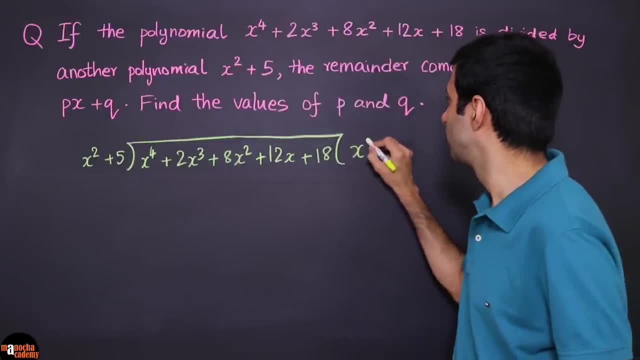 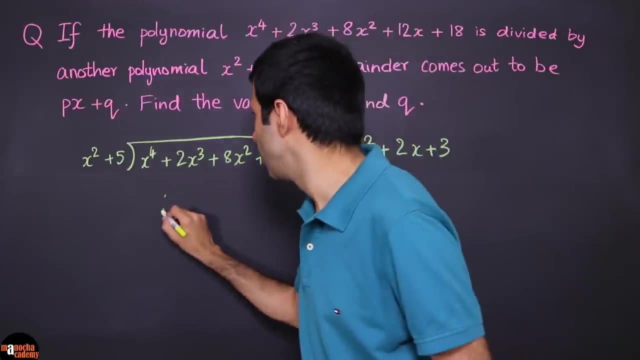 So I'll write down what's the quotient going to turn out to be x square Plus 2x Plus 3.. So that comes out to be the quotient, And when you divide this, We'll get the remainder as 2x plus 3.. 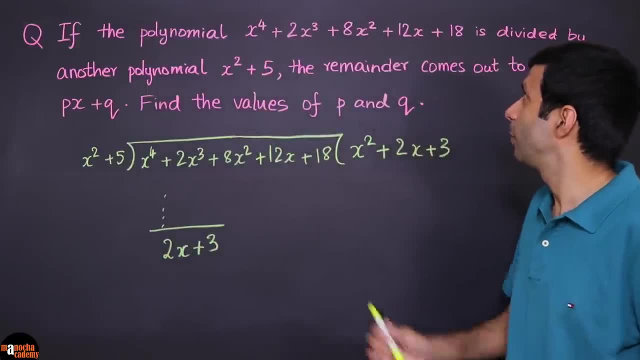 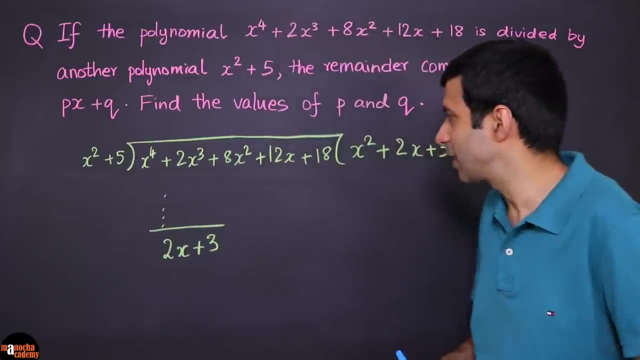 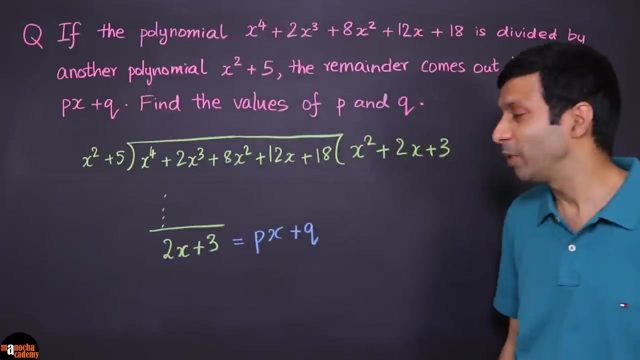 Okay, And note that the question talks only about the Remainder, not the quotient, So take care to compare Just the remainder with the form px plus q Basically is going to be px plus q. Now it's pretty simple. 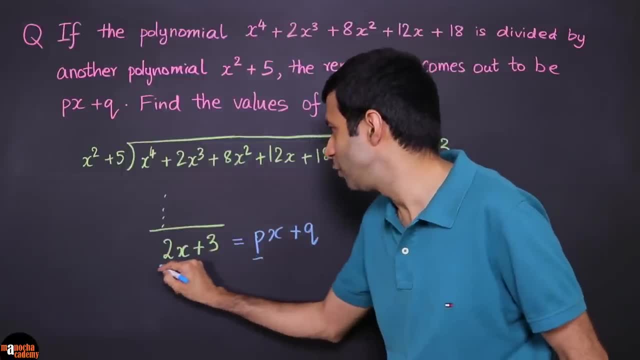 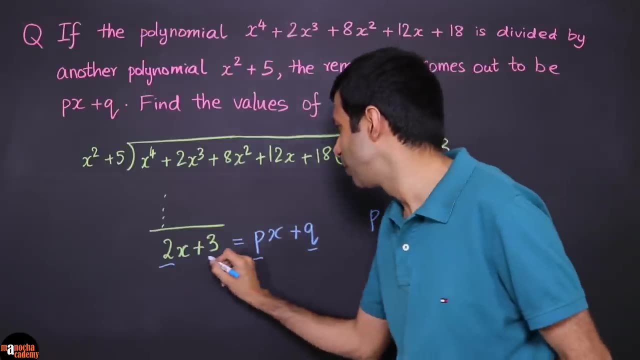 You just need to compare the coefficients. So p is going to be 2.. Right, Just comparing the remainder with this form. So we have p as 2.. And what will q be? Very simple, q is going to be 3.. 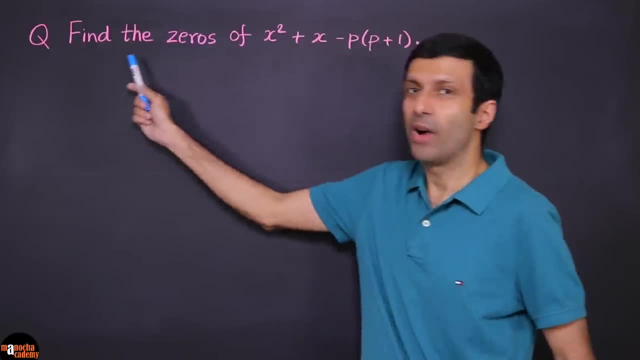 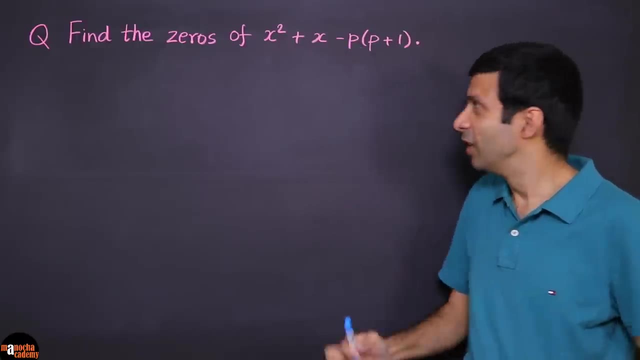 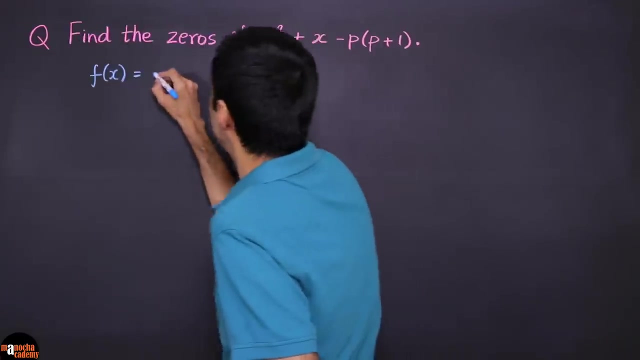 Okay, So that's our answer here. Let's look at our next question. Okay, So let's write down our polynomial. So our polynomial fx Is x square Plus x Minus p into p plus 1.. Right, 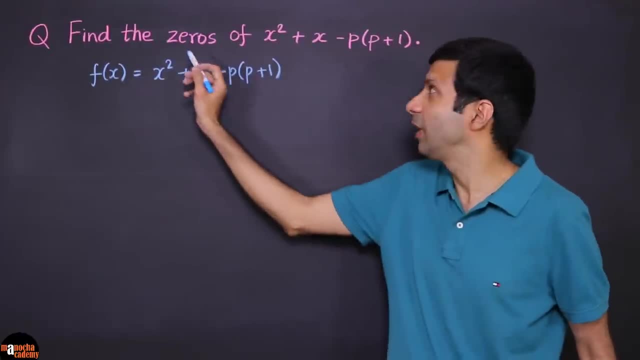 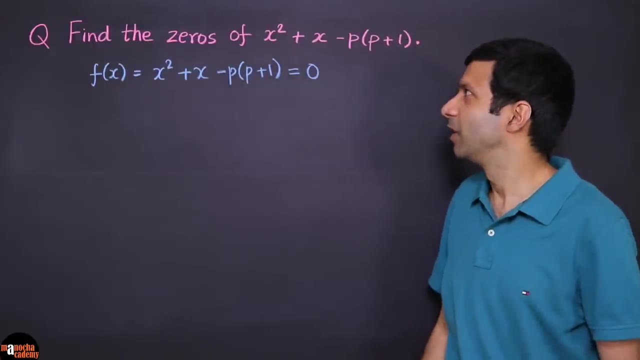 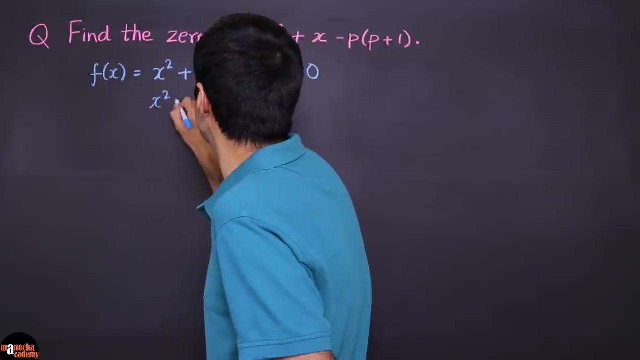 Okay, And remember, to find the zeros of the polynomial, We need to Equate this polynomial to 0.. So that's our equation And we need to solve for x here. Okay, So it's pretty simple, And first let's expand it out here. 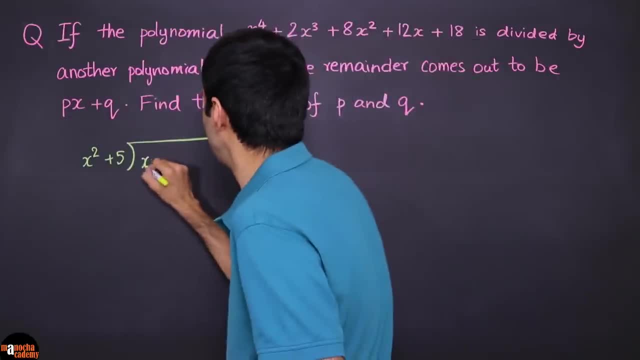 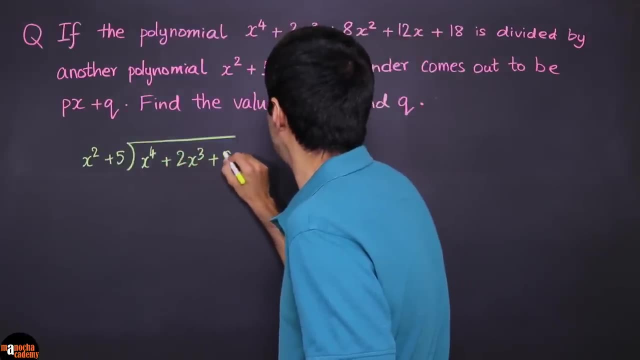 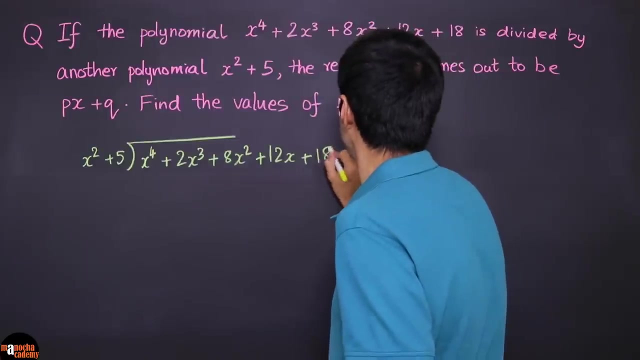 and we need to divide this long polynomial x to the power 4, so just write it down: plus 2x cubed, plus 8x squared, plus 12x plus 18.. And so let me extend this line right up to here, okay. 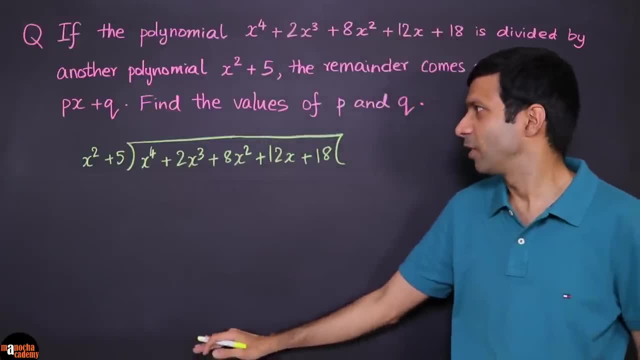 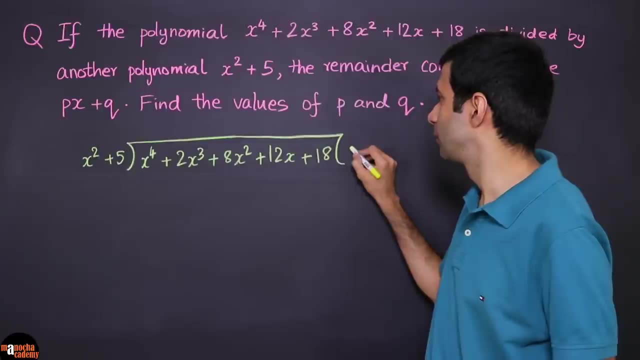 And so you need to sit and do this division right. It's simple algebra, so you need to divide it, So I'm not going to do it here, So I'll write down what's the quotient going to turn out to be. 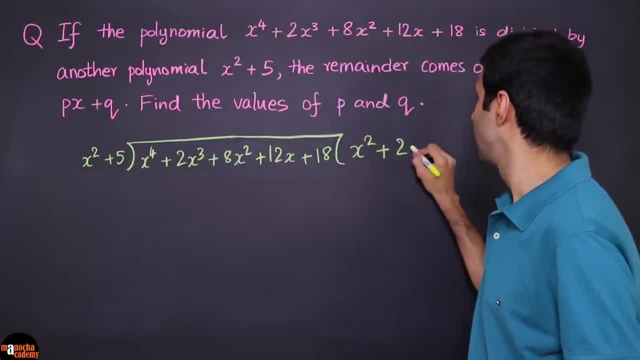 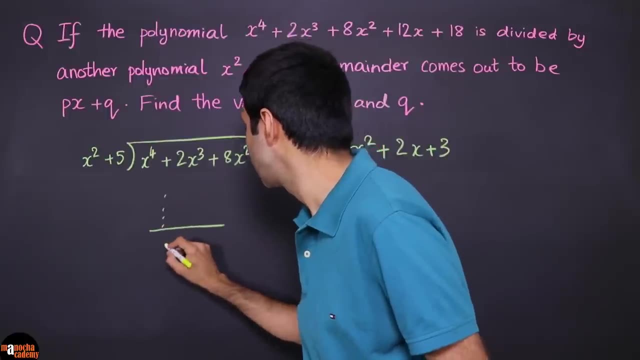 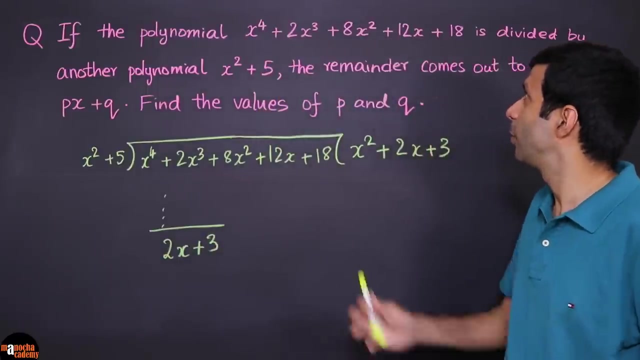 x squared plus 2x plus 3.. So that comes out to be the quotient and when you divide this, we'll get the remainder as 2x plus 3, okay, And note that the question talks only about the remainder. 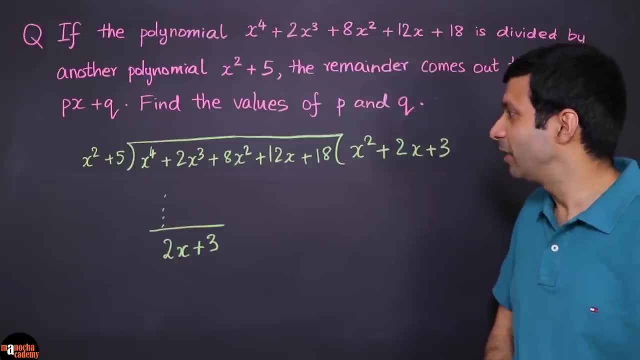 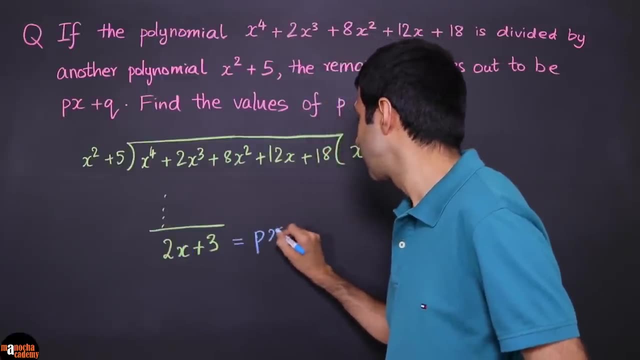 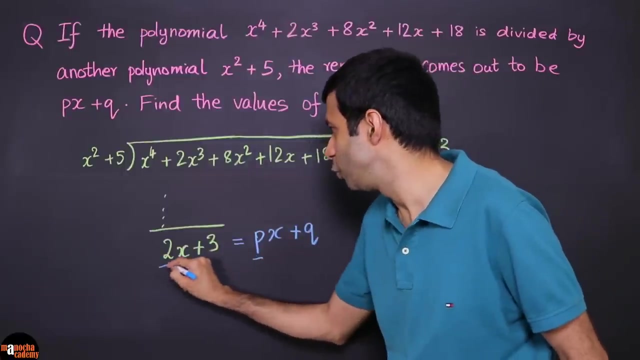 not the quotient. So take care to compare just the remainder with the form px plus q. So this, basically, is going to be px plus q. Now it's pretty simple. You just need to compare the coefficients. So p is going to be 2, right. 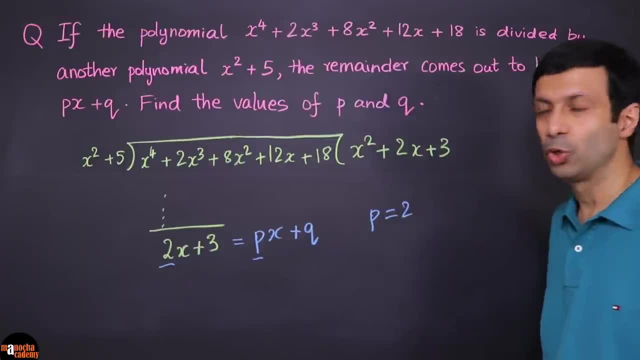 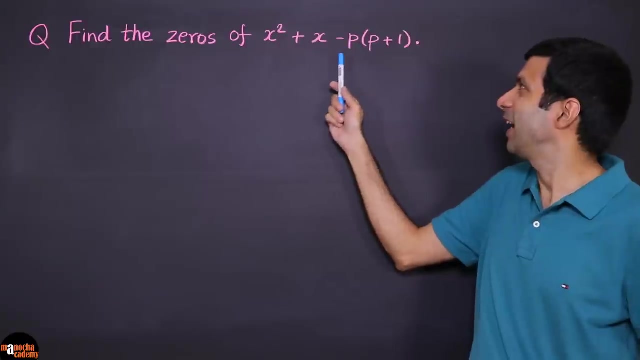 Just comparing the remainder with this form. So we have p as 2, and what will q be? Very simple, q is going to be 3.. Okay, So that's our answer here. Let's look at our next question. Find the zeros of x squared plus x minus p into p plus 1.. 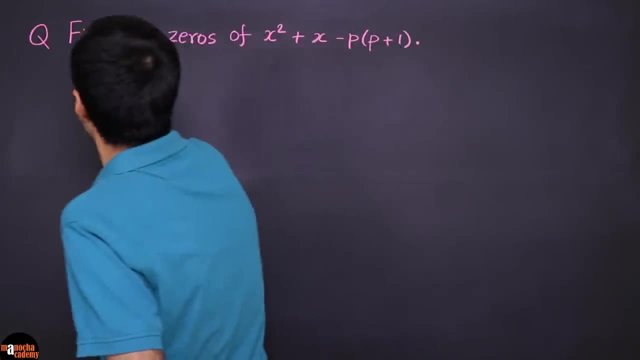 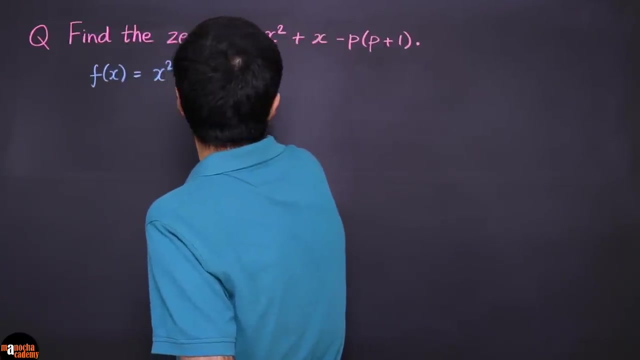 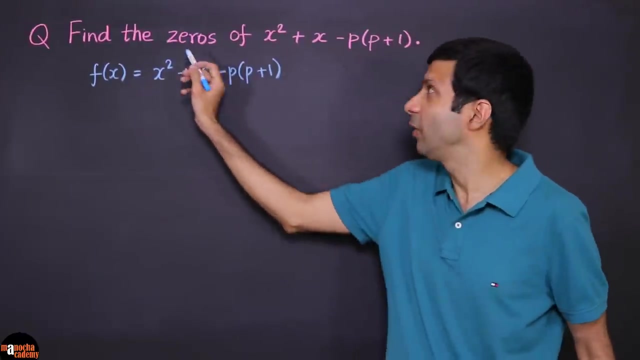 Okay, So let's write down our polynomial. So our polynomial f is x squared plus x minus p, into p plus 1.. Okay, And remember, to find the zeros of the polynomial, we need to equate this polynomial to 0.. So that's our equation. 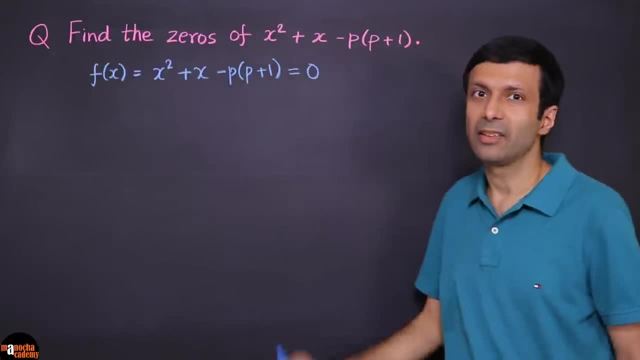 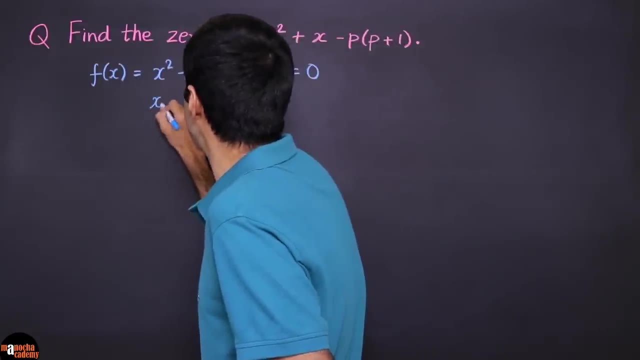 And we need to solve for x here. Okay, So it's pretty simple, And first let's expand it out here. So x squared plus x, and let's expand out these terms, So we are going to get minus p squared minus p equal to. 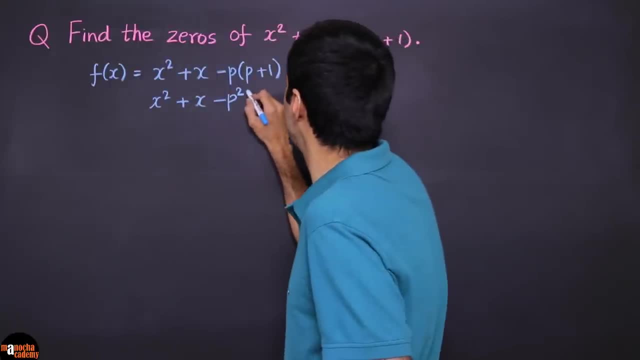 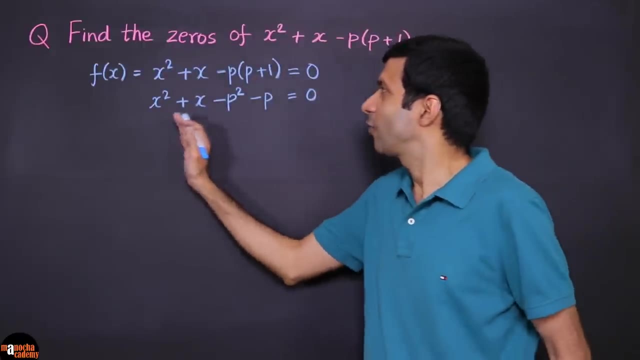 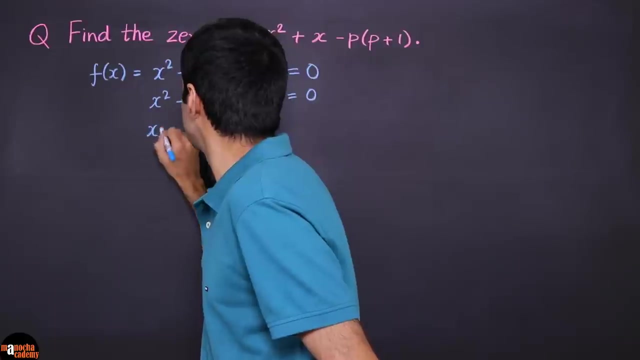 So x square plus x, And let's expand out these terms, So we are going to get minus p square, Minus p equal to 0.. Right, So now we need to factorize this To find the zeros Of this polynomial. 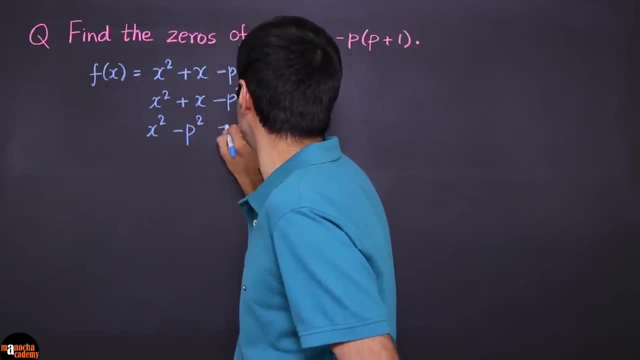 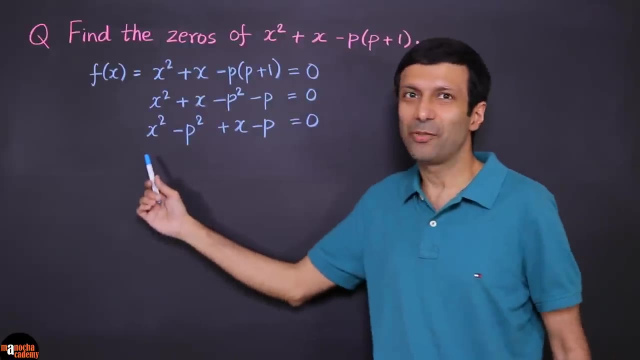 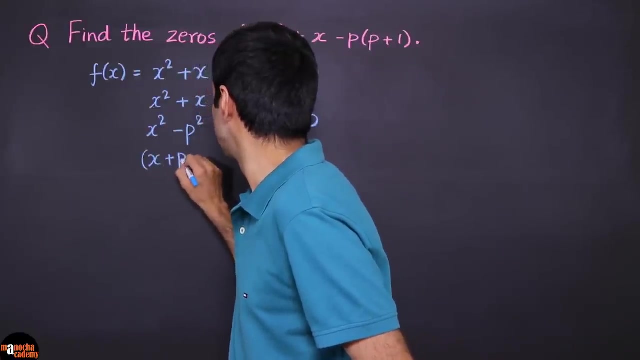 So let's take the square terms together, So it's x square Plus x minus p. So we are doing this to Factorize it, Okay, And can you see that form A square minus b square, Right? So let's write that as: 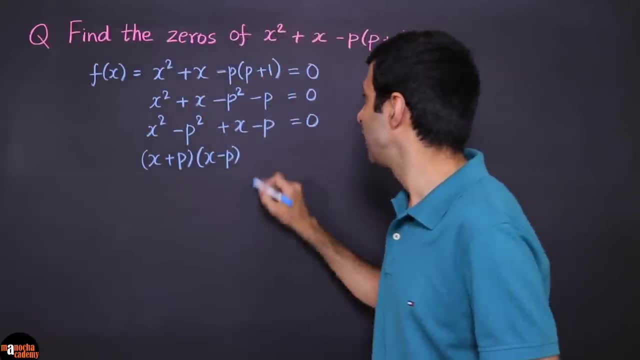 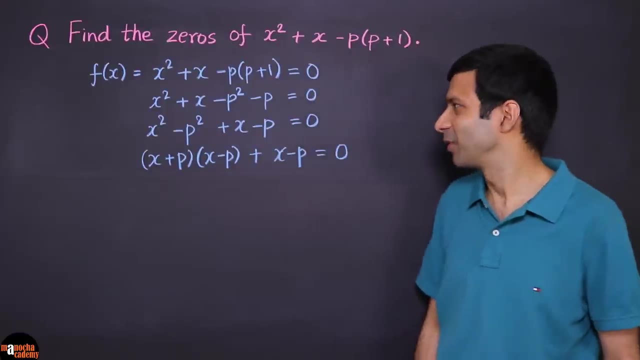 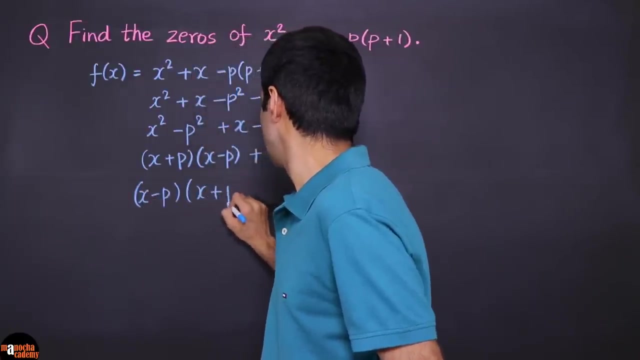 x plus p Into x minus p, Right? So that's that. And then we have Plus x minus p Equal to 0. So what are we going to get? Into x plus p Plus 1.. Okay, Right. 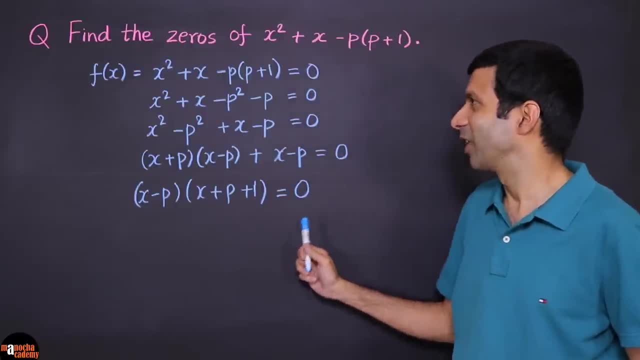 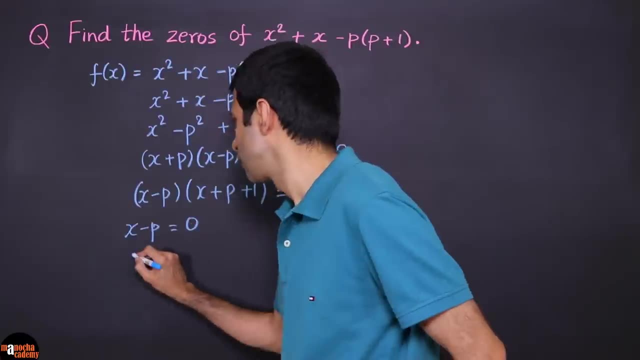 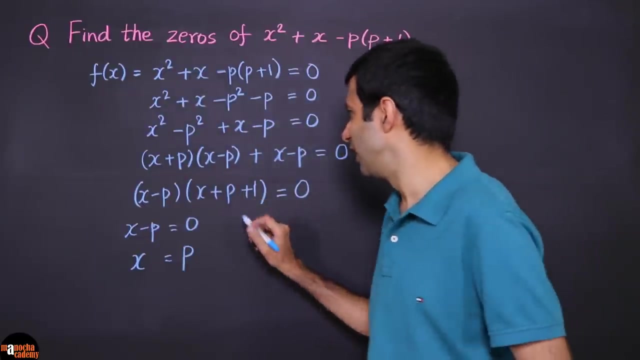 So either this is 0. Or this is 0.. Right, So those are our zeros of x, So we can have. So what do we have here? So x minus p is 0. So that's x equal to p, right. 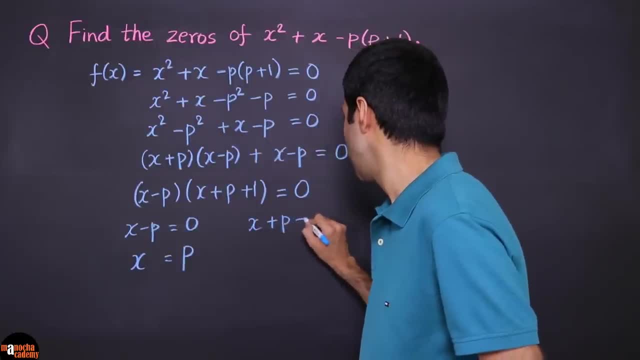 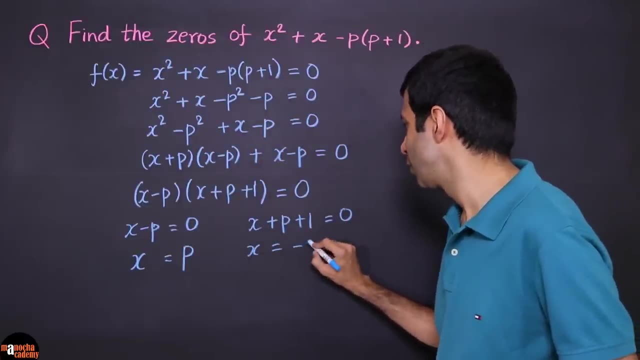 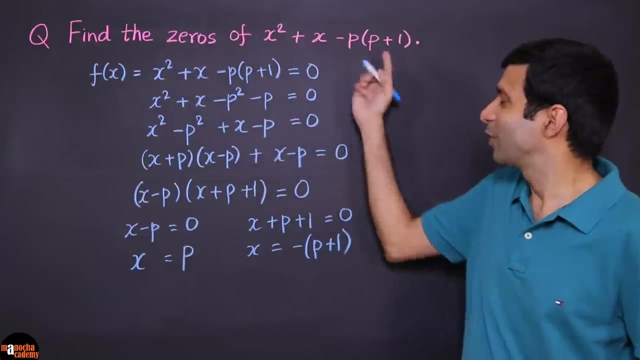 That's one of our zeros. So x plus p plus 1. Equals 0. Which basically means x equal to Minus of p plus 1. right, It goes to the other side. So here we found The two zeros of this polynomial. 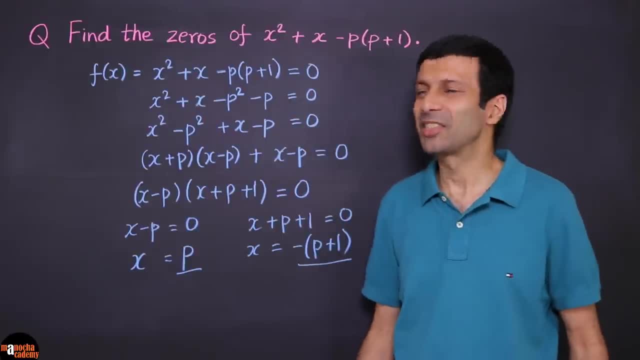 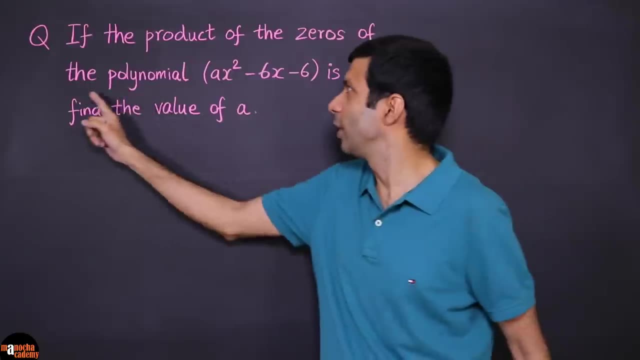 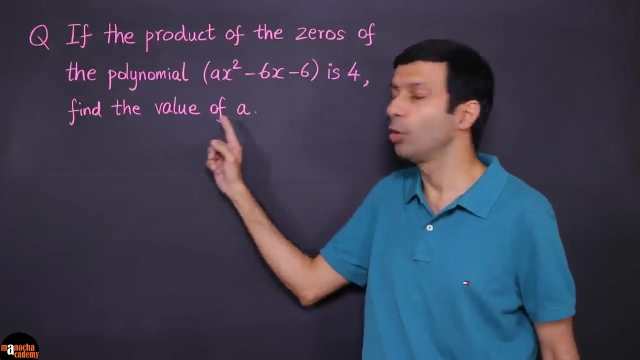 It's p And minus p plus 1.. That's our answer of this question. And here's our final question. If the product of the zeros Of the polynomial Is x squared Minus 6x, Minus 6.. 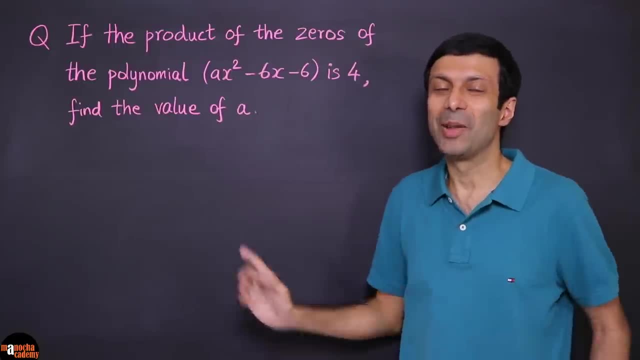 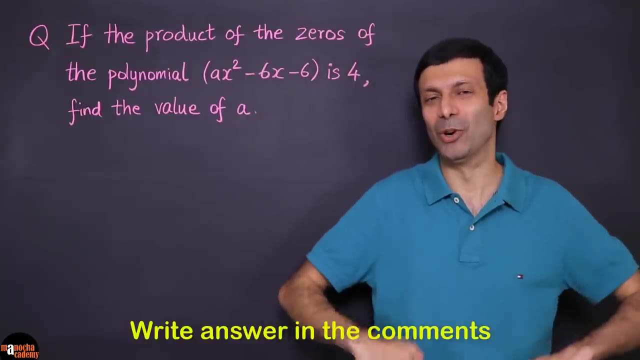 Is 4. Find the value of a. Now I'm not going to be solving this question, Because I want you to try it yourself And do let me know your answer By putting it in the comments below. I look forward To reading your answers. 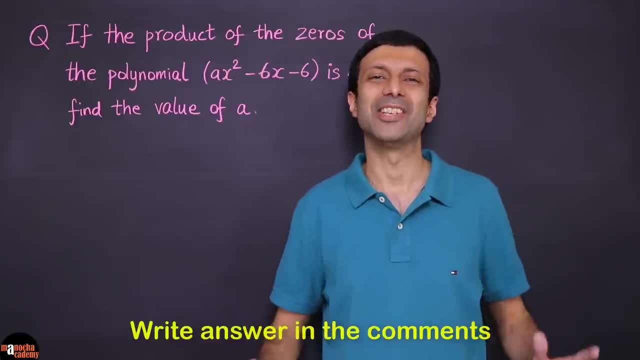 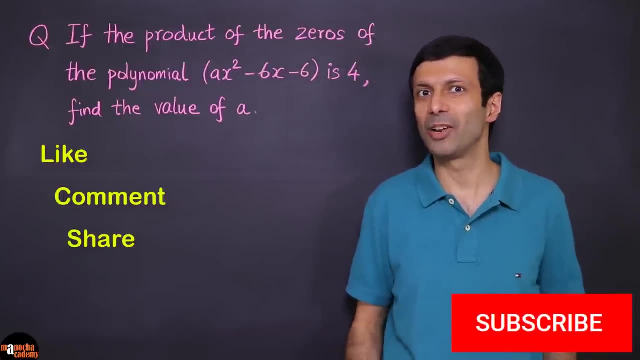 So I hope the concept of polynomials Is crystal clear to you now, And do remember To like: And if you haven't subscribed To my YouTube channel already, Hit the subscribe button Right now And do click the notification bell. 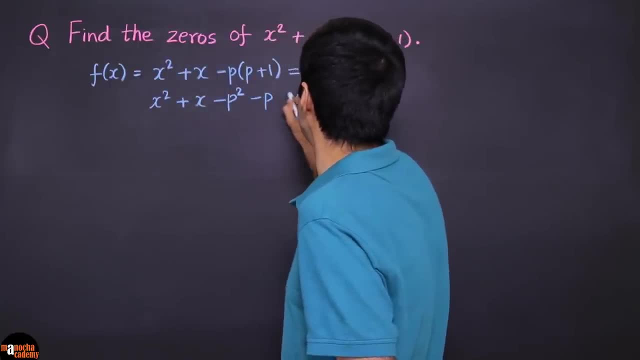 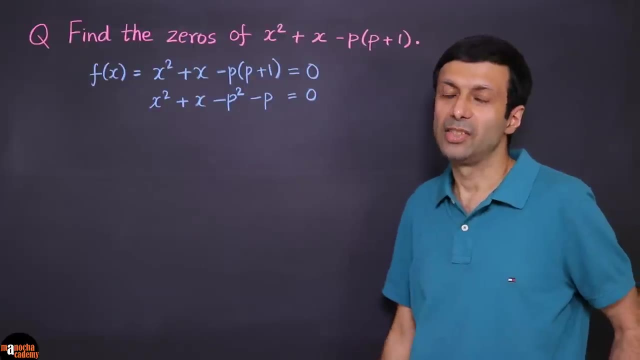 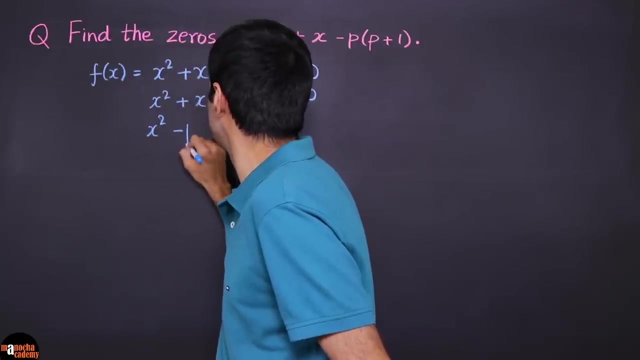 p squared plus x minus p. Okay, So that's going to be 0.. Right, So now we need to factorize this to find the zeros of this polynomial. So let's take the square terms together. So it's x squared minus p, squared plus x minus p. 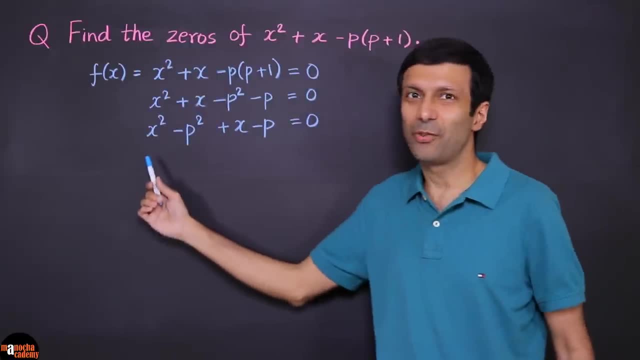 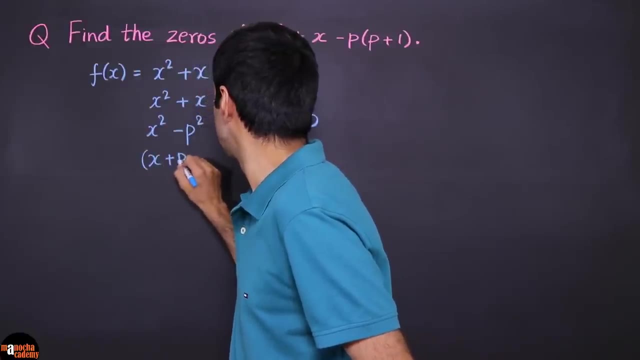 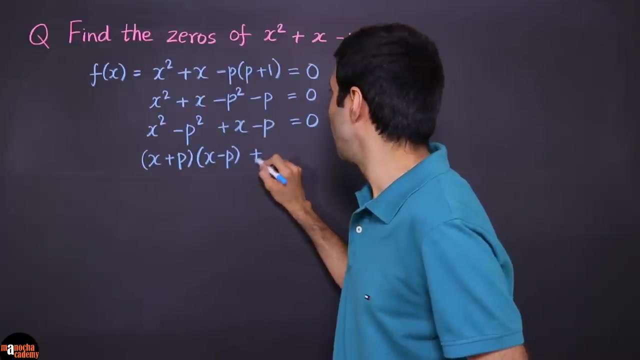 So we are doing this to factorize it, Okay, And can you see that form a squared minus b, squared Right. So let's write that as x plus p into x minus p, Right? So that's that, And then we have. 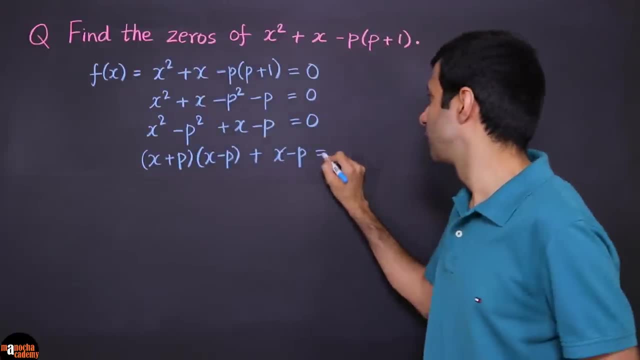 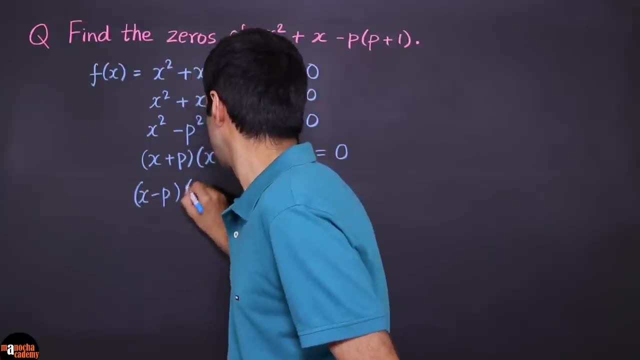 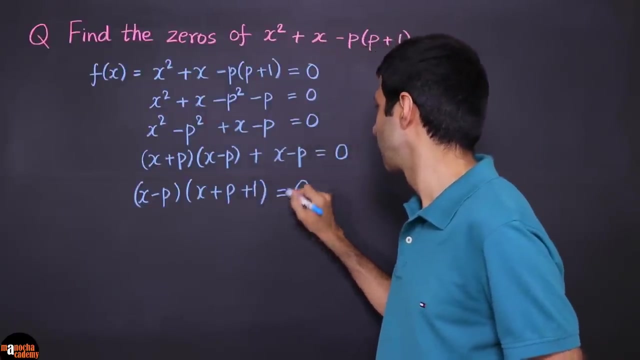 plus x minus p equal to 0.. Right, So let's take x minus p common here. So what are we going to get Into x plus p plus 1.. Okay, Right, So either this is 0 or this is 0. 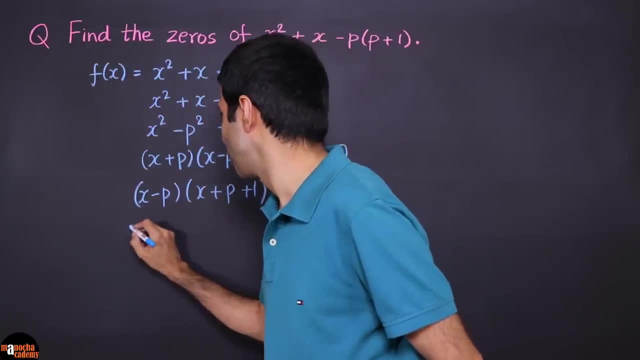 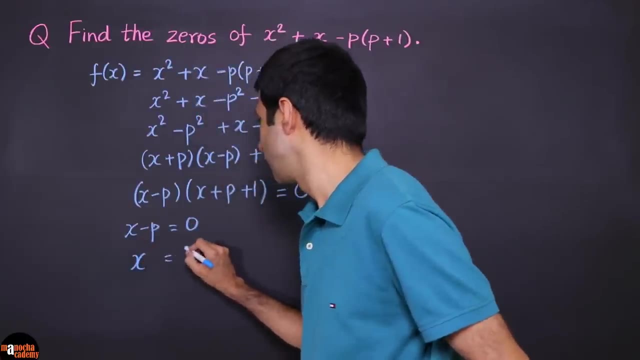 Right, Those are our zeros of x, So we can have. So what do we have here? So x minus p is 0.. So that's x equal to p. Right, That's one of our zeros, And let's also equate this to 0.. 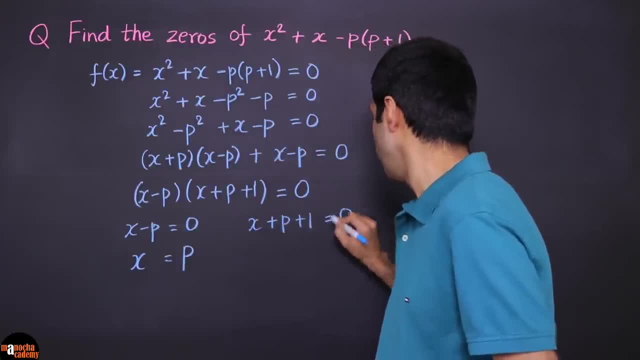 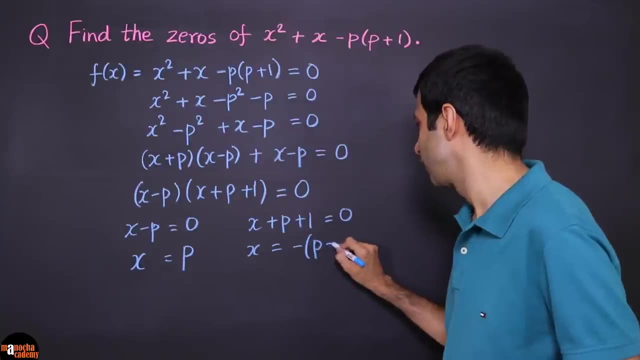 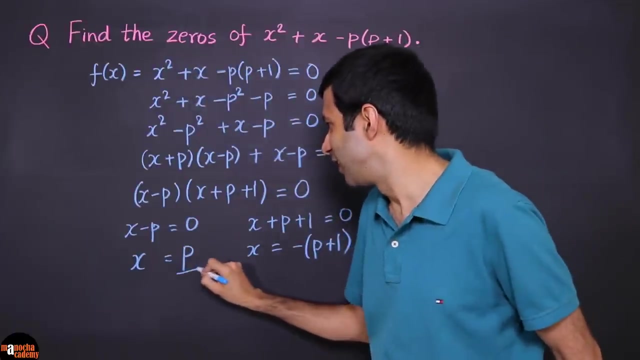 So x plus p plus 1 equals 0. Which basically means x equal to minus of p plus 1.. Right, It goes to the other side. So here we found the two zeros of this polynomial: It's p and minus p plus 1.. 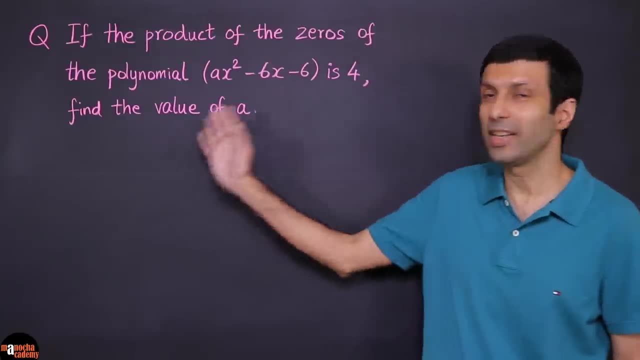 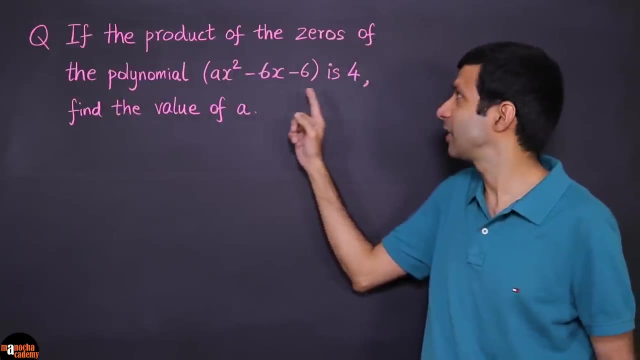 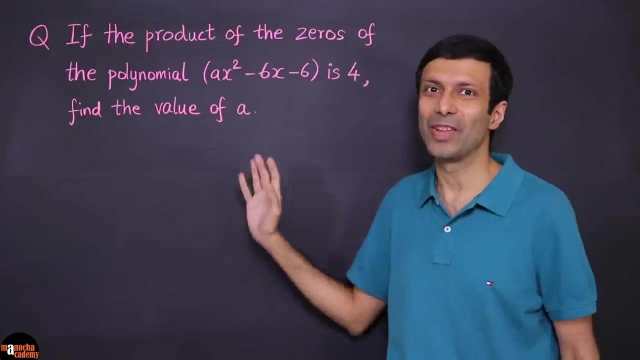 That's our answer of this question. And here's our final question. If the product of the zeros of the polynomial ax square minus 6x minus 6, is 4,, find the value of a. Now I'm not going to be solving this question. 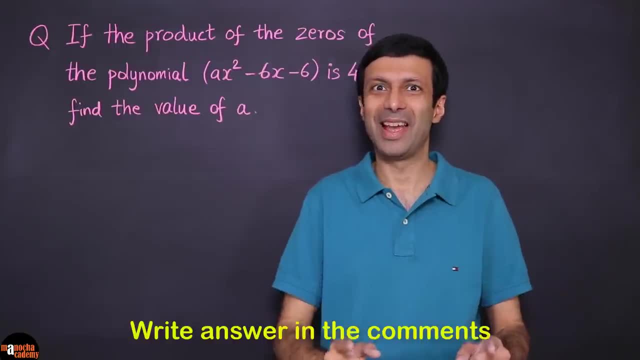 because I want you to try it yourself And do let me know your answer by putting it in the comments below. I look forward to reading your answers, So I hope the concept of polynomials is crystal clear to you now, And do remember to like, comment and share out this video.